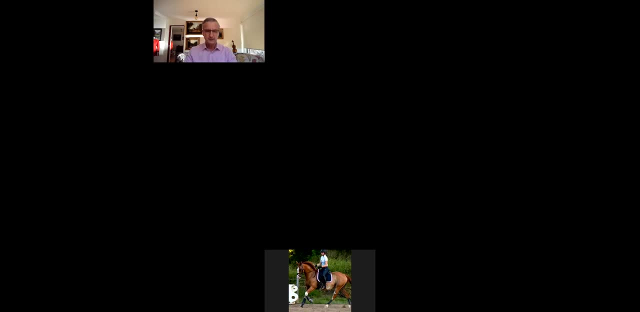 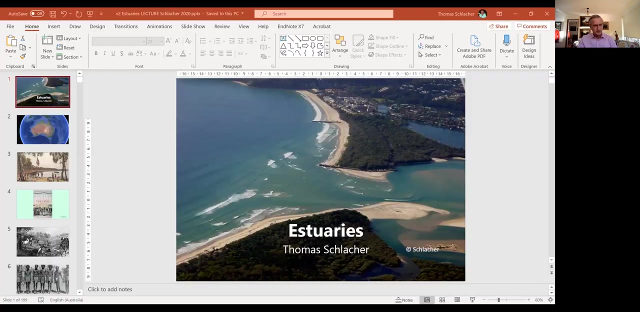 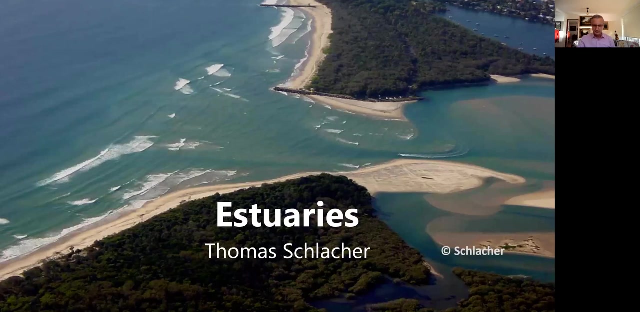 So today, our lecture is probably going to be, you know, an hour and a half or something like this. There's a lot of content to go through, but it's an interesting one because, come on, we're going to talk about environments which are, by most likelihood, going to be your. 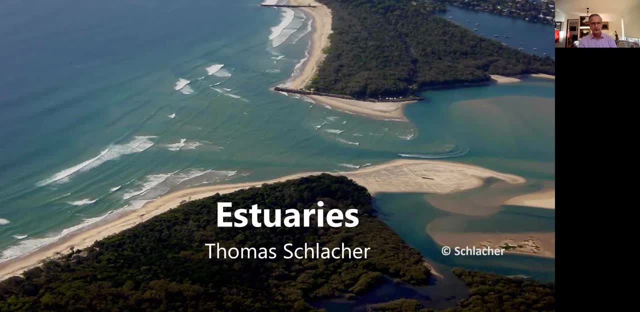 bread and butter. as a marine ecologist, a coastal ecologist or you know, whatever profession you're going to take, It is basically those very environments we're going to talk about today, in the next lecture, which are the centers, really, of our activity as a human race, so to speak, in a 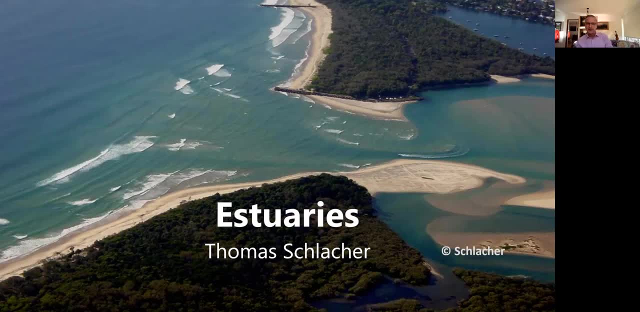 coastal zone. I mean, you do know that about. okay, let's have a guess. what is the percentage in Australia of people living within 50 kilometer of the coast? Give me, give me a number. Isn't it something like 90 percent? Good lord, it's 89.. 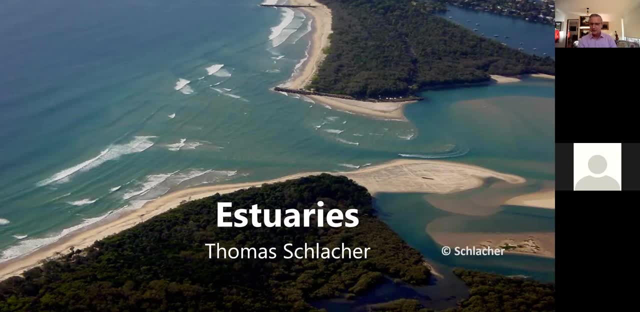 So 90 percent is is very, very good. So you know, we, we kind of when you, when you're overseas, you actually think you know, in terms of the advertisements for Australia, oh, it's the red same thing. there's kangaroos jumping around, it's permanently hot and that kind of stuff. you know. 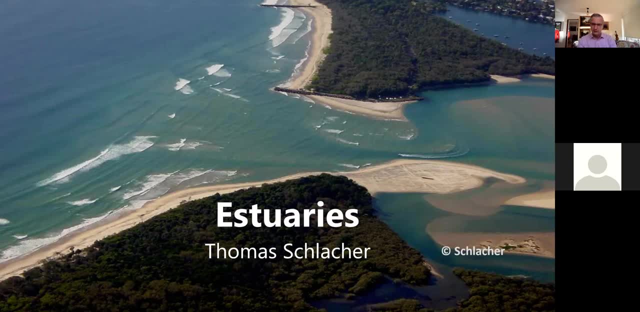 But essentially, in a world ranking, we are number 10 in in terms of the most urbanized societies, because 50 percent of all our populations live within five kilometers of a city center, 90 percent of our population lives within 50 kilometres on the coast and 90 percent of those people live within 80 kilometers of a capital city. So essentially, 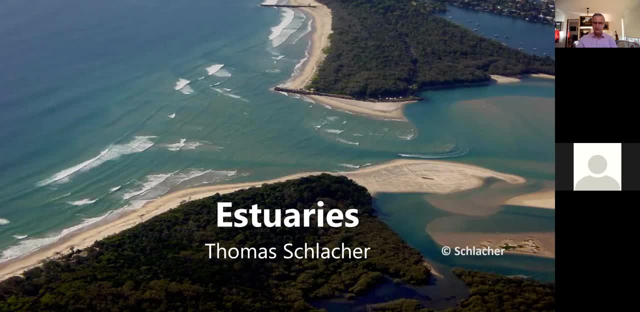 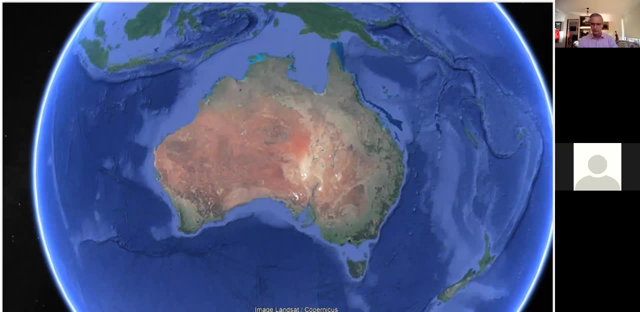 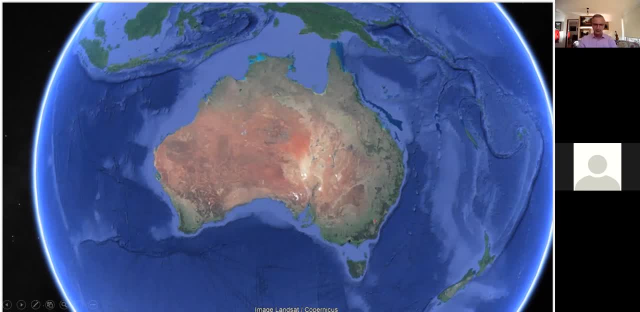 What I really want to know is about the big blue sea out here. Well, you know, that's, of course, very, very exciting to study, But in reality, as a human society, we are intensely coastal, But we don't actually pick every part of the coast in equal measures. 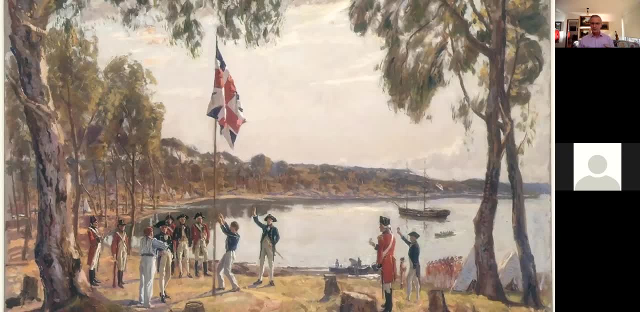 We actually pick bits and pieces which are sheltered, which are easy to anchor aboard and which actually protect us from the elements and also, you know, conveniently carry our sewage away, And there's no better example in Australia than this kind of painting here. 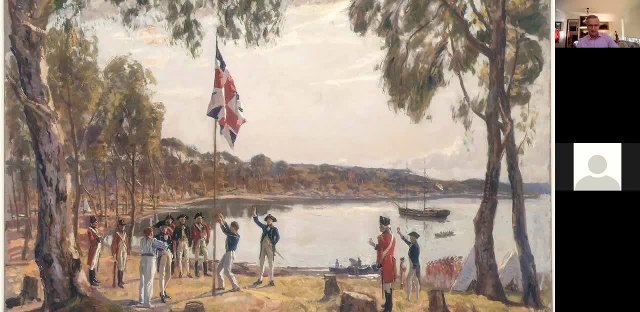 This is, of course, you know, Captain Cook, you know- landing in Botany Bay. Now, Botany Bay looks rather, very different today. This is more or less where you land in a plane. It's in Sydney International Airport. 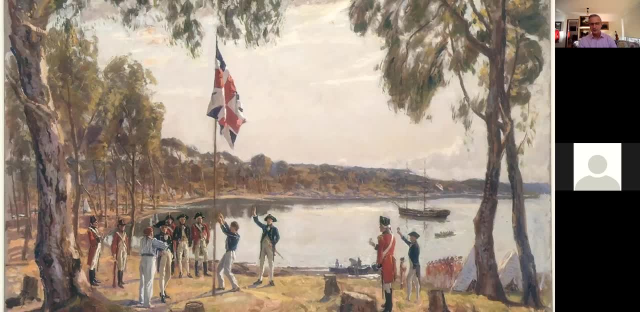 Now I just chucked a couple more slides in there because it is rather interesting. If anybody watched SBS two days ago, they had a short little report or a segment on the 250th anniversary of Captain Cook's landing. Now I thought this was very interesting because about 20 years ago, 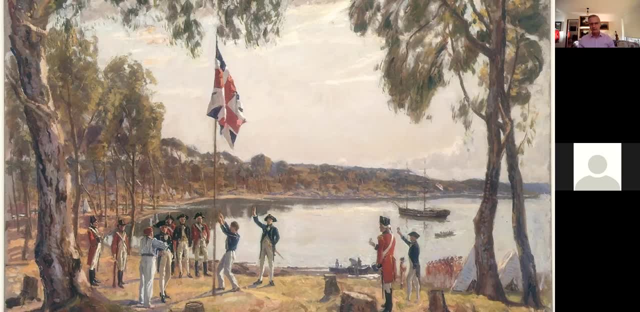 when John Howard was prime minister. it would have been a massive national celebration And you can't really, you know, put it down to. you know the virus. Our views, and quite rightly so, about those colonial events have actually changed quite fundamentally. 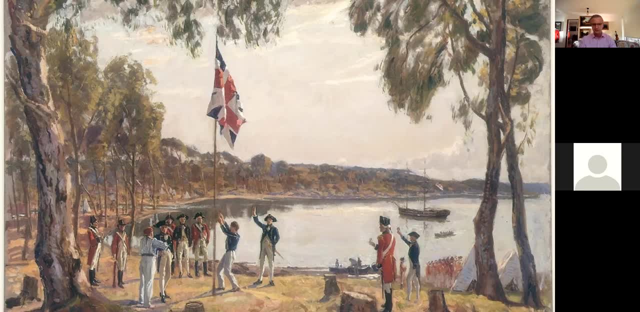 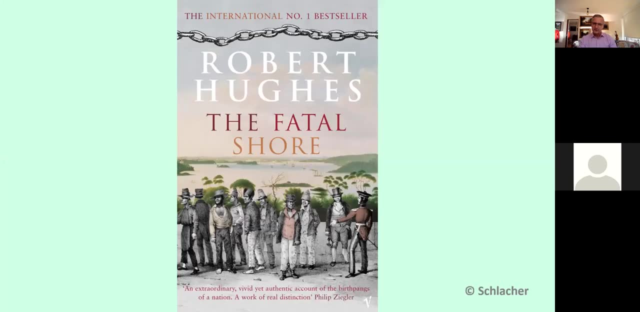 because this is the Anglo-Saxon view of the world, of course. and here is the Union check being, you know, erected on a flagpole. But I very, very much recommend to each of you, you know, to read this book here called Robert Hughes' The Fate of the Shore. 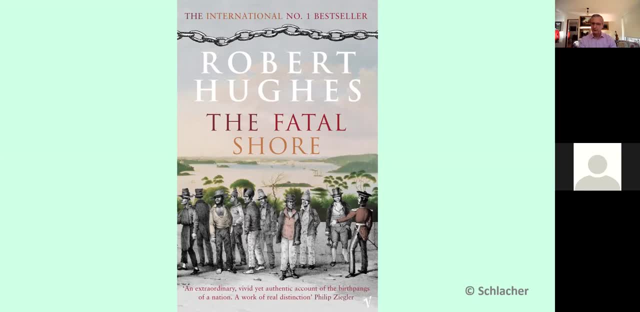 I wouldn't say it gives a, you know, fatalistic view of you know Anglo-Saxon colonial ambitions, but it presents a true one because in the right view of course, our you know historical narrative is that we discovered continents. 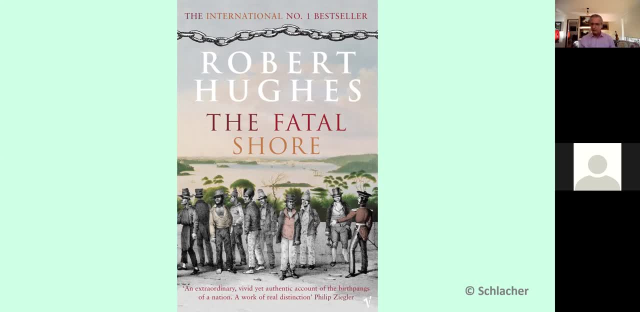 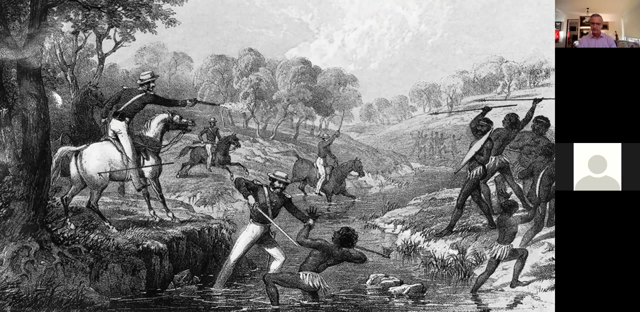 islands, seas and so forth. It was a bit inconvenient that we discovered them and actually somebody already lived there. And, of course, what actually happened in the aftermath of the landing of James Cook were, you know, quite brutal events which haunt basically our nation until this day. 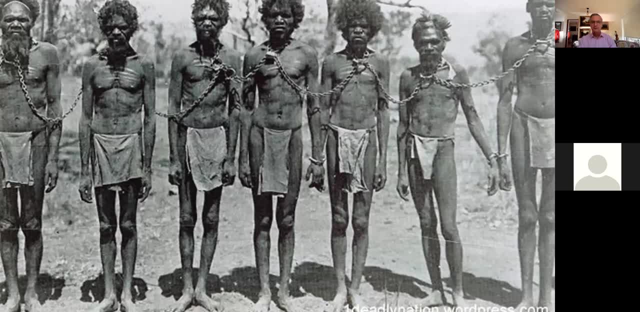 And we shouldn't really forget that, And I thought it was actually very well done and very poignant That Captain Cook's landing is actually seen in a very, very different way nowadays. Now you might say, why do I show you rather confronting pictures of the treatment of the native people of Australia by the white settlers? 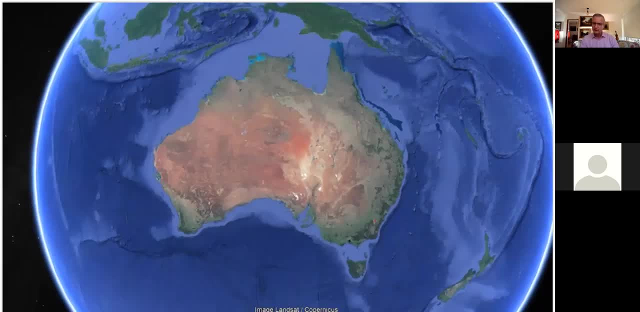 Well, because it is those shallow water bodies which enabled our existence, and still do, on this continent. So let's do a little bit of a geography, Chris. have a look at the Google Earth images I'm going to put up and give me your best guess what place around the Australian coastline it is. 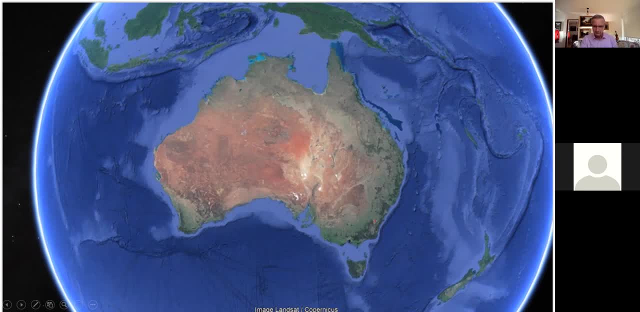 We basically go from here around here. what's that? Adelaide, the Great Australian, Bight and up to Perth. So what kind of place in Australia do you think that is? We got an incredible view. We got an incredible view. We got an incredible view. 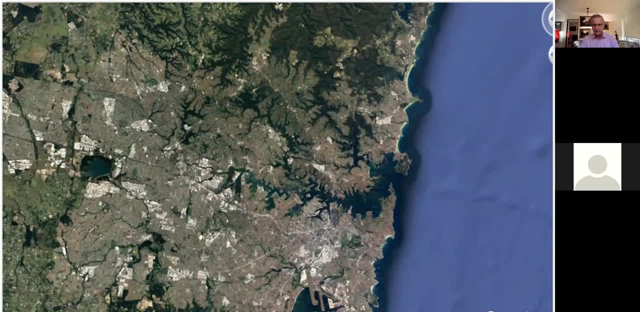 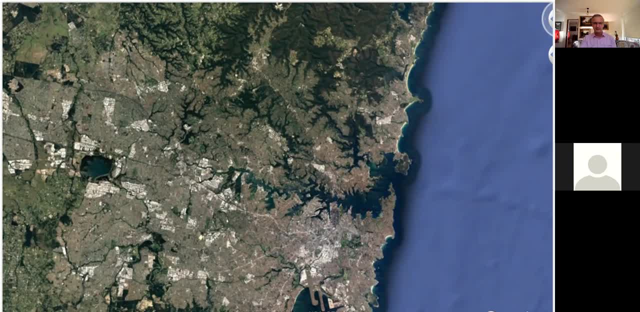 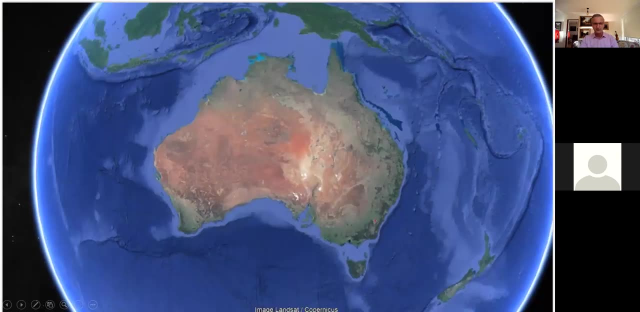 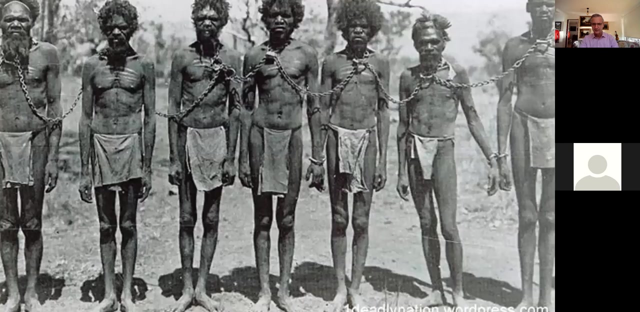 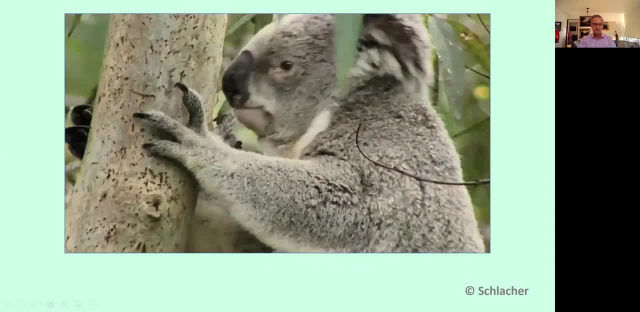 So, essentially, when I showed you the landing of Cook, he landed in Port Jackson, in basically what we call nowadays Sydney Harbour. But you will get that because there is mass to the madness here. But you will get that because there is mass to the madness here. 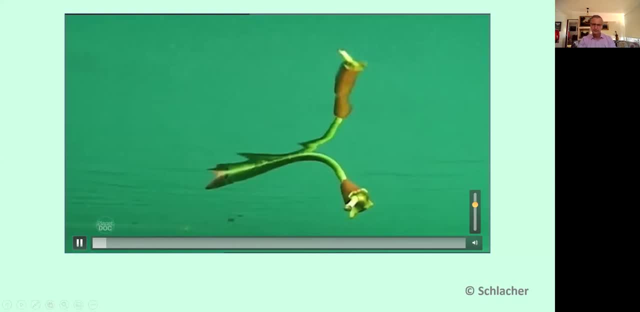 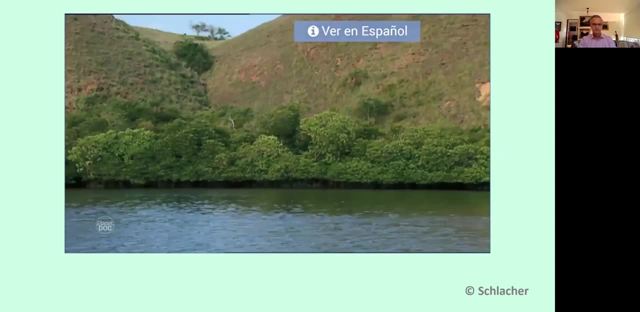 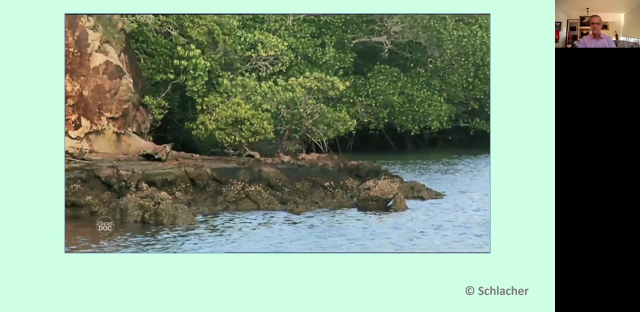 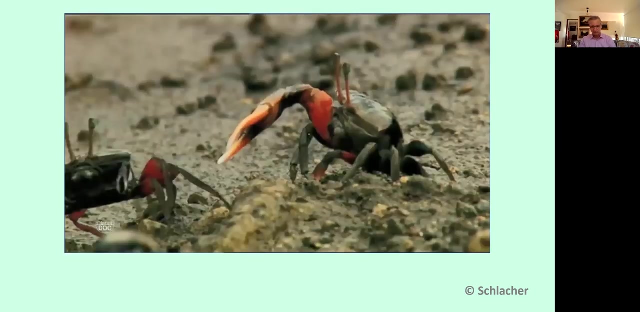 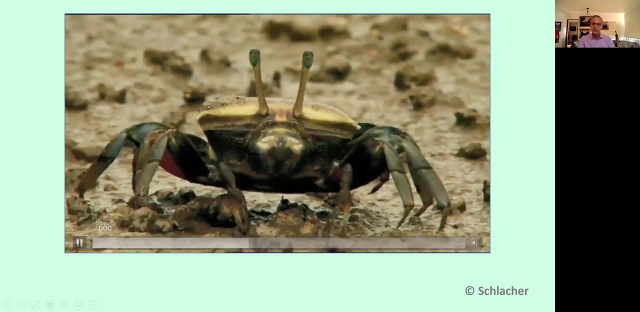 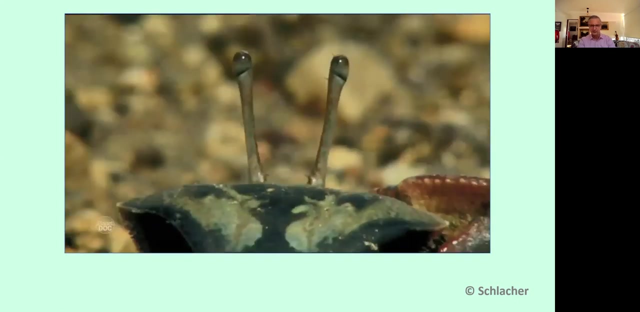 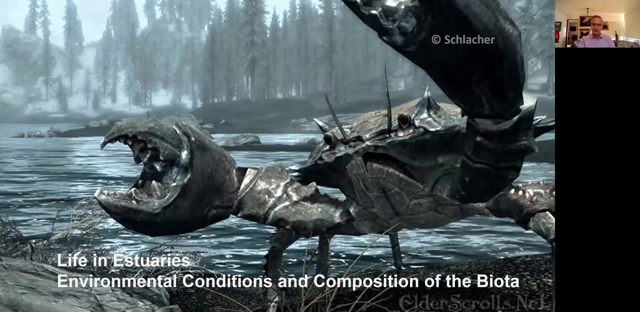 Right, here we go. here's the big grab. Now let's look at life in estuaries. Hang on there. where is myself Now? life in estuaries might seem very idyllic because you're in a sheltered environment. 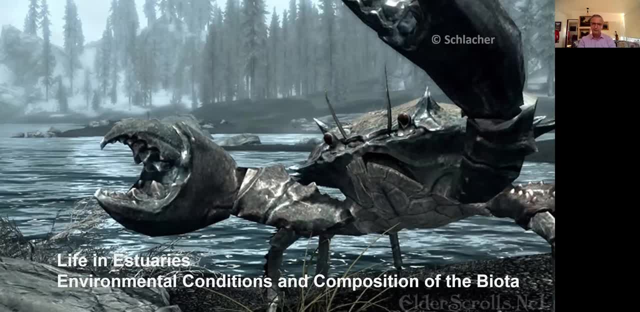 there is not the vicissitudes of waves and currents to deal with, but it might not be, And I ask for your forgiveness, so to speak, or patience of actually sticking with me for a little while to explain life in estuaries and why it is quite difficult. 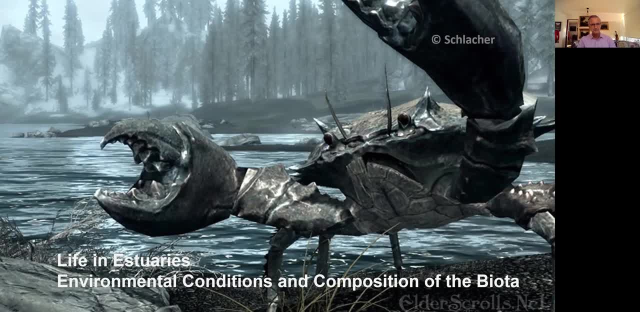 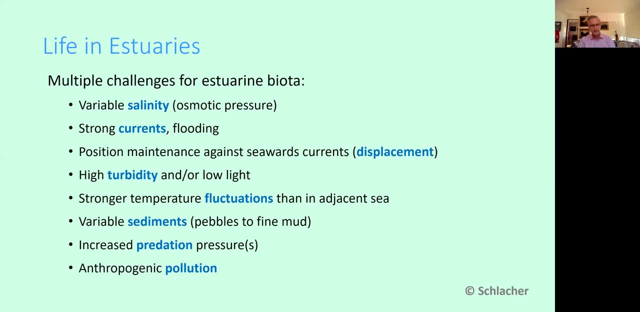 So here is a list of what might be a challenge if you're an estuarine organism. The first one is: salinity can be quite variable. we're going to talk about this quite a bit because salinity is a difficult issue to deal with in terms of the osmotic pressure on your 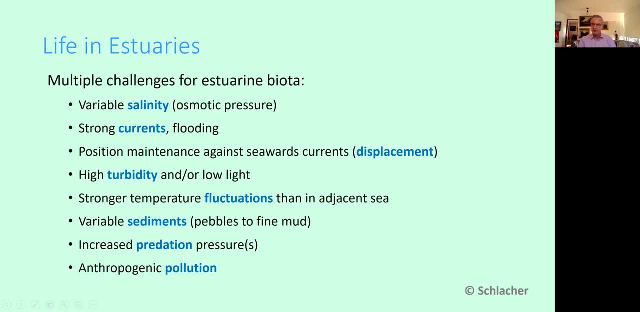 body, If you- I mean we all know that. I mean people die at sea because they're trying to drink salt water. they're alive for us. And you might say, Hmm, why is that? Because of the osmotic pressure. salt is actually a very, very toxic substance in high concentrations. 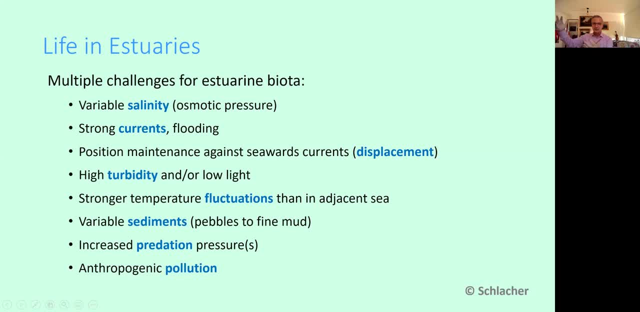 We have strong currents, sometimes our rivers flood and then everything goes out to sea. Now, if you are a crab or a prawn or a fish, it's actually not such a good thing. Now that actually requires you to have some sort of behavioral mechanisms in place to 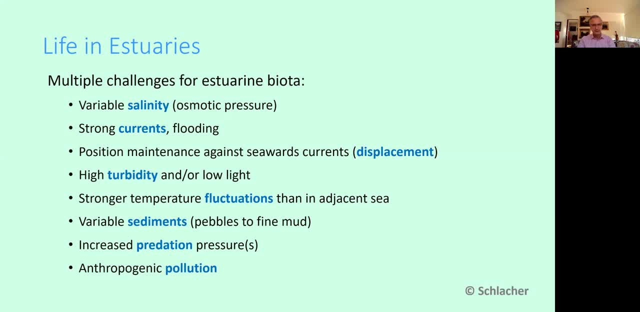 maintain position. Precision often means, you know, avoiding displacement, but a net flow of water from the river out to sea, That can be very turbid. Now, turbidity is a good thing if you are a little prawn trying to be hiding from a fish. 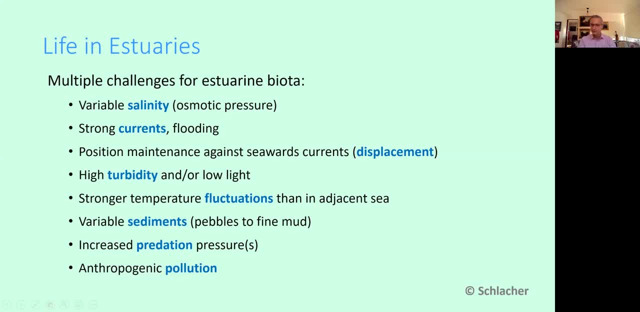 predator. But if you are a plant it's a terrible thing because turbidity means less light filters through the water column and you need light if you're a plant, for filters into this. Temperatures can vary. Temperatures sometimes, you know, fluctuate more, but that's probably not such a big problem. 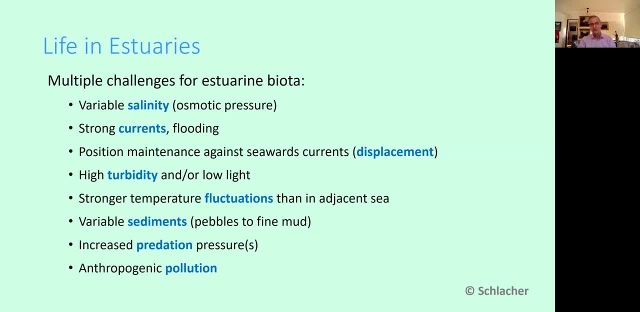 if you live in Queensland, But it is a big problem if you, let's say, live in Scotland or in Norfolk, because you can freeze. You hardly ever freeze. you know, at about 100 meters down in the ocean The sediments can also vary from, you know, being fine paddles to very fine mud. 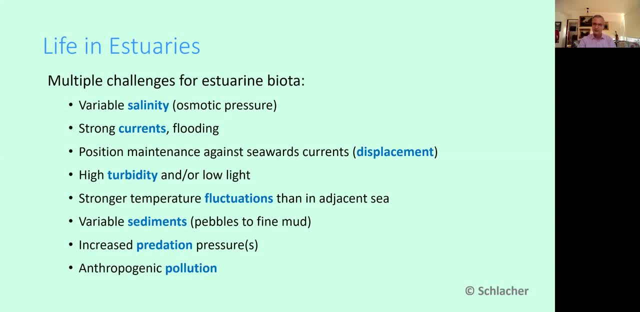 And fine mud is a lovely thing, but it can always be a terrible thing if it actually blocks your skills. It's a fine thing Because it can, you know, cause a lot of damage to the environment. So it's a bit of a debate whether there is increased predation. 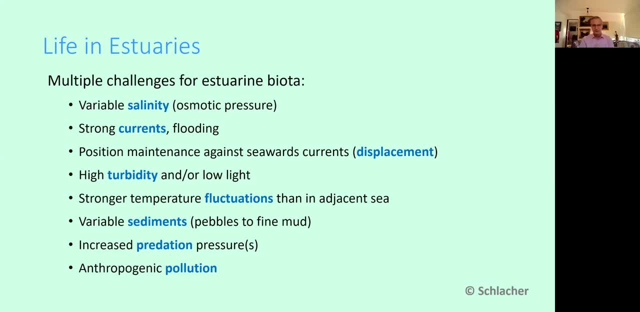 But what certainly happens, because- and that's why I've spent so much time in the introduction of estuaries being the center of civilization- anthropogenic pollution is a big one, And I can show you some of the work we have done in the MoG estuary down swim there ever. 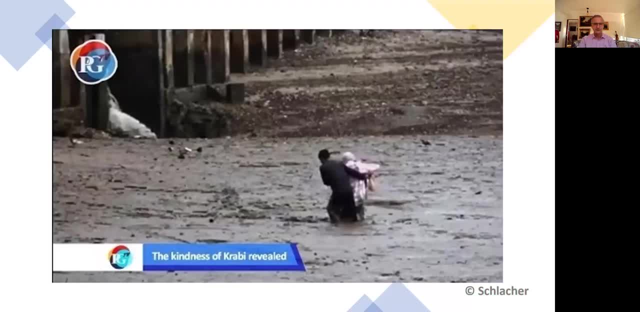 Did I say that No. So I thought: how can I show you how fine the muds are and why mud is such an important thing? Now, estuaries can be very muddy- Ours are very muddy, and I remember the very first time I had 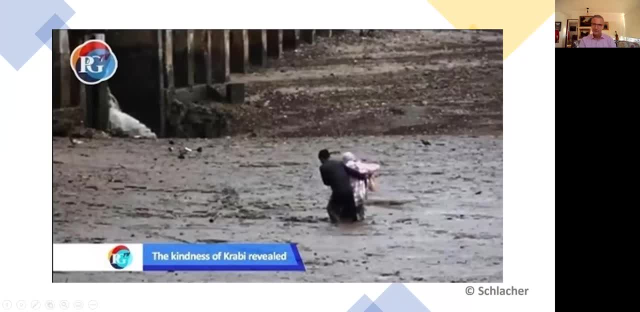 to get out from the boat up at Bullock Creek in the Parisian Basin. I stepped out and tried to push the boat out and I literally submerged to about here in oozy mud, which turned out to be good thing because it actually baked on my body when I climbed into the boat and was a good 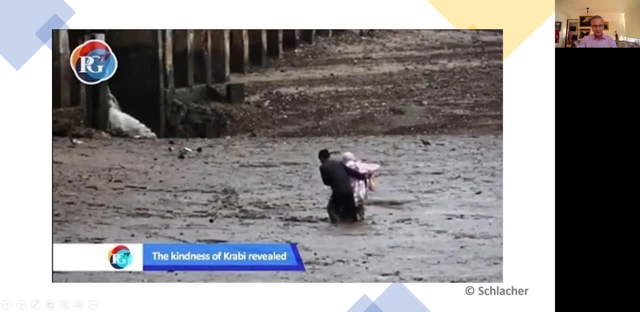 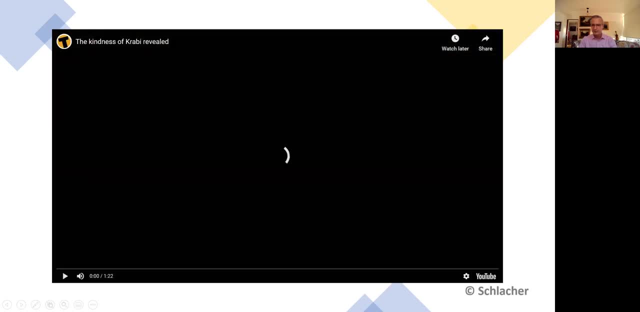 mosquito repellent. But look at this one. Does it actually open? No, Here we go. This is a total crazy story. I couldn't actually believe that. You know, YouTube is fantastic. You go- how do I illustrate that? estuaries have fine mud And here is two pommies. Look at the pommies trying to. 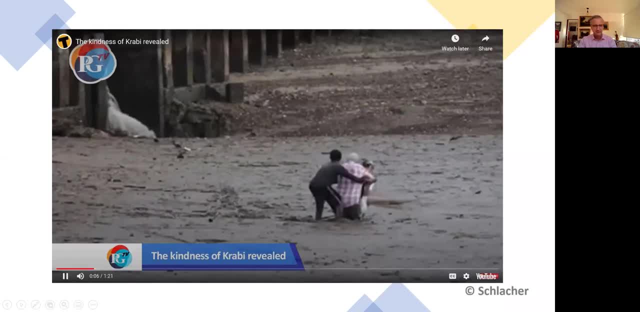 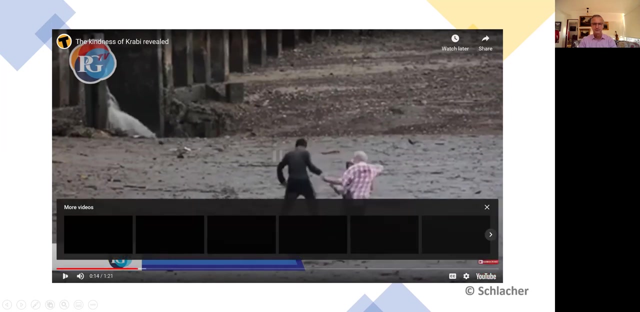 photograph birds. Sorry, It does my internet connection Come on. They themselves stuck knee deep in the mud of a crabby river estuary. Local hero chatting along, Jinda 44 left into action The tourist Norwegian photographer, Harold Hayden. Ah, Norwegian, sorry, not pommies. 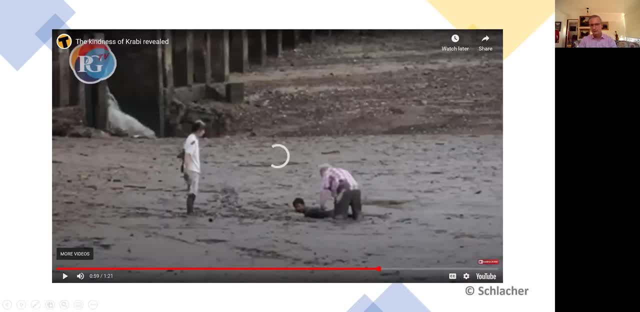 Ah, I got it. This is the problem with online teaching, because, of course, everybody in Mooloolabaat shares the same internet line as we all do. you know Telstra, And what is the time now? Yeah, it's 20 to 5. People are actually starting to actually watch Netflix, But so what's this guy did? 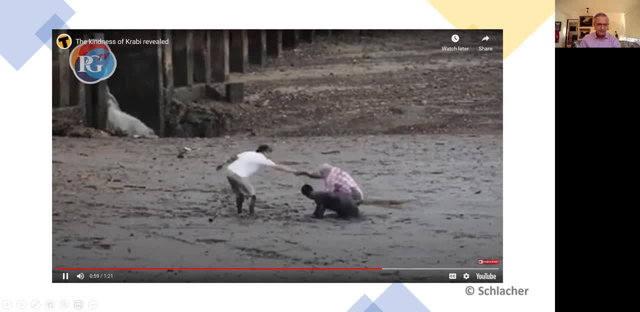 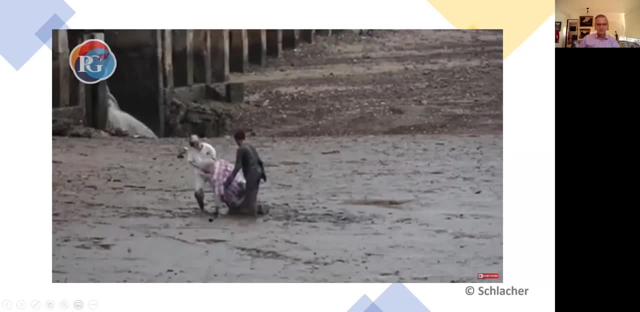 This video by Tirrasek Samshi Tawi went viral over the weekend, with over 200,000 views in just a few hours, And thanks to that, crabby governor Pinnit Boonlert and the tourists were able to track down Mr Chat and reward him. 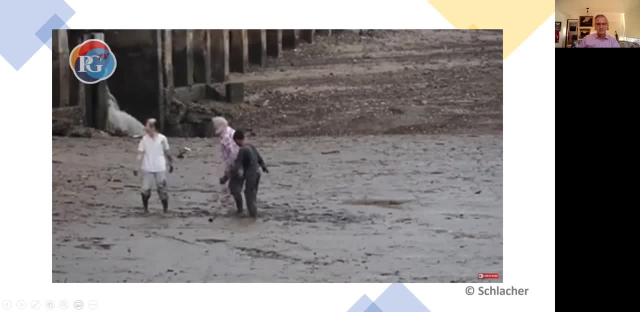 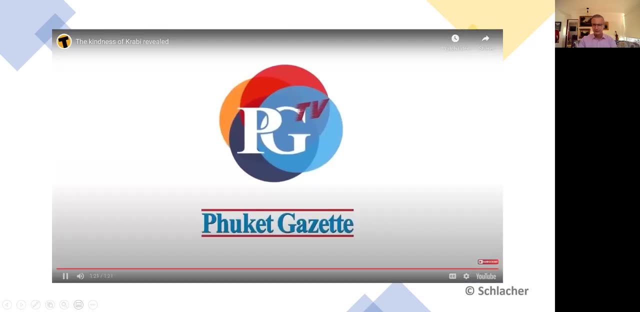 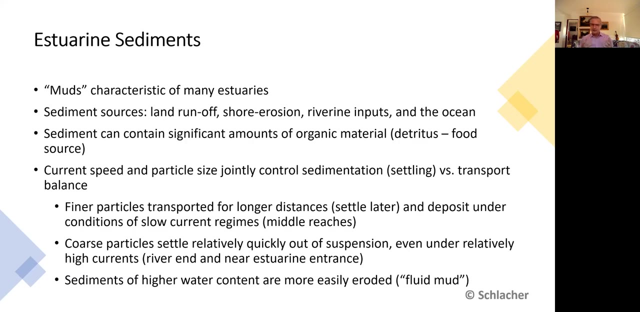 For his kindness. So soft mud. Why is that a problem? Well, mud is the main characteristic of estuaries. It's the deep sea, oddly enough, and estuaries So the very shallowest part of our oceans and the deepest part, And there's an explanation for that. 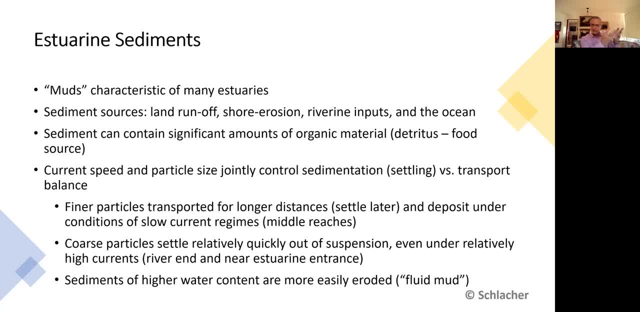 Because currents are usually weak, modest, a little bit ambling around in estuaries So mud can actually settle there. But also because this is where basically mud flushes in as terrestrial runoff from the hillsides And mud we again we have in the deep sea, because that's where the currents slow right down. 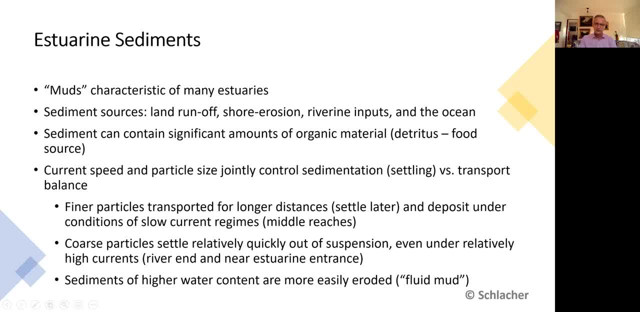 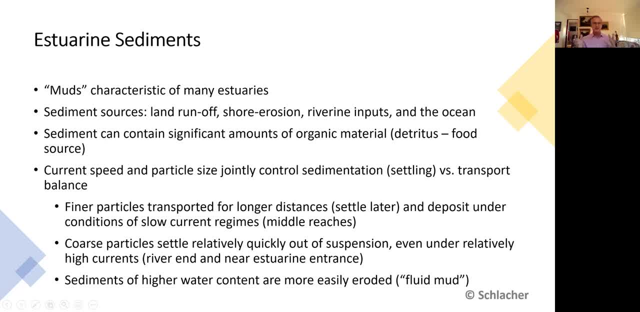 Now detritus is. you know we talk about detrital deposits sometimes, or somebody's a bit of detritus in a, in a very in a derogatory way. But formally speaking, detritus is a dead plant, Mostly dislocated, uprooted, floating around right at the bottom. So any bits of plants. 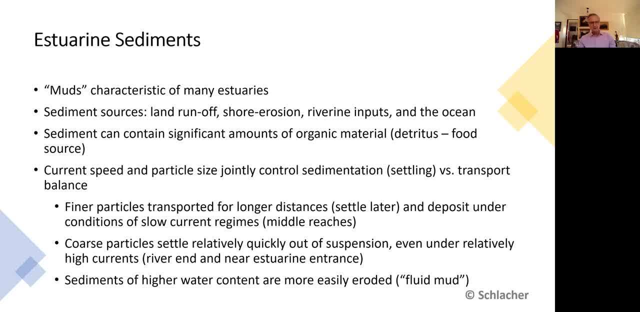 you know, shed leaves, shed branches, which are not attached to the plant anymore and which are dead, are detritus. The animal equivalent- and I work on that- are, of course, cadavers or carcasses or caraham. So a dead animal is a carcass or a caraham or a cadaver when you talk about humans. 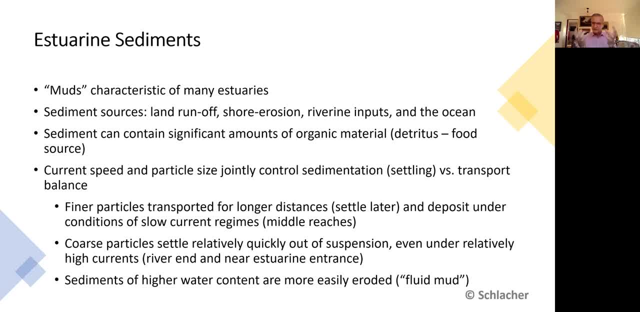 Whereas a dead plant is detritus. They're the same thing really. it's basic Carbon, which is very, which is not running away from you anymore and you can eat it, and it's very, very important. Now, essentially, you get mud because it is the interplay between current speed and particle. 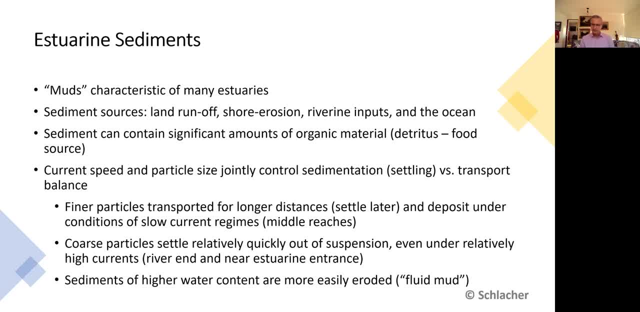 size which determine settling velocity. Why is that? Essentially, fine particles stay in suspension for a long time and they settle later, whereas coarse particles usually get transported. you know further, and that's why the very fine muds you often find up the S3 and the bottom of the S3 is quite often sandy. It's all about currents. You can actually 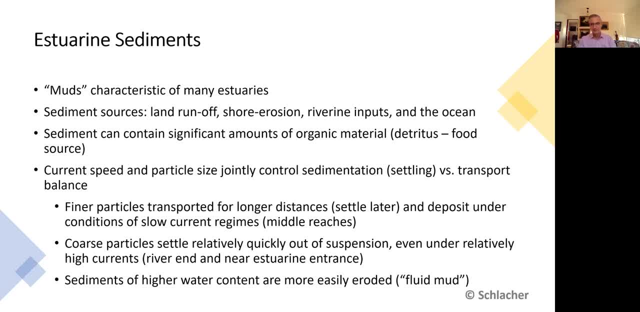 investigate or prove me here. you know right, because I'm not going to be wrong in any of our rivers. here the very you know most seawater part is used. It's usually a nice sandy bottom and as you go up it becomes muddy. 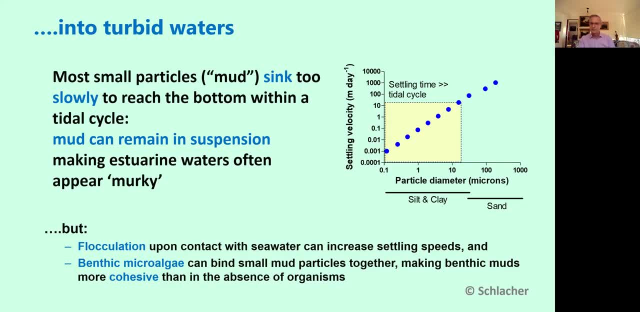 Now this is quite curious If you are in Brisbane, and I think we can officially go there- again fifty kilometers- but whatever you know, we can't go to Fraser Island. I try it all day to day to actually go up there. 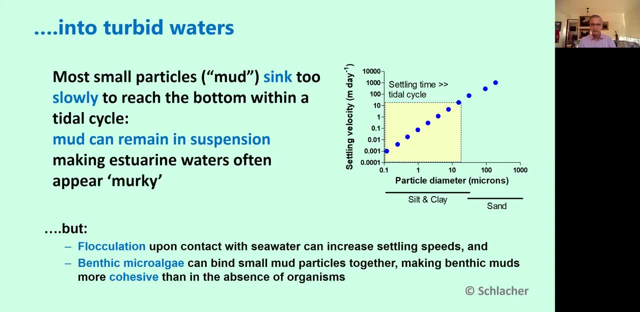 but the island has been treated as well as a quarantine place for the indigenous people and so essentially it's closed for quite a long time. but let's see how it goes now. but if you go to Brisbane and you walk between the casino towards the museum and the Arts Complex there and you stand, 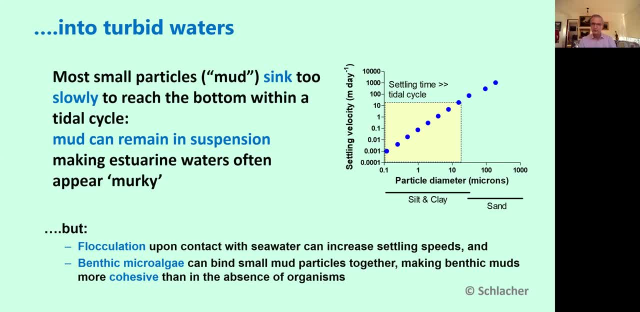 on a bridge and you look down, most people say, whoa, the Brisbane River is really polluted. here we go. who works on crows? he comes in a three times a day. it's quite interesting actually. I actually wonder whether we got everybody complains about the crows. we actually got more crows now. maybe they have to come. 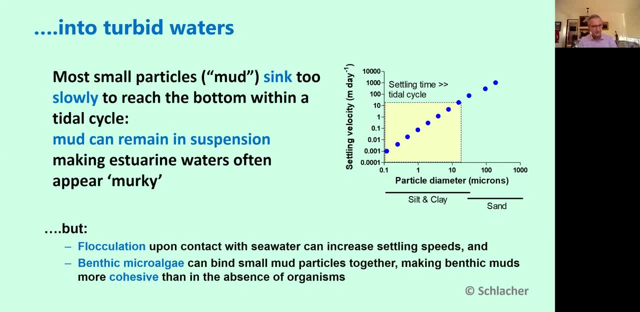 and feed on the estuaries because the campgrounds are all empty. here it goes. so you look down on the Brisbane River, on the bridge from the Cholley Bridge, and it looks really round and murky and turquoise. the reason for that is because it's really polluted, because it's really polluted, because it's. 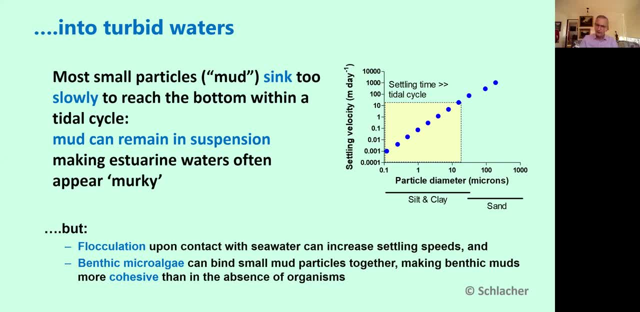 it is that the currents are very, very strong, so essentially they keep the mud in suspension. so what you have is a very, very fine diameter sediment- about 10 micrometers- and essentially it takes, you know, more than three or four tidal cycles to reach the bottom. now, a tidal cycle is six or seven hours, so it's 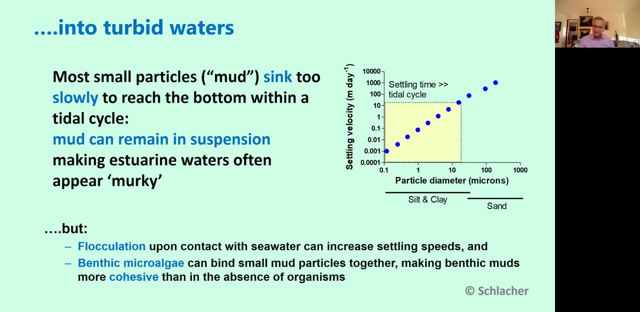 actually they never have a chance to properly settle. but the Brisbane River was never really that turbid and we kind of figured it out a few years ago and said, well, why is it so turbid? because the currents are a lot stronger. why the currents are a lot stronger? because the ships coming in at the bottom of the Brisbane. 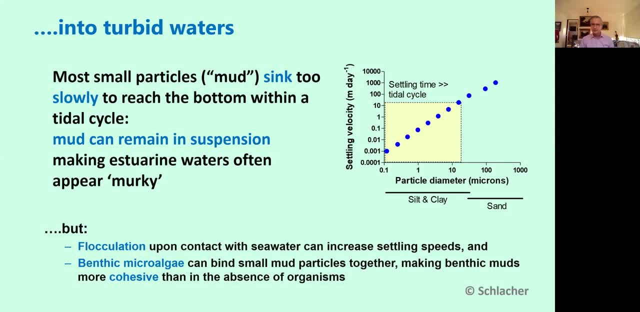 River next to the airport- on the other side is the harbour- have become bigger so they have to dredge out the river mouths much deeper for the bigger ships to come in and dock. now a bigger and wider and deeper channel meant the currents going up the Brisbane. 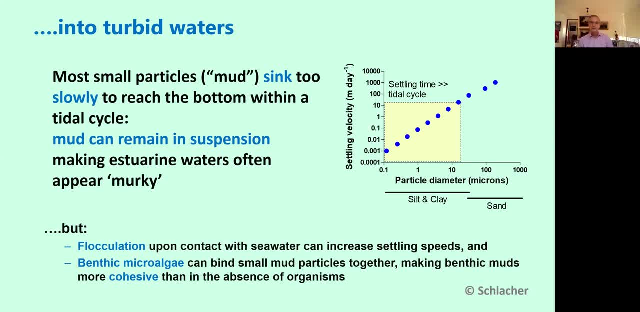 River all the way the Brisbane Estuary, I should say all the way to the Choddy Bridge, are of course much stronger, so they keep all this mud which has settled there for centuries now in suspension. so this is actually a curious side effect that the city of Brisbane desperately 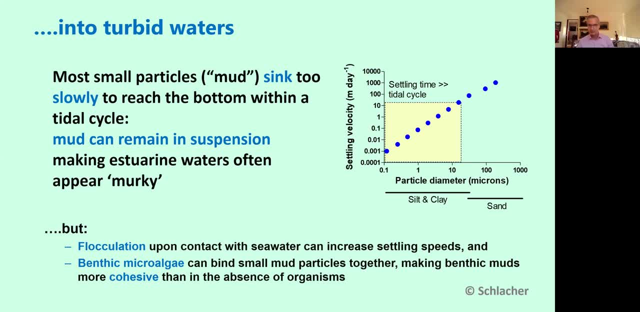 wants a kind of bluish looking, or at least greenish looking river, but it's never going to get it because the port of Brisbane needs a deep channel, and a deep channel basically means strong currents moving up river. so here you go. now you can make estuarine waters less. 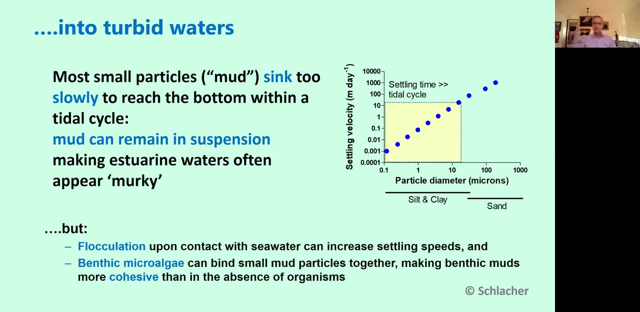 turbid, and that means sometimes, when mud interacts with salt water, it actually flocculates and it settles to the bottom, or when you have benthic microalgae, a fine film of very small plants right at the surface, binding it all together, and we're going to talk about the importance of benthic microalgae. 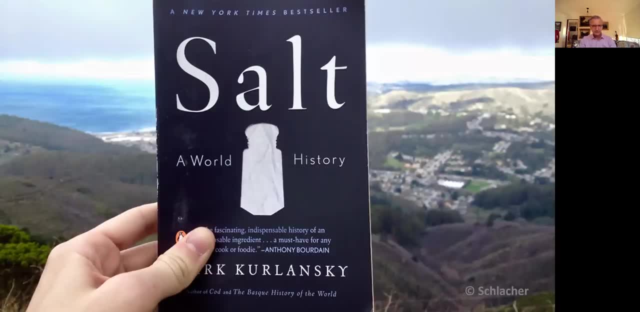 in about 42 minutes now. I recommend to everybody to read that book here. salt: we're going to talk a little bit about salt here, because living in an estuary is all about managing soil, changing salt concentrations. it's an excellent book, so of course it was a very, very excellent. 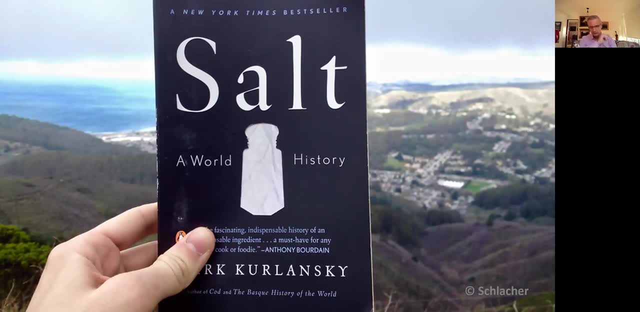 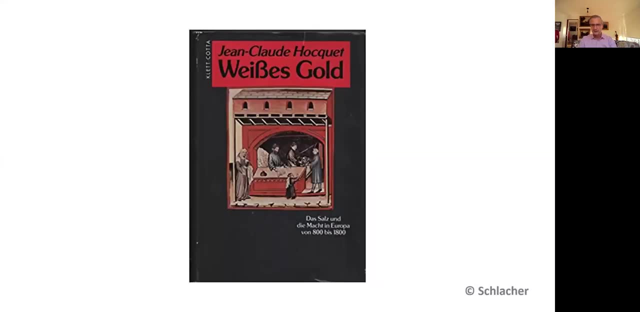 because you know my village has two chapters in it, because you're in the oldest salt mine in the world. but never mind. and why is it actually so important? well, unfortunately there's only, you know, a German book here: Vices gold basically means white gold and salt, right. 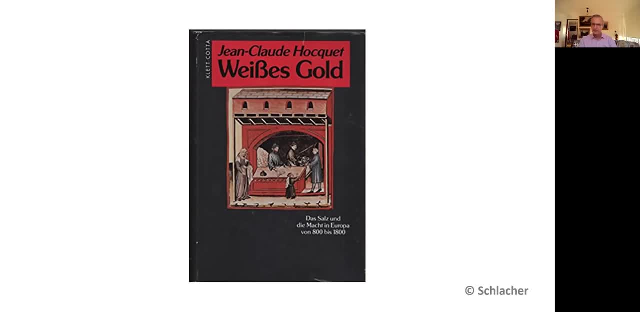 up to about 2 or 300 years ago was more valuable than salt should have been. so we we would have done a lot over and over because, seeing salt on the stats, it would have had negative impact on the salt climate. but there's a got plant economy. 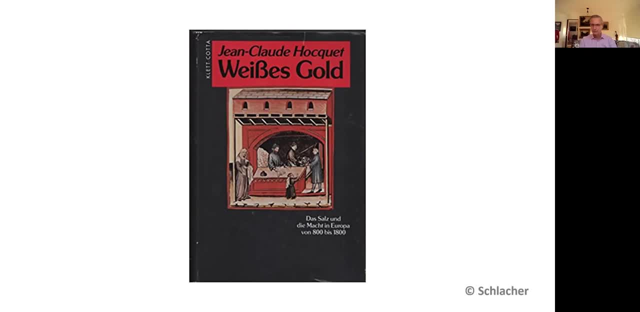 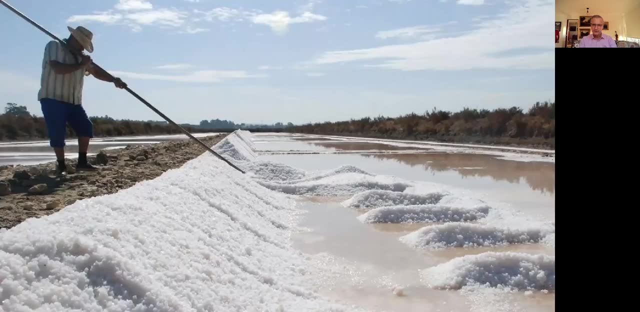 and while lots of different sorts of fish finding salt happening here, you can literally find things that that号 can't find. then try to Roz fish. can you catch some cool fish like soient, hortensia sanphia than gold? You might say what Why? Well, wait a second. So here's a guy in southern Spain producing salt, And mankind has for many, many millennia tried to harvest salt from the ocean or from mountain deposits, which basically captured during the mountain formation. shallow seas compressed the water literally out of the rock and the salt stayed behind. This is how the salt mines got created, And if you buy Himalayan rock salt, there's actually. 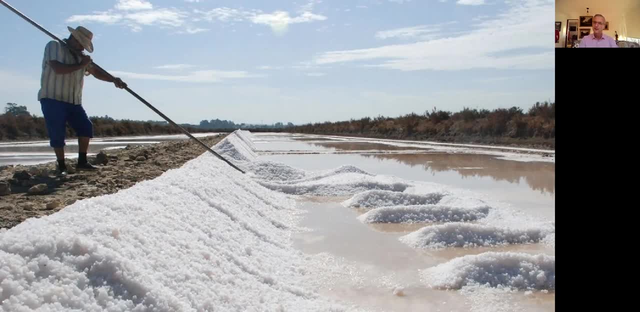 up to a day's worth of salt in the Himalayas in that kind of form. It actually all comes from Germany and Austria and France, but never mind. So, oh, I should actually show you that. So this is the good thing you know, when you actually teach at home, you can actually 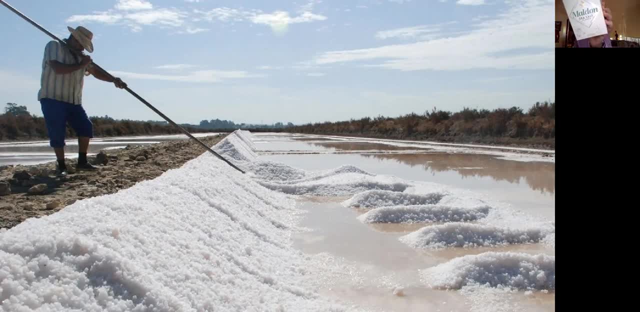 get quickly a prop. So here we go: Meltdown sea salt flakes. It's a very, very expensive salt. I have no shares in it, But you know what? It changes your cooking completely. If you have a salt, that salt is salt and it all tastes just salty. This comes from. the North Sea because all the pollutants are captured in it. But I once had it many years ago in Spain on some goose liver organically farmed- I actually knew a few of the geese- and it tastes completely different than normal salt. It's. 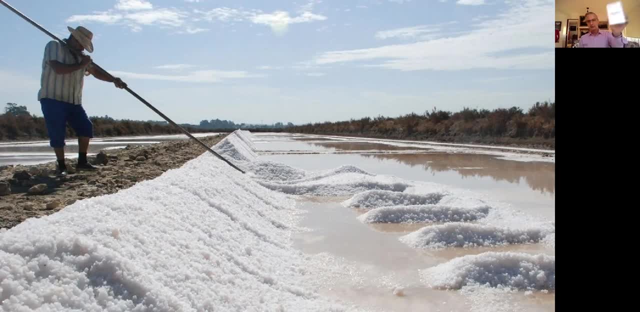 really well worth it. if you like your food, Buy some of the sea salt flakes. And this is how it's made: You basically put sea water into a shallow pan in the ground, let it evaporate, and as it evaporates you put it in a jar. And then you put it in a jar and you put it. 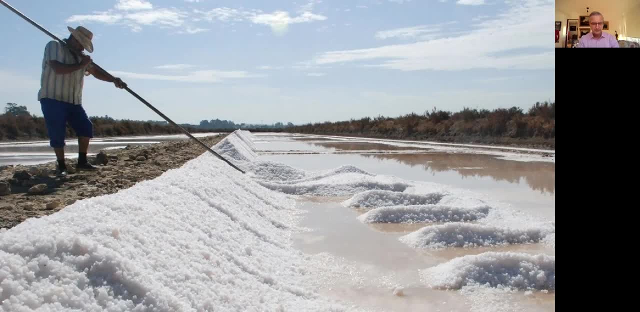 in a jar with a little bit of salt. You see, It evaporates, It becomes salt salt and eventually it crystallizes out. However, the traditional way of actually making salt comes from having salt mines in mountains, And this is kind of great, You know. this is great because 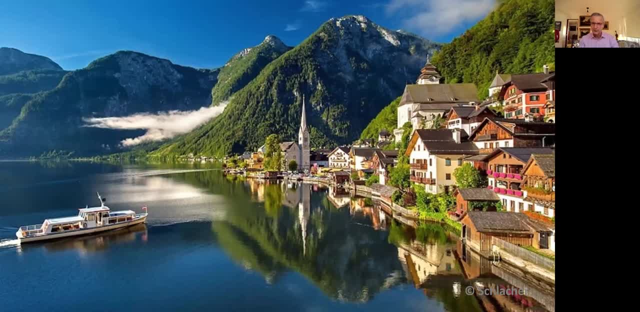 this is the same picture you get when you buy a TV at Harvey Norman, or a choice of anyone who goes to the TVs- and to have like five or 10 pictures which actually runs over. And every time I go there I'm like whoa, here's my house. 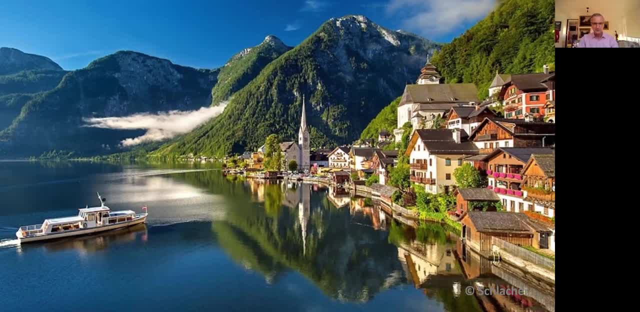 Whoa, here's my house. Whoa, here's my house. Here we go. So, basically, we come to this village here called Hodgetup. Our house is about 7,000 years old and it sits there And it has all this salt mine in the world because people actually 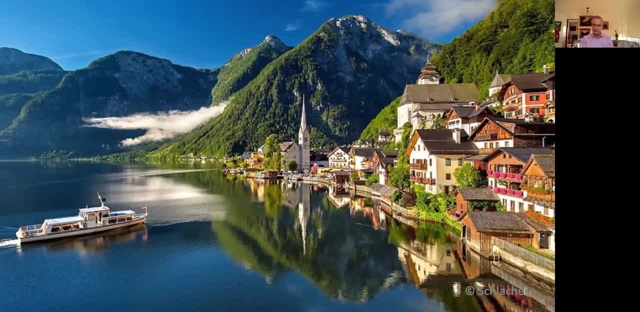 discovered that one of those mountains here as it got folded. it must have literally folded in a shallow embayment like probably a very big estuary, and all the salt just basically got contained. Very, very convenient. This is actually a boat. 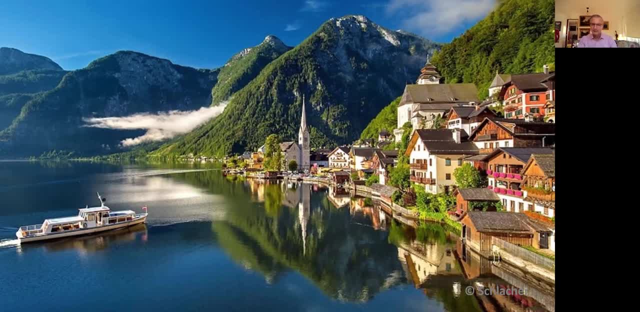 We took it to school which is on the other side here And whenever we had a teacher who was new and we were late, he's like, oh, we missed the boat And that's like what We did, what They didn't actually know that in the next valley, where the high school 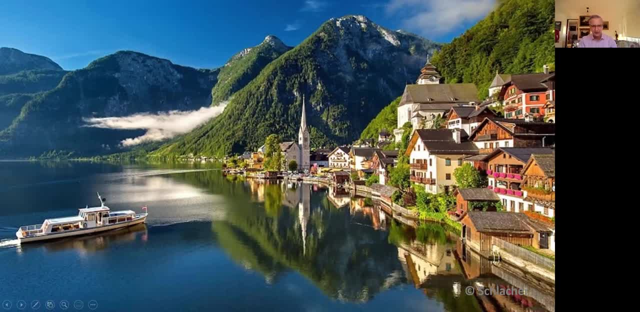 was that we had to go across the lake And, of course, in winter you skated across the lake, which is also kind of funny because when I quite knew whether the ice would actually break and a few people actually died. I'm not kidding, but here you go. 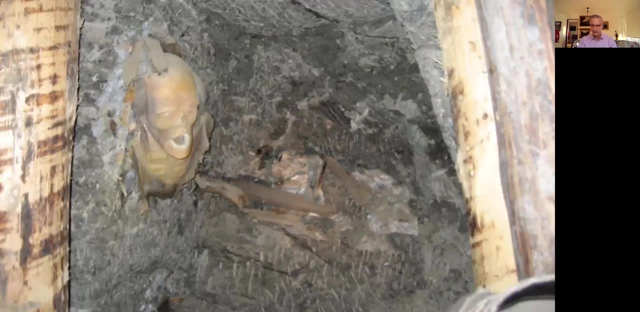 Anyways. and so what happens in the salt mine? A few years ago they found- this is a reconstruction. They found a salt miner who must have fallen into one of the bits where the salt concentration was very high, And he was called the man of the salt. 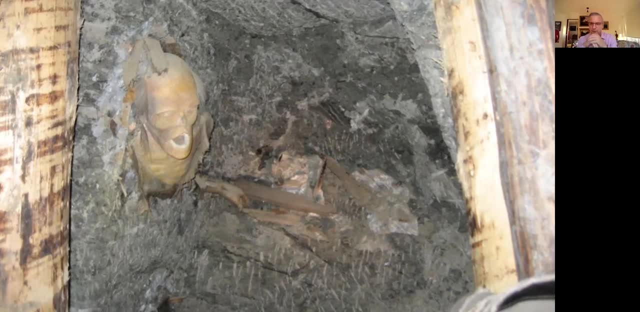 And it was a major discovery because he was incredibly well preserved. Now, think about the word I just used: preserved. If you want to preserve, if you want to preserve food, and you don't have a fridge and you don't have a cannery, what do you do? 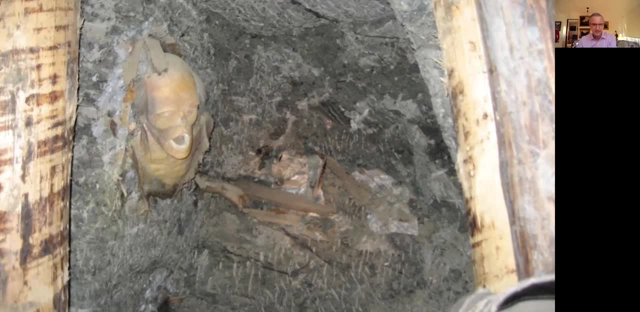 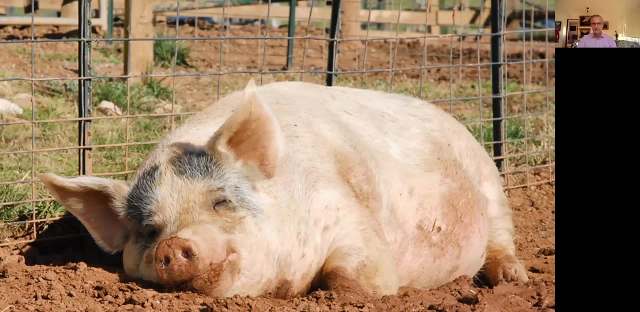 You basically put it in a salt solution, And this is the whole idea. Here is a very content big, And this is the big- not so content anymore, I guess, but you can actually eat it and you can actually store it for a long time. 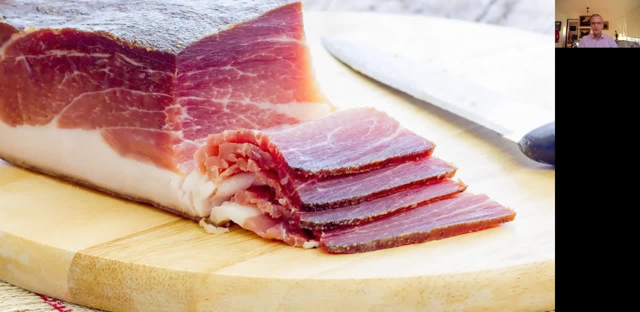 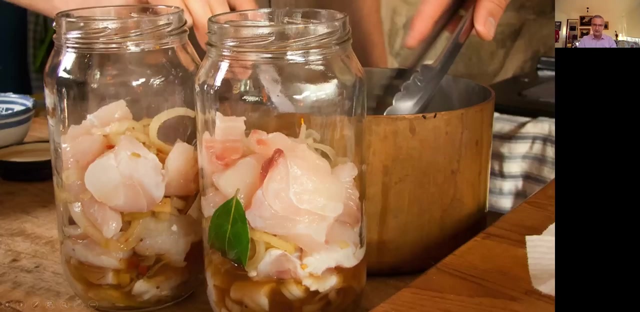 This is bacon, any form of bacon. When you make bacon, you cure it in salt And then usually you smoke it or you try. You say, okay, this is the new age, I shouldn't show you pigs and bacon. If you like pickled fish, here you go. you basically cut it up. 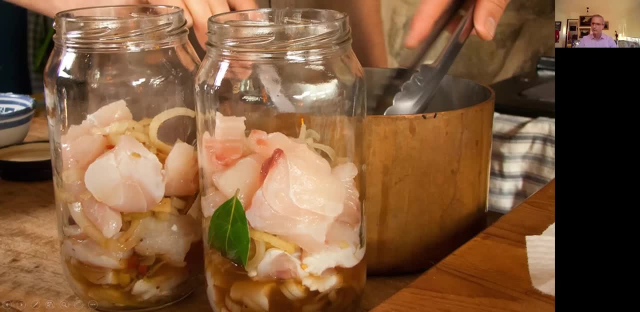 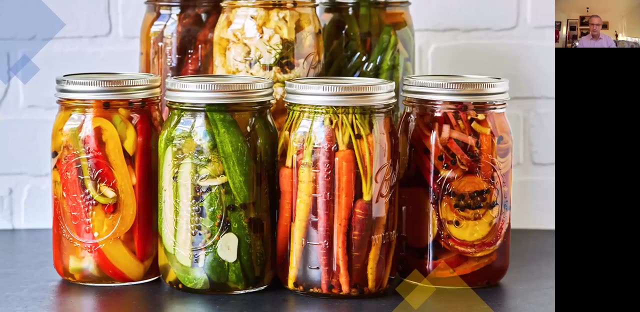 And then you pour over a salt and vinegar solution. That's the vinegar that makes the taste, but the salt is the preservative, And you can do exactly the same with vegetables. As a matter of fact, I discovered lately that making your own preserves 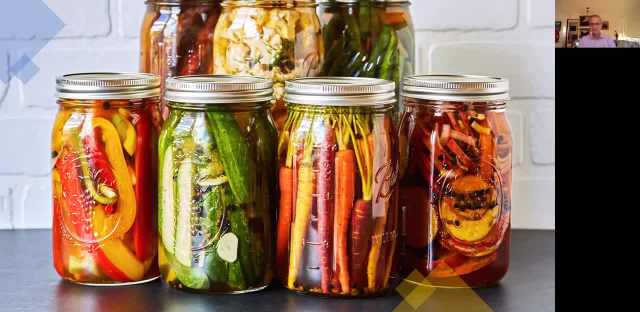 is one of the great comebacks or renaissance of the Corona crisis, Which is kind of really, really, I think, paradoxical for me, because when we were children, we had to eat bloody pickled stuff for an entire winter And we couldn't actually wait to get fresh stuff anymore. 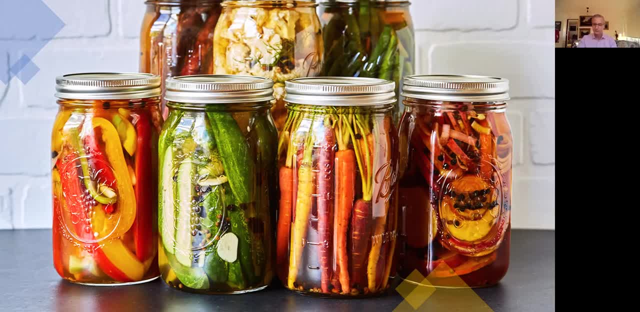 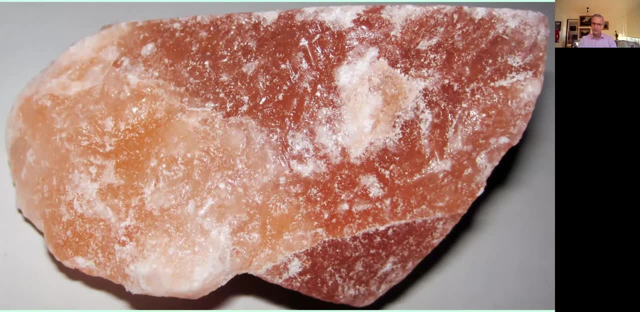 Nowadays it's a delicacy because basically that's how you preserve stuff. But let's sort of go. Why salt is so important? The first thing you have to think about this is a piece of rock salt of that size. Now you might ask yourself: how do I get salt into solution? 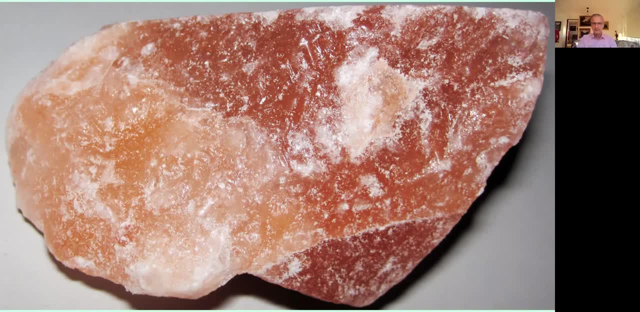 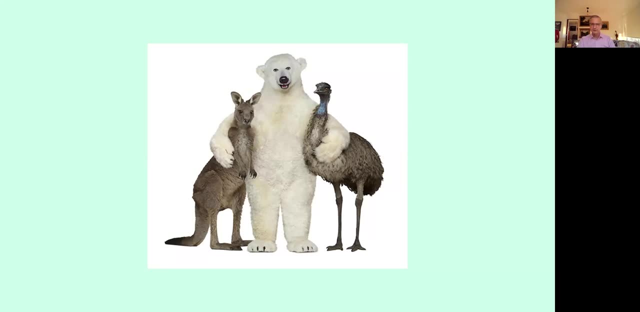 It's a fairly rock hard substance. It's not easy to dissolve salt, However, so I thought: how can I find an Australian example of a polar substance? And I don't know why this came up. So this is the Bundy Grum Bear. 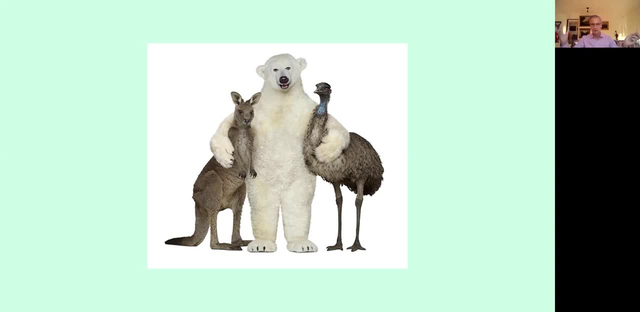 I you know, and it comes up because he's very polar and it comes polar bear Here. he is Bundy Bear Grum And it has two mates here, a kangaroo and a Nemo. So you can actually view this as a polar substance. 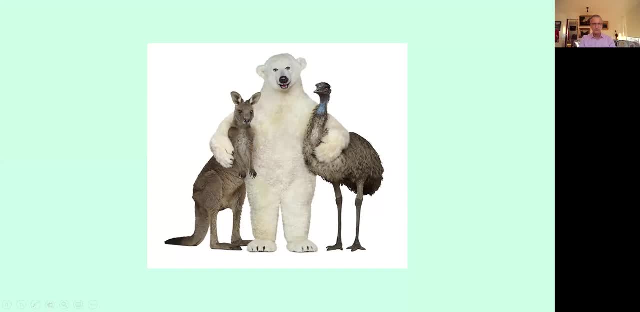 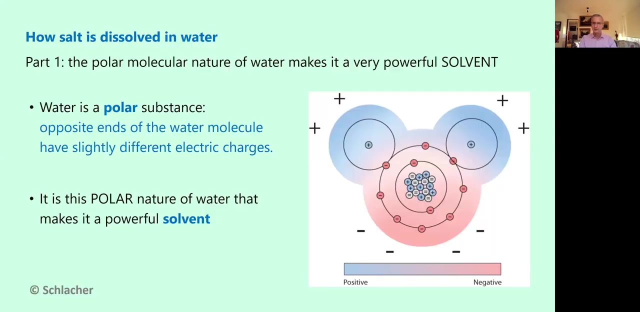 There's two gray-brown organisms here, And in the middle is the big polar bear. Now, why am I showing you this? Because it is, of course, exactly the same as the water molecule. The water molecule is a polar substance. 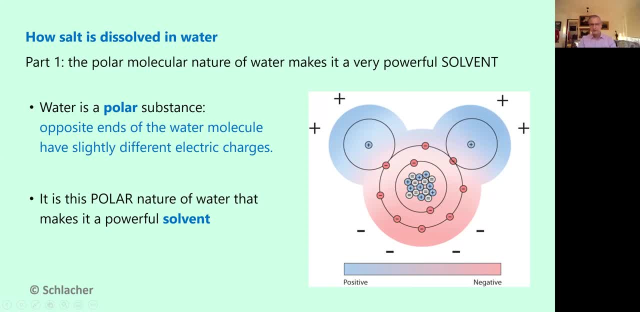 It almost looks like a Mickey Mouse here, But essentially, here we got the oxygen molecule and here we got the two hydrogen ones, And, as you can see, the hydrogen ones are positively charged and the oxygen one is negatively charged. Now why is that important? 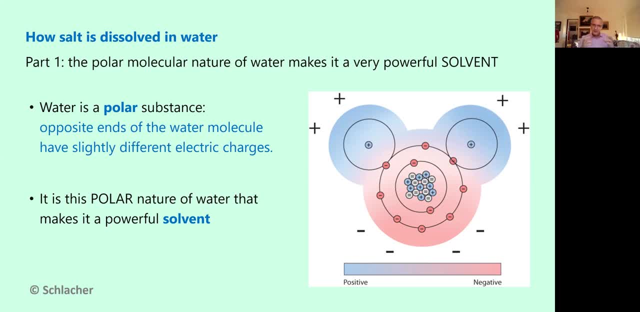 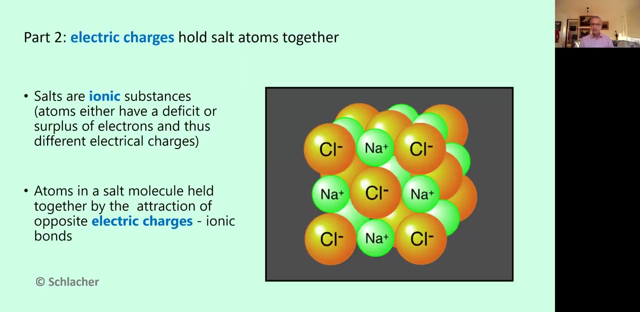 A polar substance acts really really well as a solvent when you have a material which is also held together by electrical charges, such as salt, sodium, chloride, taru. So all you have to do, basically, is hit a molecule held together by electrical charges. 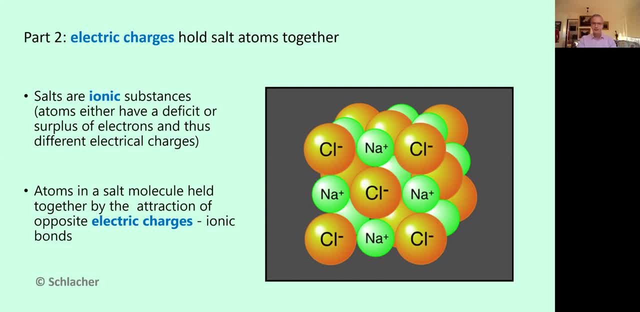 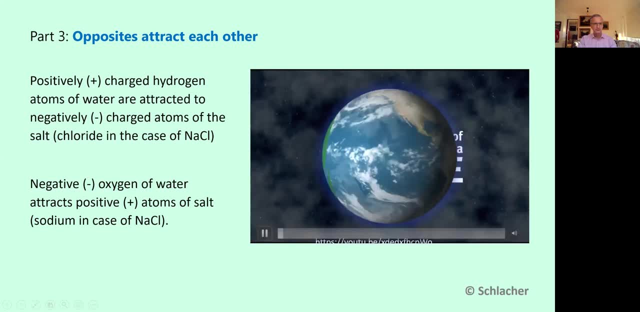 with another electric charge, which is the water molecule, And it falls apart. Look at this one. Here we go, Opposites attract each other. The Canadians made something very, very interesting. I suppose this is something you watch on a flight. 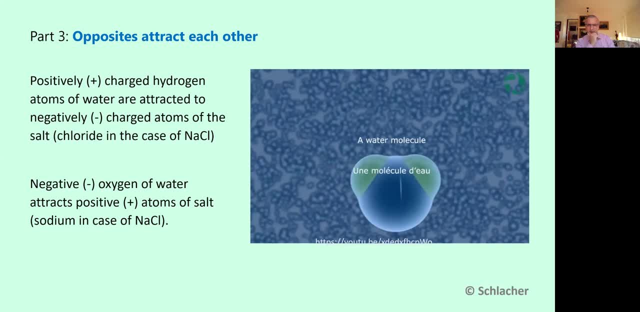 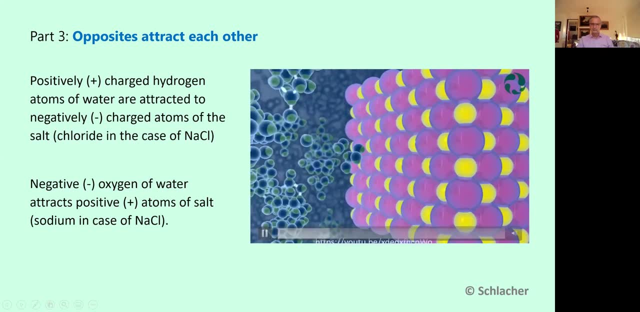 at about 2 o'clock in the morning And you go like, Oh, this is quite fascinating, But basically those little blue things with the green ears are the water molecules And here's the salt crystal. What a big lump of rock I just basically showed you. 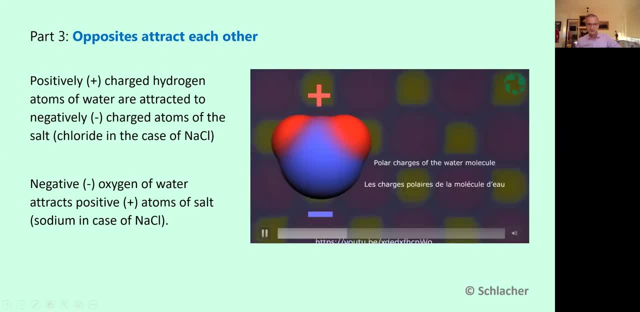 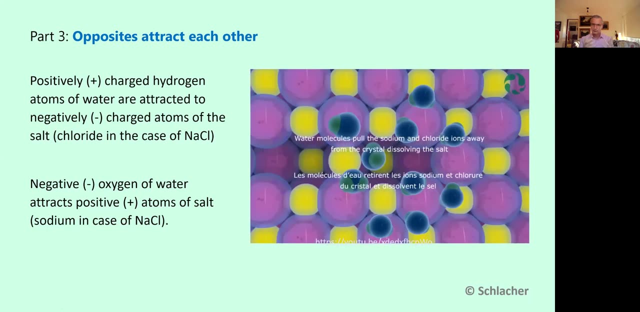 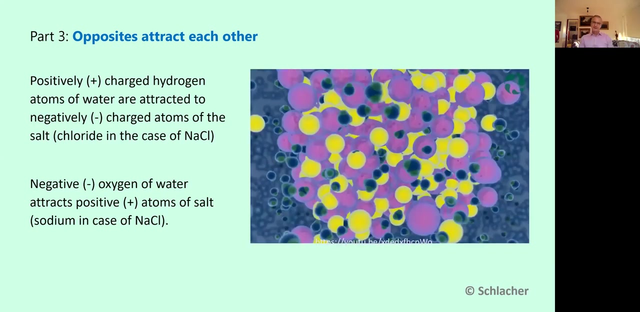 And so we see it's a charged surface. Here we go, blah, blah, blah, and as it actually interacts with the salt crystalline structure, it breaks it up. So the salting powder of water as a polar substance is pretty much determined by the interaction of erosions and salt being a ionic molecule. 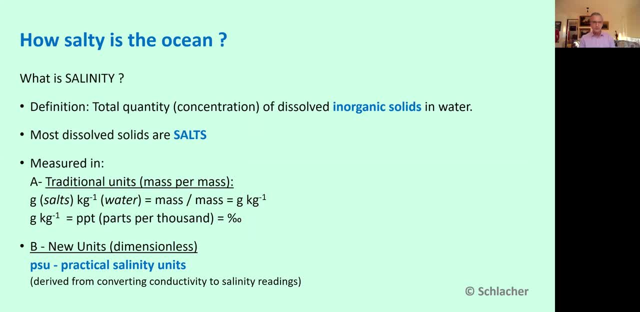 being held together by electric charges. This is quite important. Now you might actually say you know, this is just a little bit of technical jargon, but traditionally speaking, we talk about grams per kilogram or parts per million, parts per thousand, or we talk nowadays about practically salinity units, which is 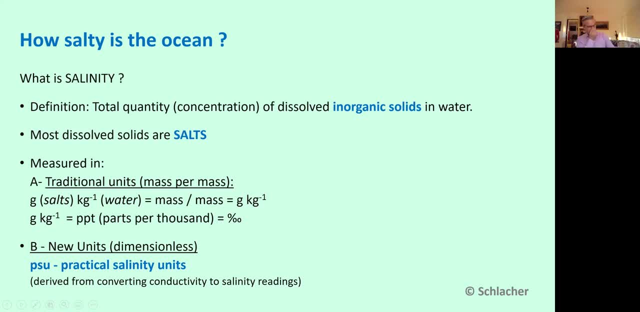 more or less the same as this one. Now I need another prop. Oh, here we go. You always have to have a chin and tonic, you know, kind of ready. So this is about a litre of you know water. Just imagine this is water and not chin. If I would. 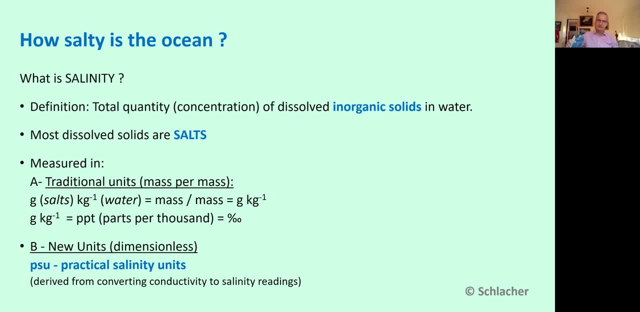 actually go out and basically you go out in the ocean anywhere along the coast here and you take a litre of that home and then you put it in a pot, Right, And you boil it up. How much salt would you actually get out of a litre of seawater? 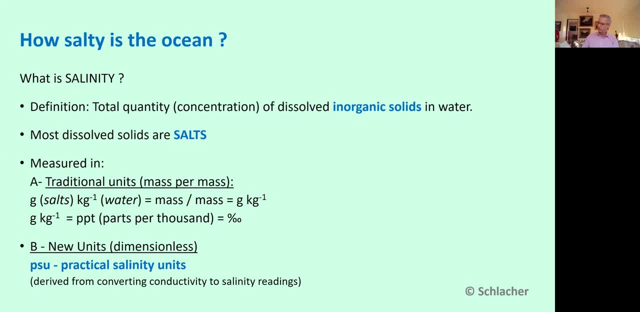 You know What do you actually get? There is 240 grams in this packet, which is kind of, you know, reasonably sized. Now here's a pencil to actually show you. So how much salt would you get out of a litre of seawater? A litre of seawater is not terribly much, is it So? 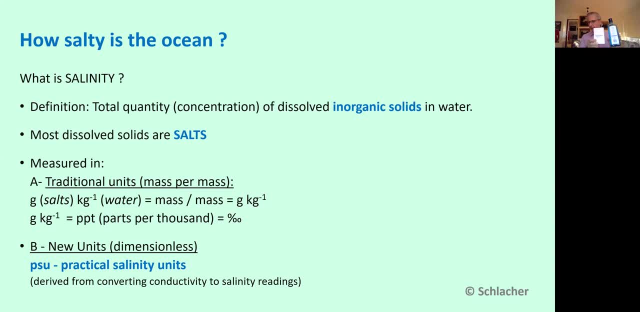 how many litres of that would you need to make a packet of salt? Anybody guess? Isn't it about 40 grams of salt per litre? That's a lot of salt, you know? 40 grams. Think about it. You would only need eight. 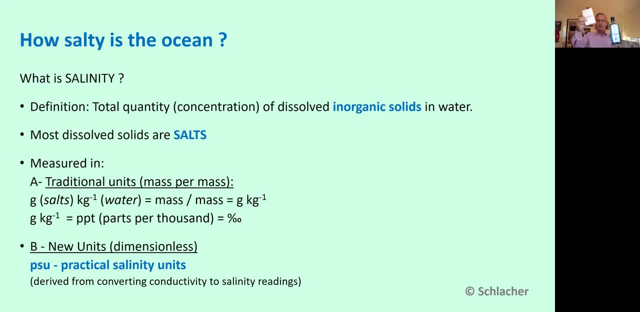 litres to make a packet of salt. And if you think about it, a packet of salt like this- because it's a very special sort- costs about, you know, eight bucks. That's the best kind of deal in the world ever because you bought those free. 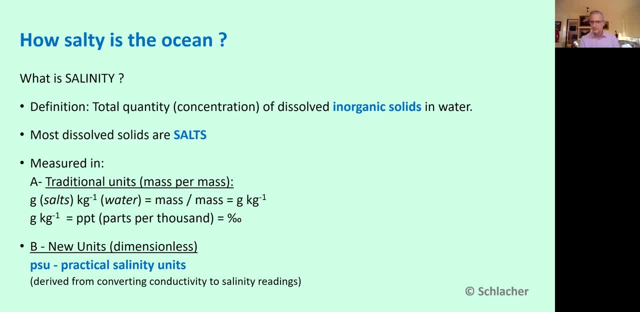 40 grams. that's quite a bit, isn't it? Any other guess? I could make myself a gin and tonic in the meantime. huh, It's only like about 3% or something, isn't it? Yes, and 3% it basically what you get out of a litre of water. you get between um. 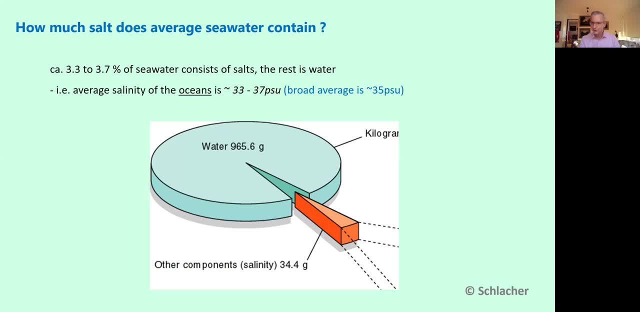 basically 30 and 40, you're both right- grams of salt. So actually seawater contains a lot of salt. Now here's a curious one. If you don't want to buy expensive sea salt, you know, take a bucket down to the sea and put it in a pot. If you make a fire at home, 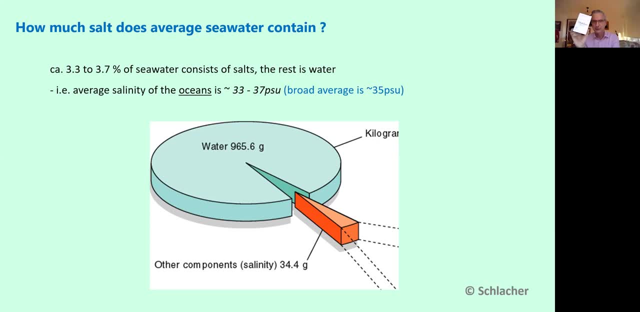 it costs you nothing And you evaporate it and you scrap the salt out And you've got exactly the same, sometimes from a cleaner ocean than what you buy. I shouldn't really promote that. I should actually do it myself. But actually you can make salt very, very. 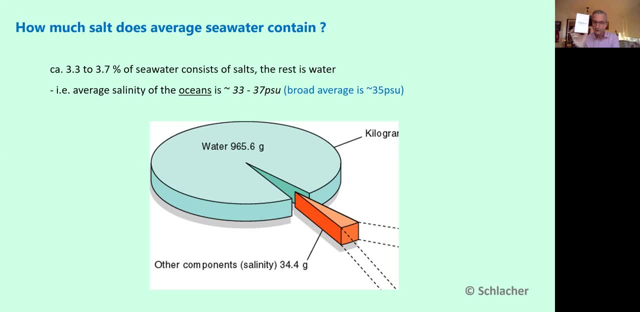 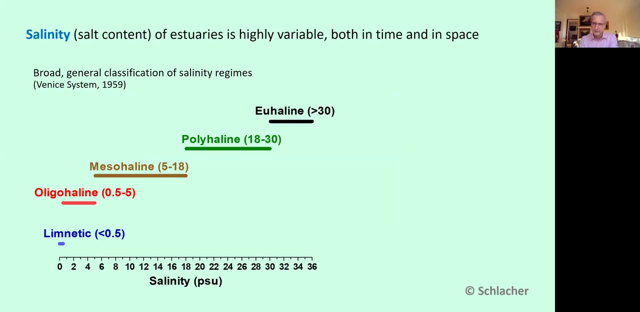 simple, your salt, because the ocean is very, very salty. So 35 grams or whatever, on average is a reasonable amount of salt. So here you go. So what, what? and somebody came up then you know, and a classification You might come across. this, you know, you hail. 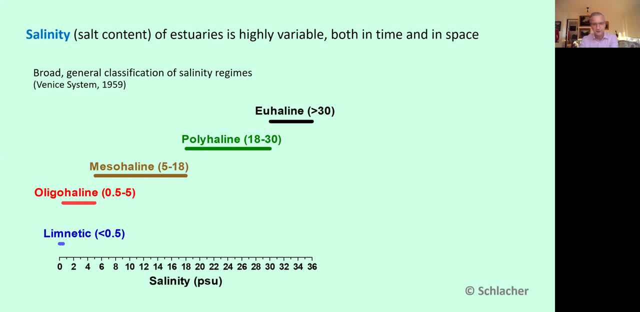 line is basically fully marine. Fully hail line is sort of you know in between, And then we come towards the freshwater areas. Now, all freshwater contains a little bit of salt as well, And this is why you should never, ever drink distilled water or deionized 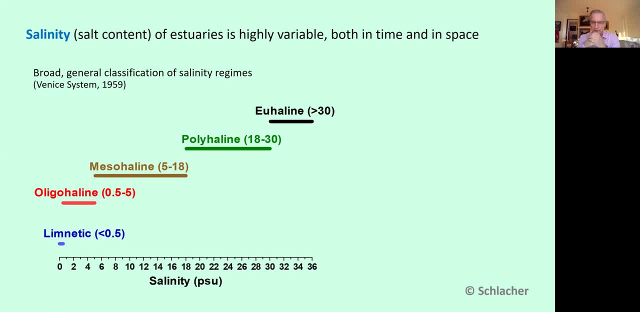 water from the lab because it will actually, just like seawater does in high concentration, rupture. You know the lining of your intestinal system and you bleed to death. How is that Death by distilled water? But also, you know, you need to actually think that there is, of course, 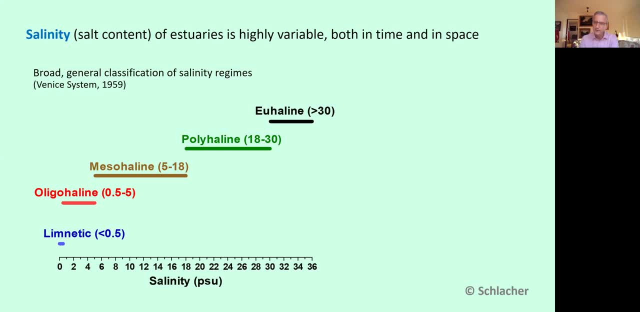 a little bit of salt in freshwater because it leaches continually salt out of the earth and off the rocks it comes from. But that's okay, you know. So basically you get 0.5 grams of salt from a lake. 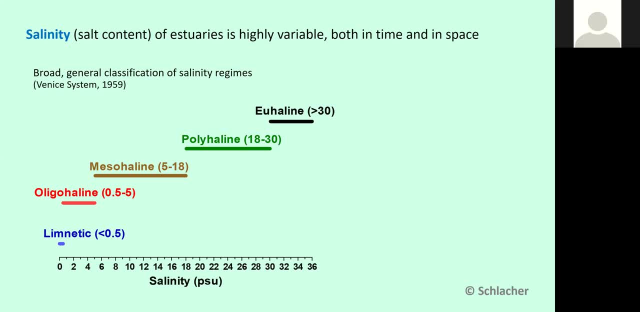 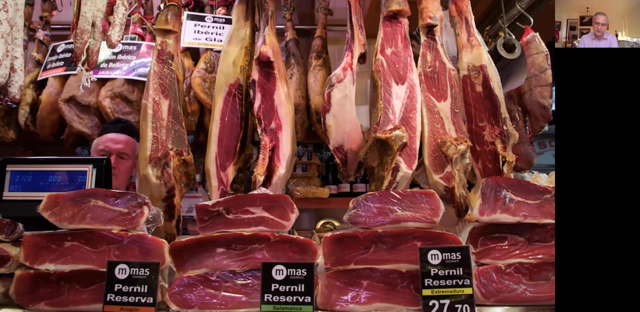 From a liter of freshwater And you get 35 grams. So it's basically 10 times, 500 times more, So you can. So, for those of you who are vegetarians, this is sort of a typical picture which you get in a Spanish market. And there's all these hams And we are going. 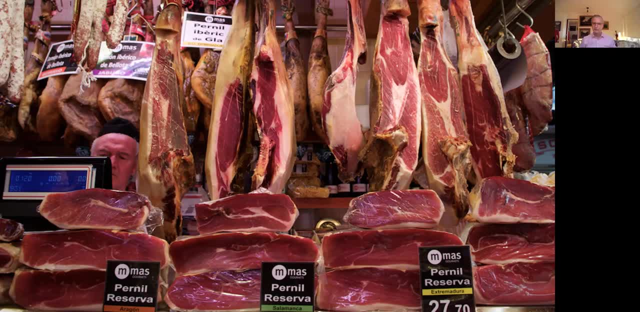 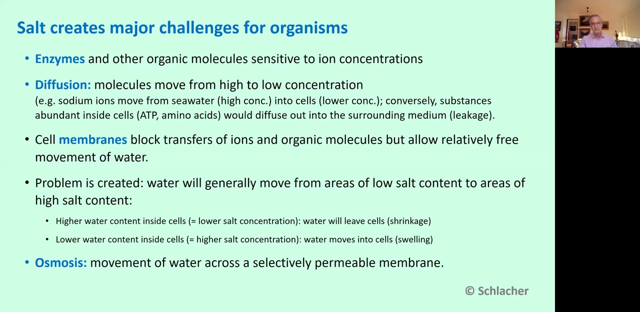 back to the person who was preserved in a salt mine, and the beak and the fish and the pickle vegetables, Because salt is an excellent preservative. Why is that? Because what it basically does is a number of things. The first one is many enzymes and other organic 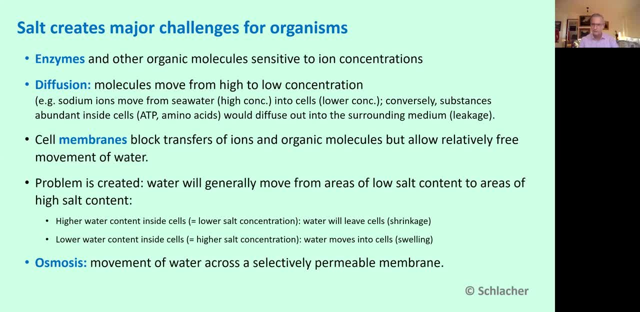 molecules, particularly proteins, are very sensitive to changes in the iron concentrations. To put it basically down to the most basic principles: If you put something in a brine solution or rub it in salt- and this is a you know, you can also make- it's quite actually funny. I should actually tell you that We used to make our own bacon on the farm, you know. But you can also make prosciutto If you go, you know, do an Italian providor, as they call it nowadays in Brisbane. Prosciutto costs about 40, or 50, or 70 dollars a kilogram And you can make it in the same way that you. 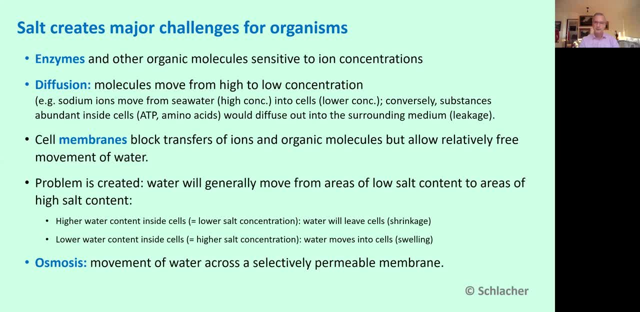 can make it in a brine solution. So what you need to do basically in the winter here is get a good leg of pork and rub it in salt like crazy And then you hang it in a dry place. that's why I have to do it here in winter and let it dry And that's. 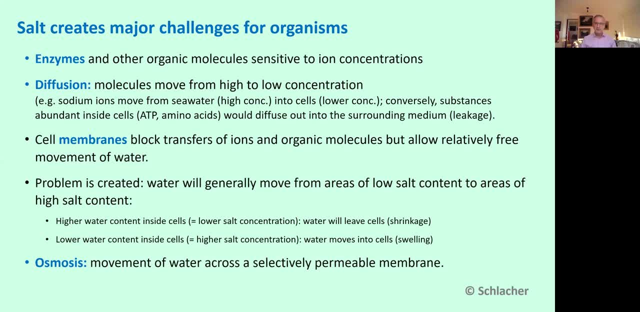 all you need to do. And why does it actually work so well? Because salt essentially kills the bacteria protein, But it also makes the protein in the ham denaturalized. Now you know it's not a good thing to do. Now why does that actually work? It works because 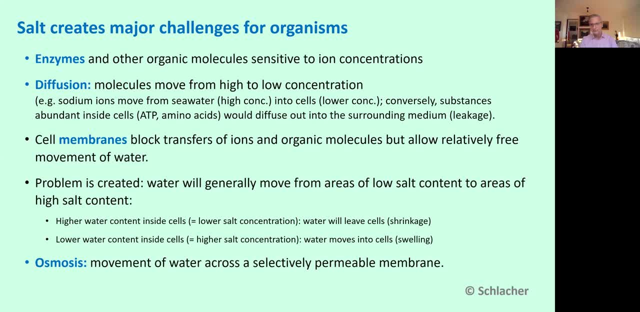 nature tries to be nice to everybody. So what it basically does is, if you have a difference in salt concentration, liquid like water will move to smooth out that difference. So if I would actually have two different, oh, here we got salt and here we got water. So 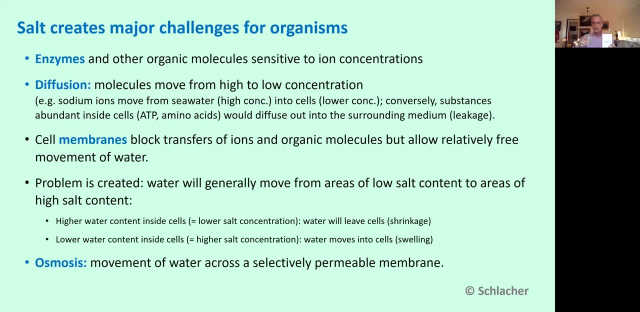 what would actually happen is if I would actually have two different. oh, here we got salt and here we got water. So what would actually happen is if I would actually have two different. if there would be a connection here, like a cell membrane water, this water here would 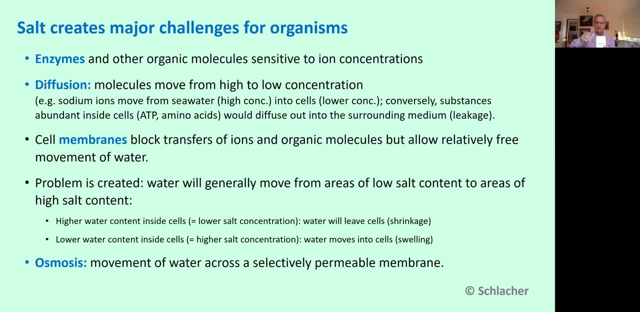 rush like crazy into the salt packet, because the aim is of natural systems, that the concentrations even out, And what actually then happens is if I take salt And, let's say, I have my skin here, This is all actually, you know, mirrored. So it's actually quite funny if you think. 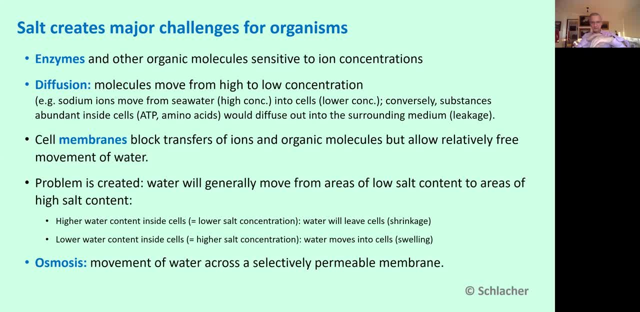 actually quite funny, if you think my movements are funny, and i would actually rub this in continually. and let's say, i sleep in a salt crust overnight. uh, basically, water would actually rush out from my body like crazy, trying to get the salt concentration the same as it is inside the body. so 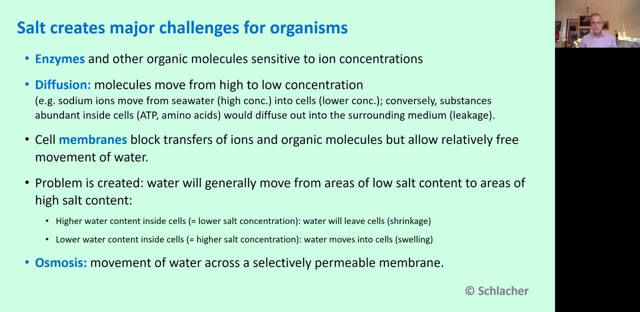 i would actually lose water like mad. if you basically submerge yourself into in the sea, this is exactly what would happen. all the water will be gone after a while and that means that, essentially, the bacteria can't actually live anymore. the proteins are all crumbled up and you 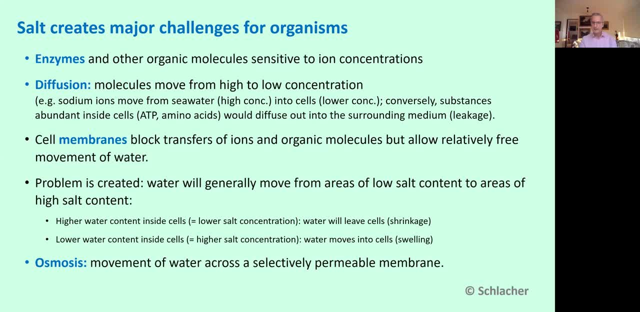 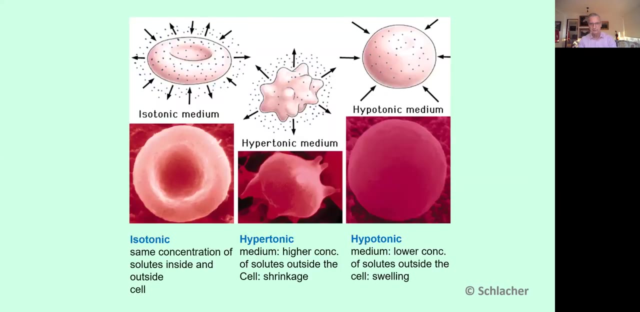 essentially die and bacon works and pickled fish works and picking vegetables work because the proteins have been completely crumbled up and the bacteria die because they explode, because all the water, basically, is sucked from their bodies. so everybody actually has seen this. 100, you know 50. 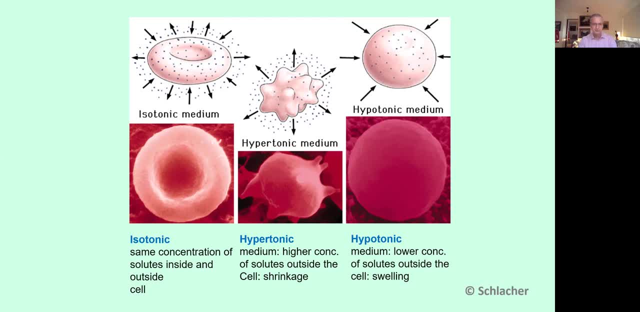 times in biology about osmosis and so forth. so if you have an isotonic medium- this is why i try to sell you these sports drinks you know, which is, of course, complete rubbish really, but never mind, people make money. but let's say you drink, you know sea water when you go into a hypertonic medium. 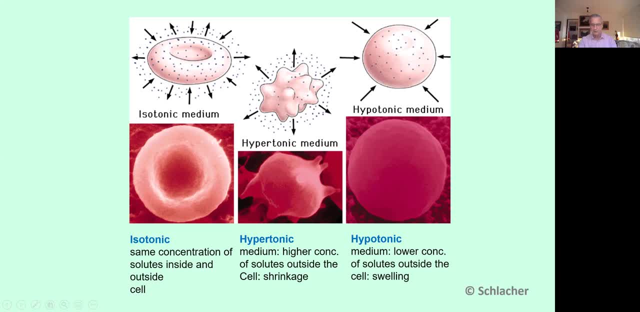 essentially, water will actually go out from your body because it seeks to, you know, equalize that difference and the cells will actually shrink. if you lie for a very, very long time in the swimming pool or in a lake, you will eventually explode because water will just rush. 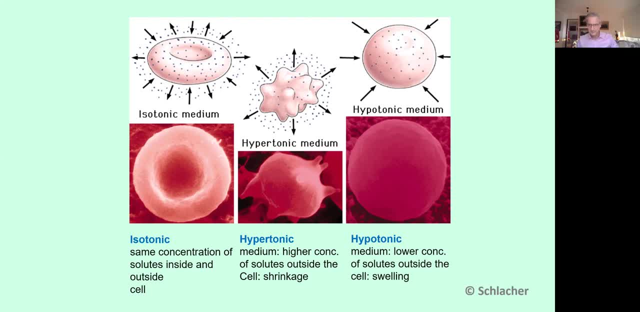 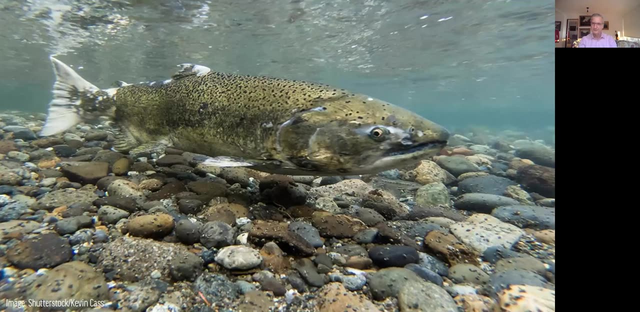 into your body and make you pop. uh, why is that? because the salt concentration in your body is higher than outside. why i'm telling you that? now imagine, uh, you are a salmon, is a nice looking salmon, and someone have a very, very hard time because they have to go between the fresh water and the sea, between the fresh water and 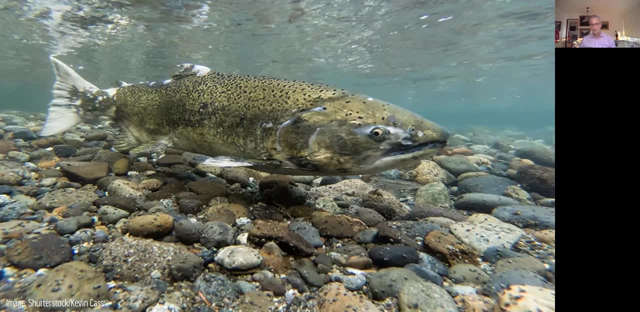 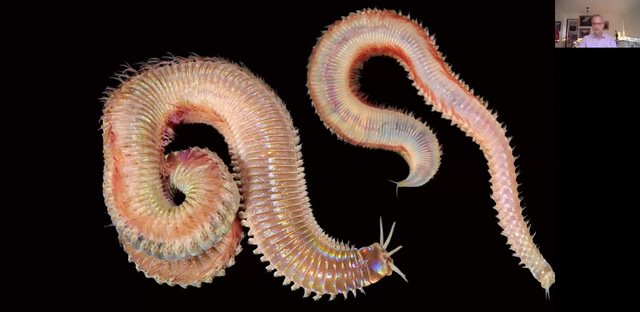 the sea and so forth. so do yields. remember what we talked about last time about migrations. now that actually exposes you to a very, very- you know- big range of- uh, basically- concentrations. what happens is that you're not going to die even if you don't make any changes. 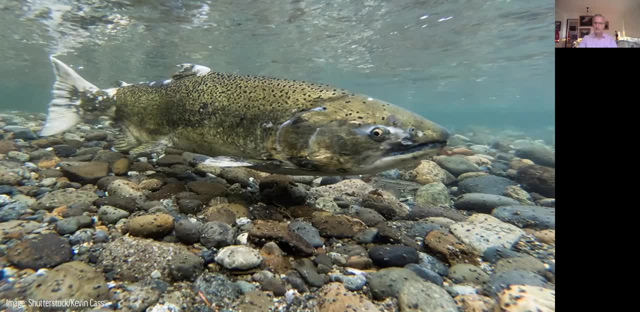 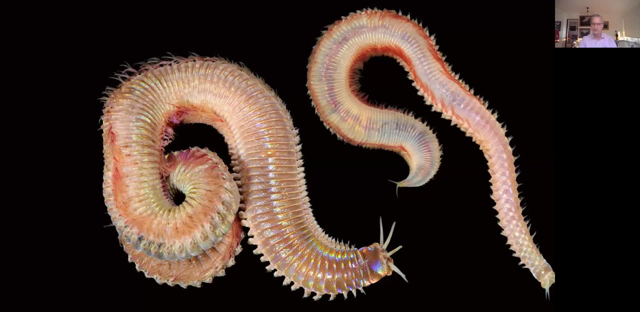 uh, and you're pretty much gonna be back to the same level of fitness and eventually you're going to live with it. and that's why, you know, it's always important to say: my life is on the line. i'm not going to die now, you know, because i don't want to die now and i'm going to live with it because 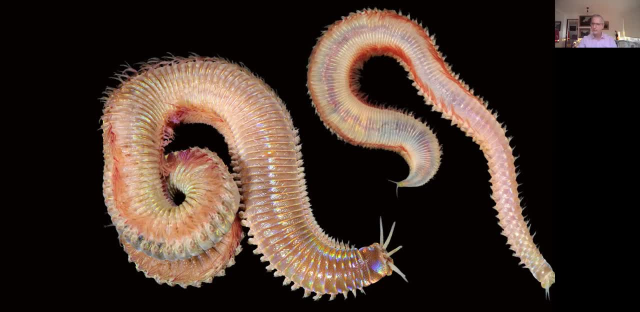 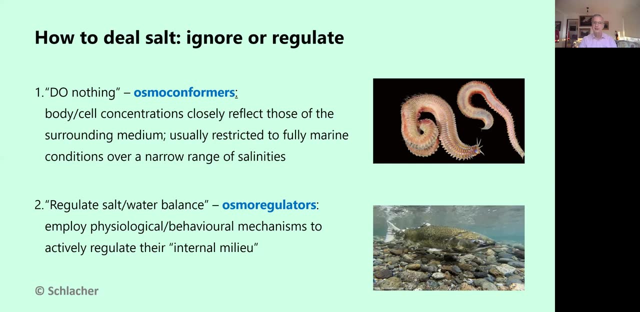 i don't want to die until the end. i'm going to live with it and then i'm going to never live again. but you look at rocketeering. you know the difference between salt concentration and big salt concentration and big salt concentration is that balance between salt concentration and big salt. 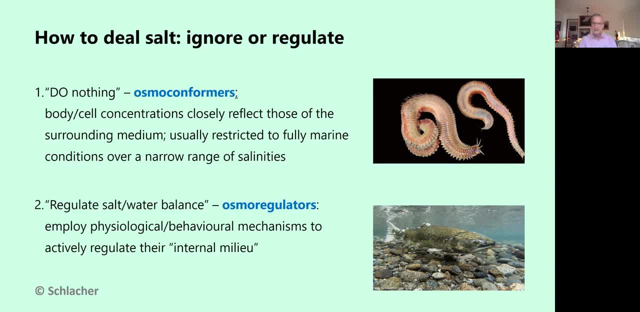 the first one is like the worm. here you do basically nothing, you just conform to what your environment is, or you basically regulate the ion concentration in your body, and this is what most organisms do. now this is actually quite a tricky process, and we actually go through that in a 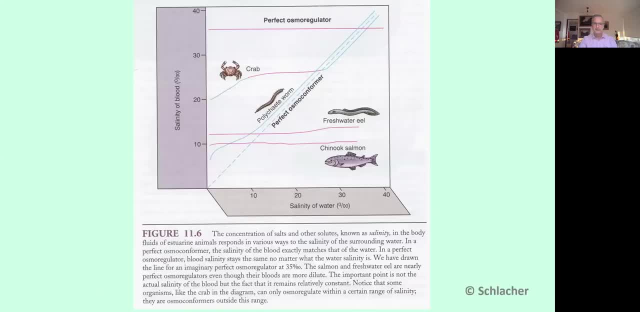 little bit more detail in a jiffy. now you get those kind of you know diagrams in every single textbook. here is basically a perfect osmo regulator. no matter what the change in the salinity of the water is, their internal concentration will always be the same. 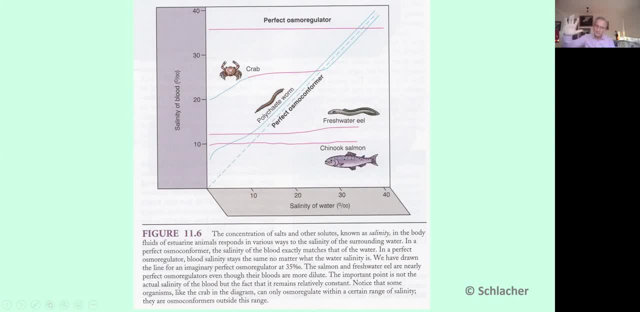 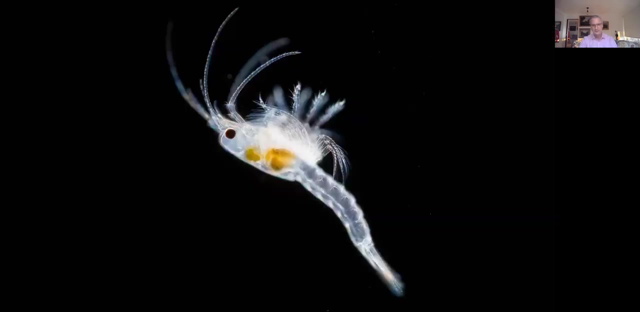 or a body hit worm or a crab might actually, you know, just basically go with the flow, so to speak, so their body concentration will mimic over time what's happening outside, which is physiologically very, very challenging. now most species, or most invertebrates, do a little bit in a of a compromise, and i do know that here is anybody knows what kind of 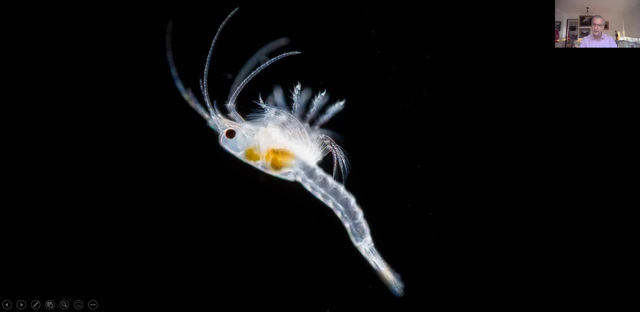 weird looking animal that is. i'll give you a hint. we talked about it. it has the balance organs, like the stones, so to speak, which we have in our semicircular canals in the ear. they have them in the tail fan. what kind of animals that is? and 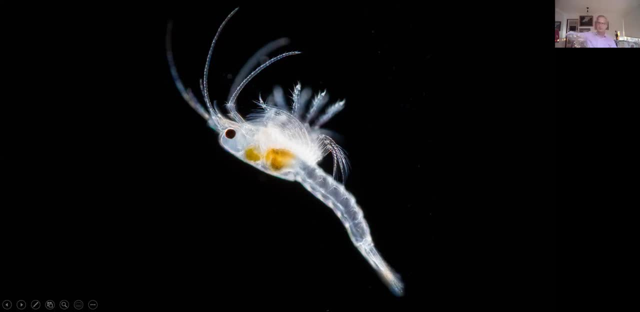 remember i told you they actually use that to actually swim upright and the stones, so to speak, they uh preserve in the paleontological record to have whole layers in shallow seas and they have a brood boat. so they bear life young and they're the main sea. uh, they're the 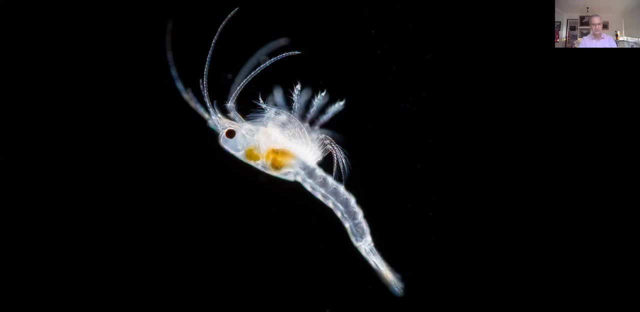 main prey item of leafy sea dragons. any idea? is it a lobster? no, it's not a lobster, it's a mysid, an opossum shrimp, because they got a bruise pouch here now, well, you know, i always say, you know, you should never actually, you know, believe people who actually, yeah, actually, if they. 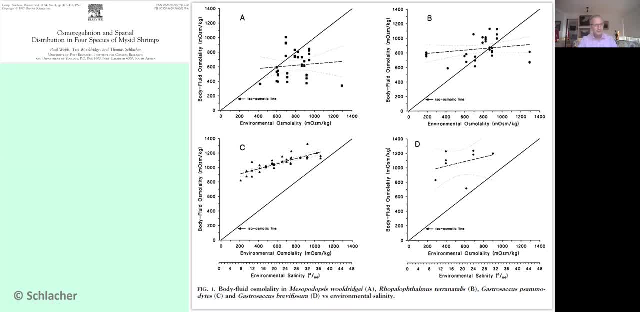 actually haven't done it. you know yourself. so this is what we did quite a few years ago. but basically, you know, i caught a lot of mysids and i caught them from different parts of an estuary going in, you know, salinity from almost like a. 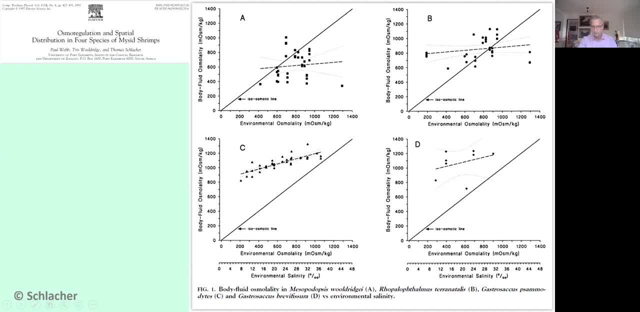 zero to about, you know, 40. this was basically because one of the estuaries closed down and we have different species here and you can actually see each species has a slight different strategy, but by and large they osmoregulate to a certain degree and then they 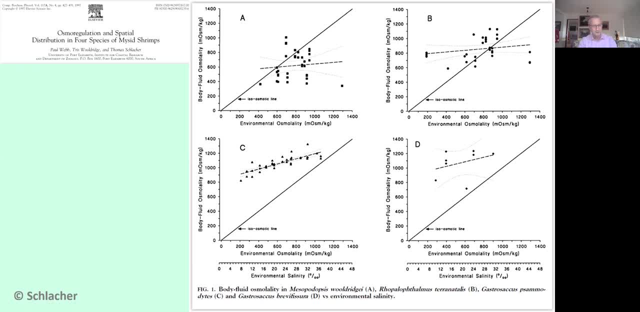 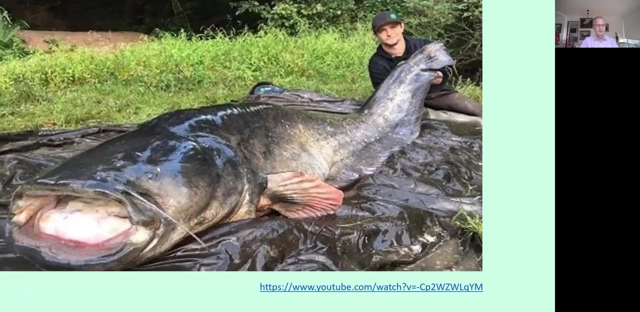 start to conform. so it's actually a very, very complicated process. uh, and again, it just goes to show you actually think like: oh, i'm a, i'm a biologist, but sometimes you also become a physiologist. but osmogulation is a difficult business for estuarine organisms. now let's look at two different fish. 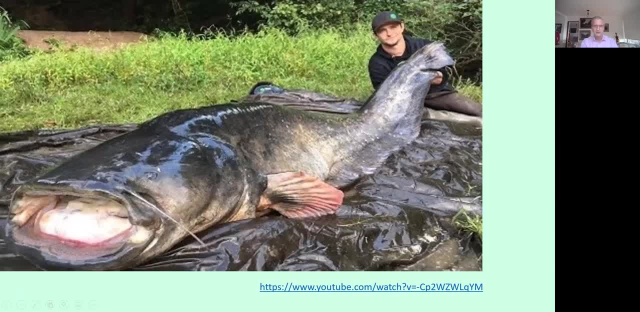 species. now this is a rather, you know, big catfish. I think this was the world record. I shouldn't probably tell you, but they used to be a practice that you fished for catfish with you know smaller ducklings, because this is what they actually prey on. they're actually very big fish. they come up from. 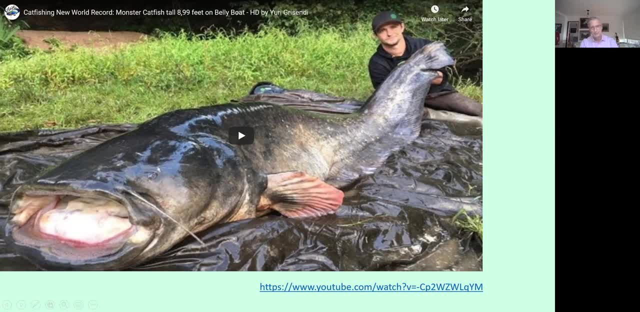 underneath and snap the ducks from the top, but also little dogs were actually used. so it's quite quite a bit really. you know, little Dachshund and they swim out, and catfish came from underneath and they're like, actually got them. now, if you are a freshwater fish like this fellow here, you know, or something more. 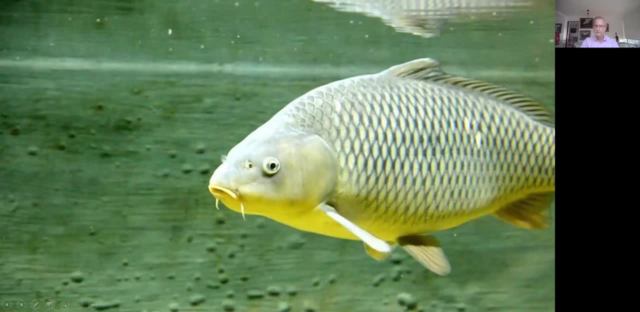 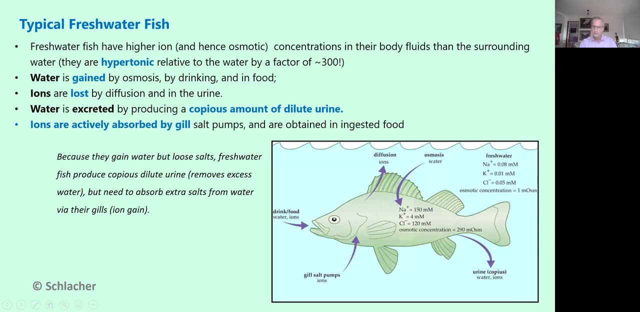 benign, such as catfish. I don't know what you could do about it. I'm sure I could. a carp life is very, very complicated because, as i told you, if you would actually lie in fresh water for a long time, they would explode. why would they explode? look at the concentration of the different. 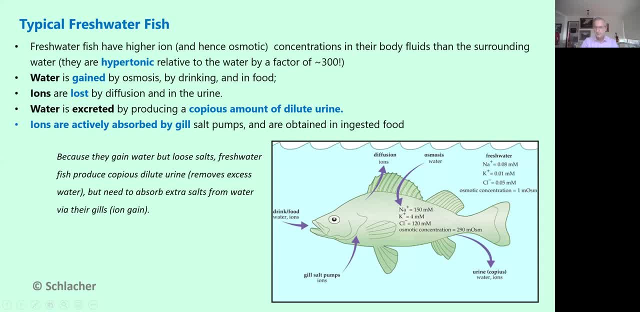 ions here inside the fish, and then you look at the concentrations of the iron outside, here in the fresh water. so essentially, a fish in fresh water is just a parcel of salt, so to speak. and what actually happens? naturally they gain water. water just rushes in through the permeable body. 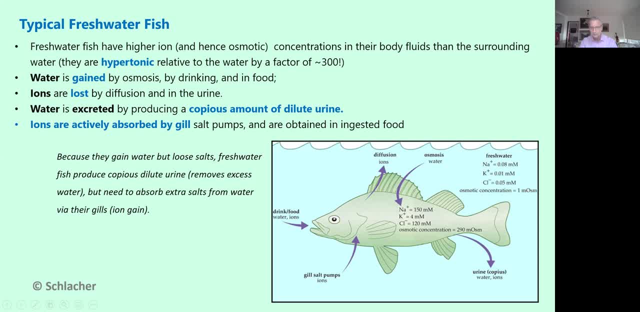 surfaces, which is often through the gills and also through the skin. now that basically means you gain a lot of water and you need to get rid of that. which basically means: um, i have always been told, don't drink water, drink beer, because fish basically make loving water. but it's actually much worse, you know, if you drink enough water from. 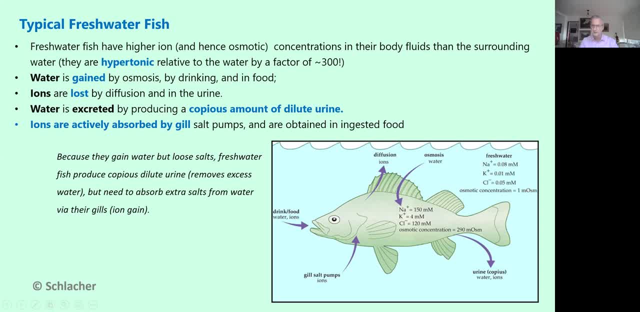 you know, a pond or a lake fish really pissing it in huge amounts. essentially they have to get rid of the water which rushes inside their bodies, but it also means they don't want to lose valuable sort molecules. so what they do is they actively absorb salt which is actually lost, and they have salt pumps in the gills to suck salt from the water. 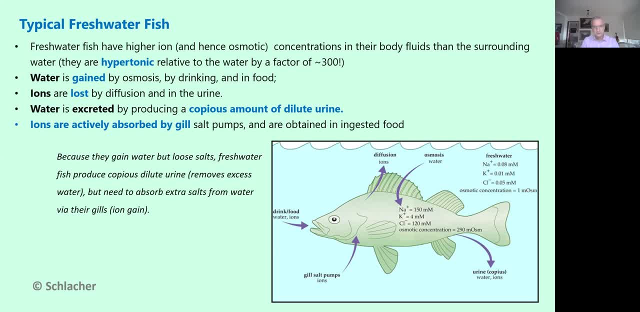 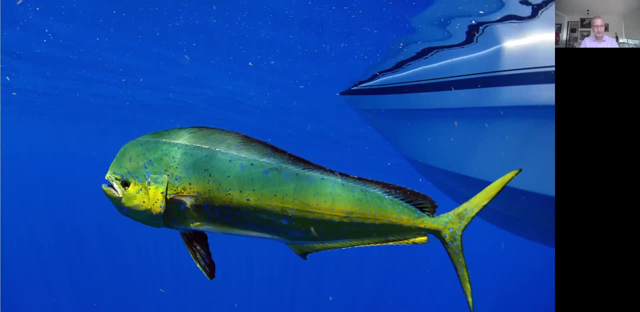 inside the bodies now. so this is, of course, you know, a strategy where you absorb salt and you get rid of the water. now, if you're a marine fish like this, maybe you won't be still in the pH through and the enjoyed. you are doing the very good job. 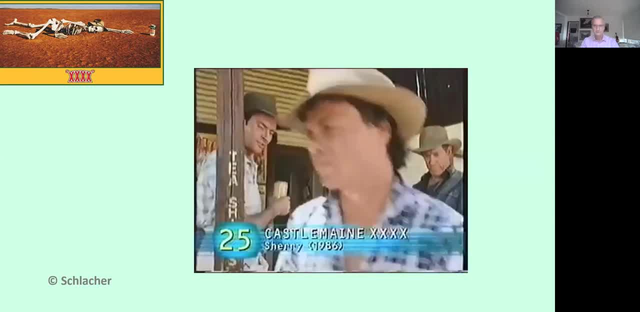 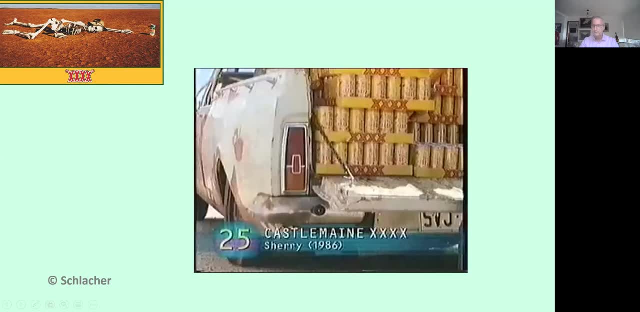 but, and just imagine, you face each one of these very low lots out there and if it's raining light, the fish. fish won't cloudy, the fish may not be. jelly boy cannot just getrolled out. you're just like the balary girl just being by. so maybe some of you have an audience in the past. 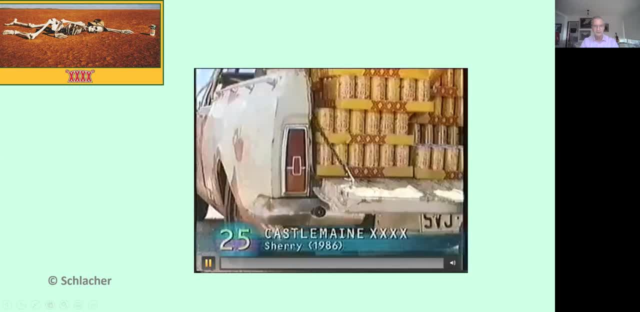 which I'll ask you that that's fine with you. but if you could adding in someegal, and certainly, but sometimes you can, but in the very courses like there can. if you can't, then how? just to get a lot of water? it's very different. so a marine fish will not have the problem of exploding because it has too much water, like a carp. it has a different problem like this plate here, just politically. 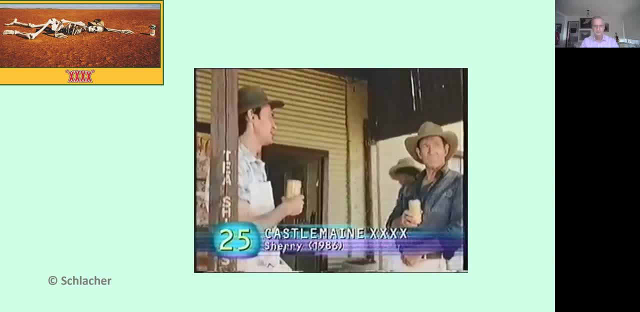 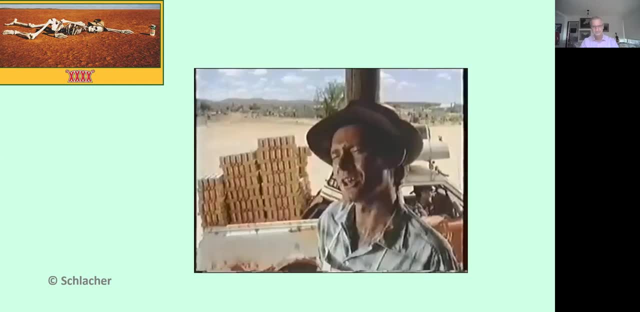 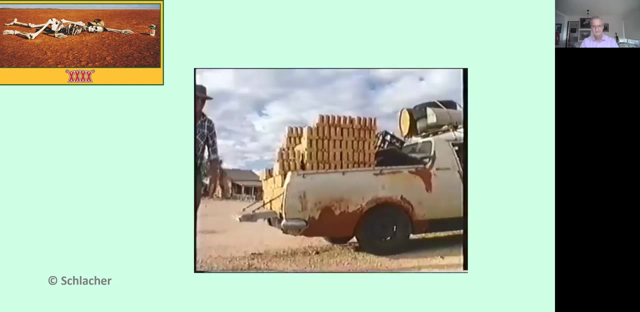 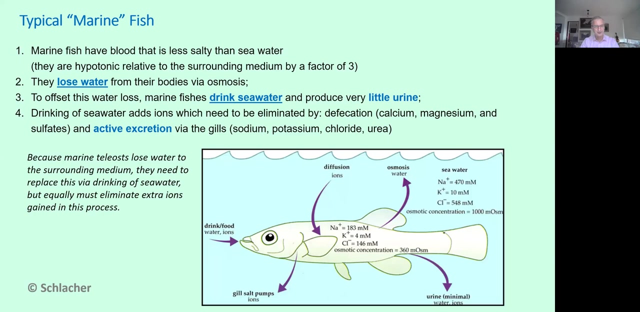 a few of you out here on this time about 40, i reckon. something for the ladies. oh yeah, sweet cherry, australians wouldn't give a castle name forex. so here you go. how is that for a politically incorrect ad? but you know, it's fantastic, what it actually. you know why i actually put it in. 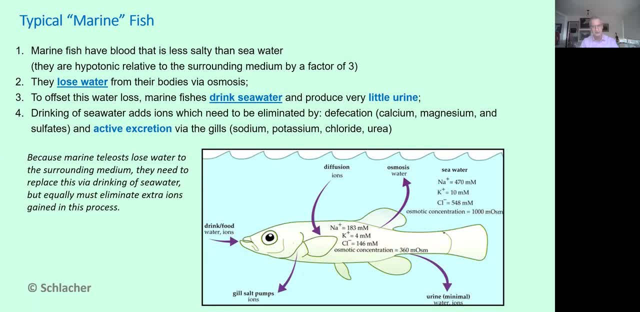 is that, as a marine fish, you're usually very, very thirsty, because what actually happens is you again look at the concentration of the ions in the seawater and you look at the concentration inside the body, you can actually see that they are swimming in a very salty environment. 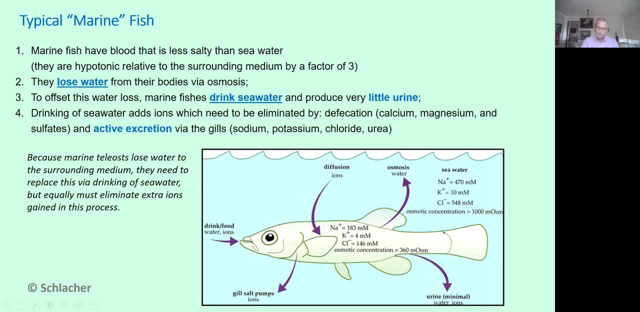 now, if you have excess water inside the fish, okay, then it tries to rush out. in a sense, the fish dries, or the exchange of water dries to make the sea less salty. of course, some kind of work, but never mind, here's the principle behind it, and so, essentially, they lose a lot of water. 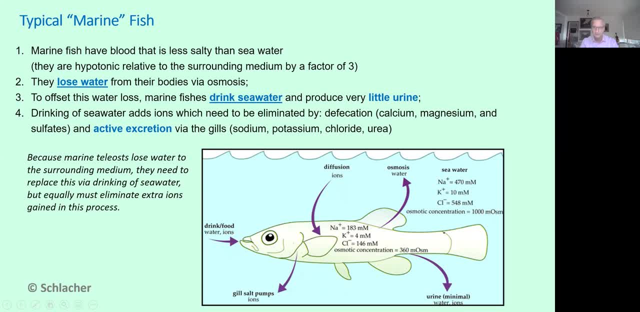 but they don't actually have any here because they don't actually lose any more. it's just like those guys you know in the in the forex head. but what they try to do- and this is actually very interesting- is they shrink a lot of salt water and then they have to get rid of the extra ions they actually take up. 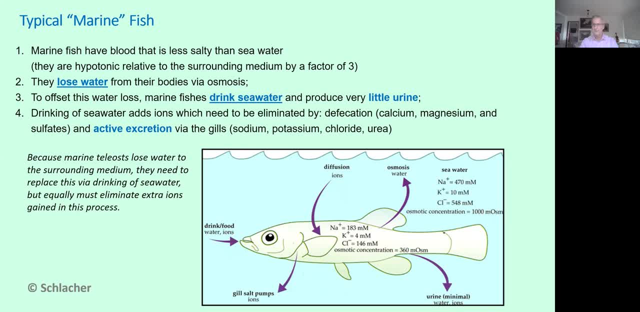 via the gills, and this is actually a trick. we die of drinking in a too much salt water when you are in a life raft because we don't have any specialized organ to get rid of salt. now, if you have done physiology, you would have also seen that in our days special 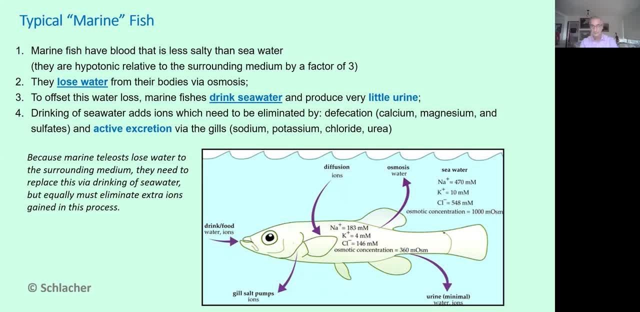 organs in reptiles. that's why people say, oh, a turtle actually cries because tears. no, they don't have tears. they're actually trying to get rid of salt by a special salt clouds, you know, on the head and so forth. so a very, very tricky proposition, uh, to be, you know, a fish in different salinity. 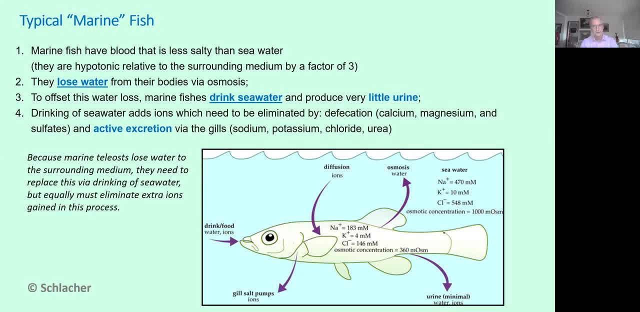 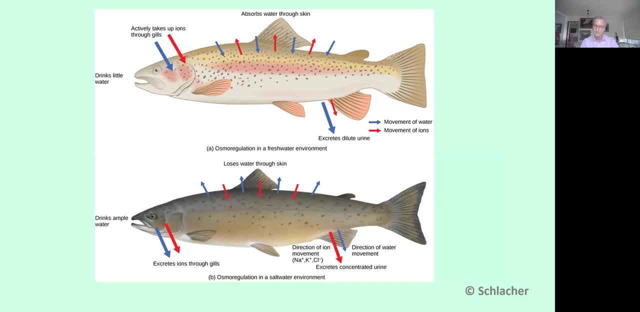 environments and that's why, basically, estuarine of estuaries are very challenging places to live. so here's another basically display item showing you the same thing: freshwater fish, basically huge amounts of- you know- urine, because the water rushes in and it takes up ions to the gill. 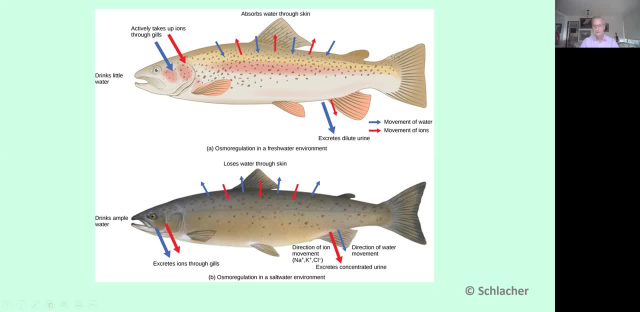 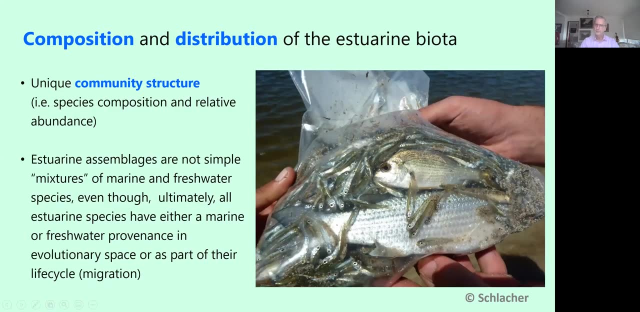 where some marine fish, such as this salmon here, that's exactly the opposite. now you might say, right, if I study estuarine biota, such as this catch here from you know, and that you see a lot of, uh, they look like hardy heads, juvenile ones. here's a brain, here's a mother. you might say, well, you know an estuary. 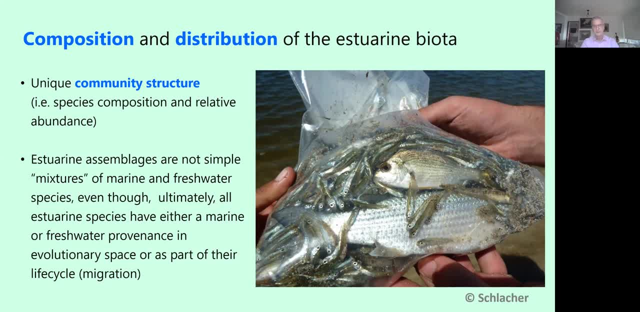 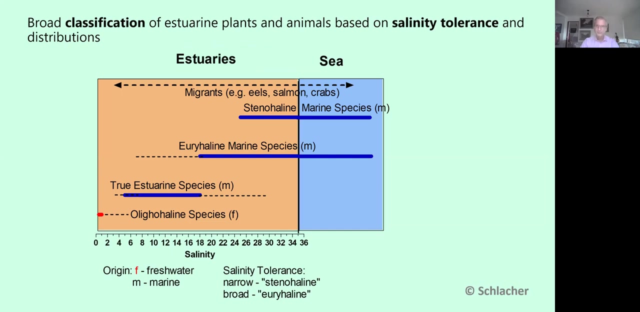 is just basically a mix of a few marine species and a few freshwater species who can actually take those different concentrations of salinity. so there's nothing special about them. it's actually not quite true, because estuaries have a very, very unique species composition for the simple reason that some species- yes, they- come from the sea, some species come from a freshwater. 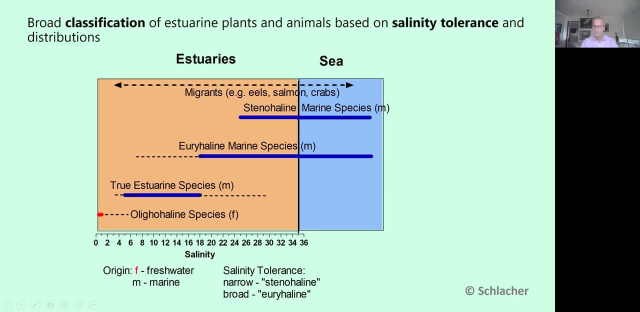 environment. but there is actually a component of true estuarine species which you normally don't find in large concentrations in the sea or out in uh or up in the freshwater deficiencies, like others, and we can't always determine easily. the Tyrannosaurus吧. information of the sea is a calm in everyone's there in the and people in our world communicate the same thing, but an estuarine dead fish which is different and haven't eaten them in many other species, such as mullet seabass, species sometimes called wandering fish and 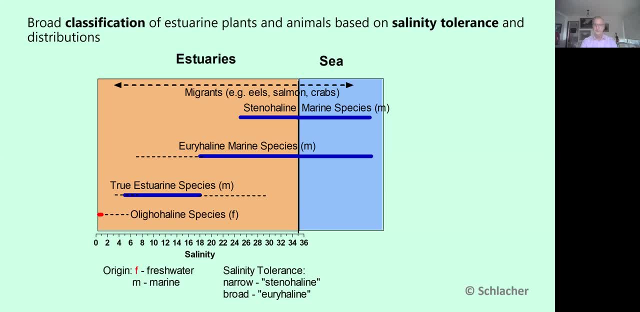 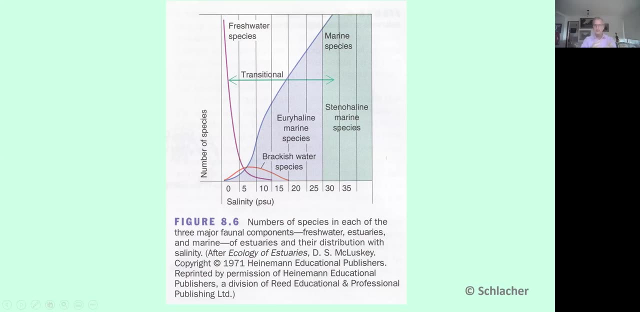 or up into freshwater species. So there is a component of what we could actually call a true estuarine fauna. Now, this is one of those classic diagrams which you actually basically see: Freshwater species, as the salinity goes up, go down, then a few brackish. 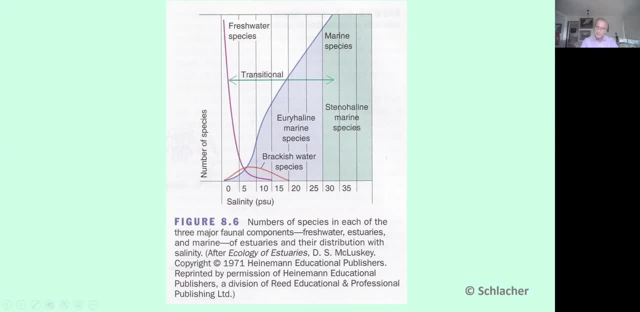 water. ones actually exist there, and many marine species penetrate to a certain degree, but not quite, into freshwater reaches. There are, of course, species such as bronze whale, sharks like the Zambeziwines eels, many of the salmonid species, including trout and eels, which can actually 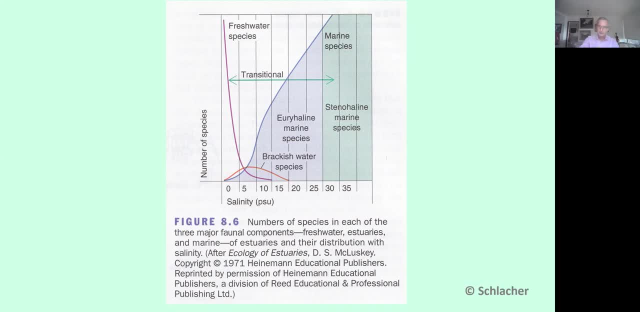 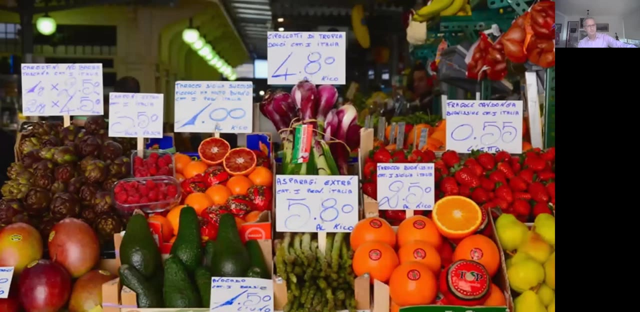 do that, But usually there's a limit to marine species going up, there's a limit to estuarine species going down, and the bulk of the fauna is then actually made up by true estuarine specialists. Right here is a vegetable market in Italy, and it looks fantastic. 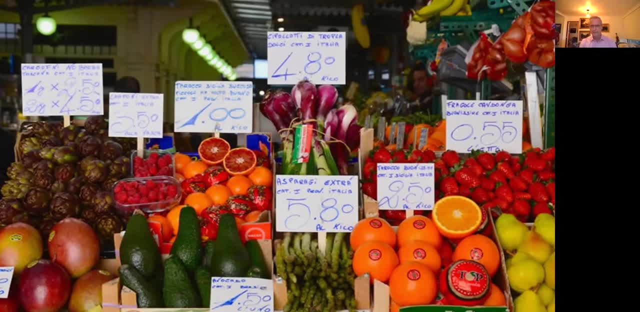 And it looks absolutely fantastic. So what we actually have here is a great diversity, And, as humans, we are drawn to diversity. We like diverse stuff, right, We like to have different things, And we also are drawn to biodiversity. Now, this could be a vegetable. 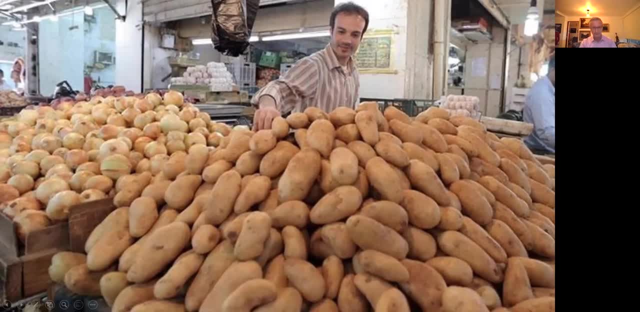 market in Ireland. You know it's got potatoes and it's got onions And we instinctively almost said this is likely not that good, It's actually not very diverse. So diverse, not diverse. And then you can say: But if I go to estuaries, are they generally speaking? because they're so important, they all live on an estuary somehow. are they, generally speaking, diverse or not? 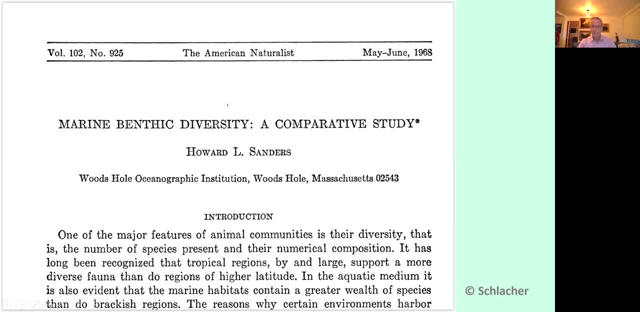 Well, here is a very famous paper which I just, you know, copied the first page and basically how it centers- you know, I mean the data are not terribly convincing- behind it, but basically said: well, yeah, where do you find the most species? 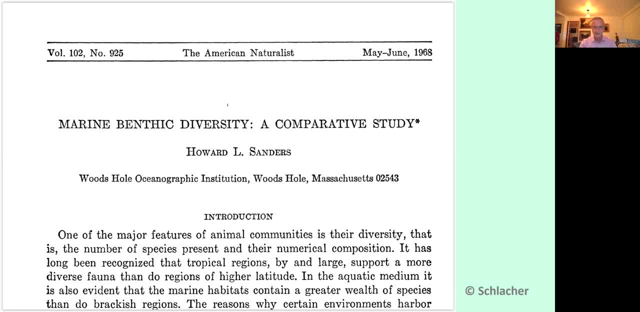 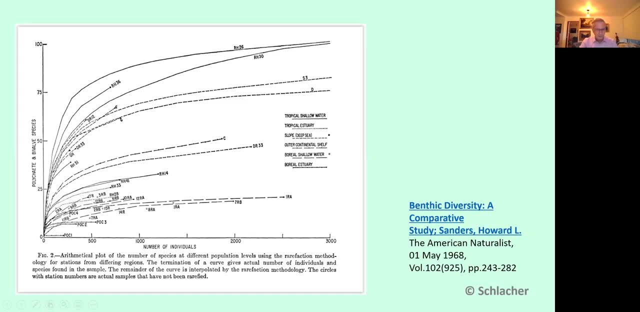 Is it a coral reef? Is it an estuary? Is it the deep sea? And actually, as it turns out to be the case, this is a horrible looking diagram. So what you actually do is you say: oh, if I catch a thousand individuals, how many species do I get on average? 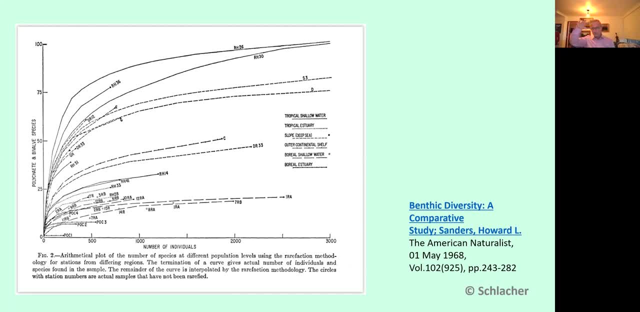 How it actually works is the more individuals you catch, the bigger your sample, the more different types of species you usually have in it And it blatters out at a certain extent. It's called a collector's curve. Originally it comes from people going across the English countryside and they say, oh, I've got 500 beetles and there are like 50 species. 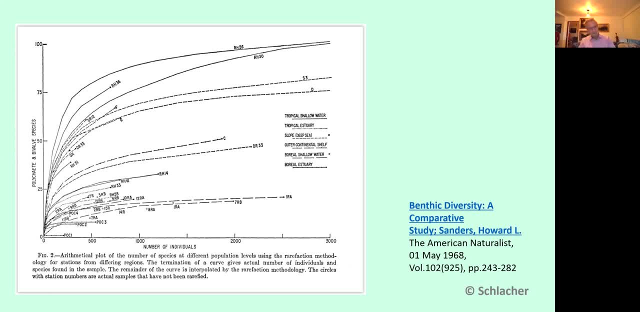 Oh, a truly good old chap. and you know I said, oh, I've got a thousand, or I've got 80 species, and so forth. People still do that. you know beauty collecting. don't ask me why. 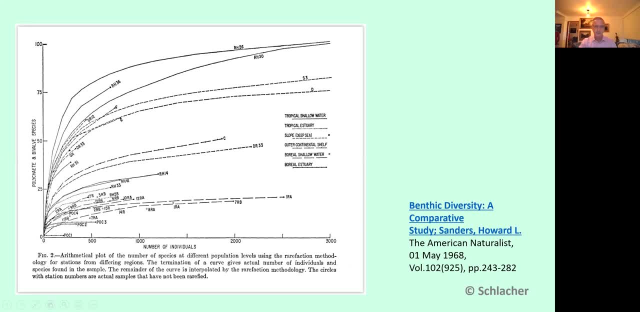 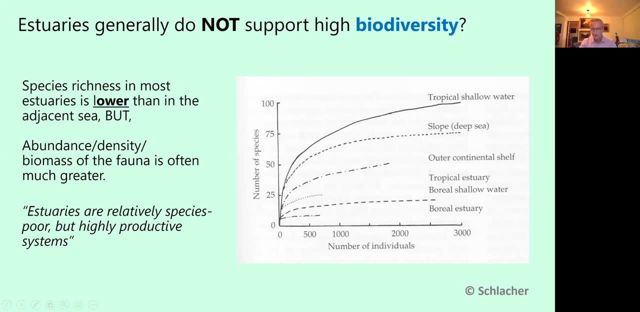 And essentially all the estuaries sit at the bottom here. So this is a bit of a cleaned up version from a textbook, and you can actually see here the coral estuary and this is topically shallow water, And also the deep sea. The deep sea is actually amazingly biodiverse, often much more so than coral reefs, and you know, I might tell you a little bit about that in about two weeks' time. 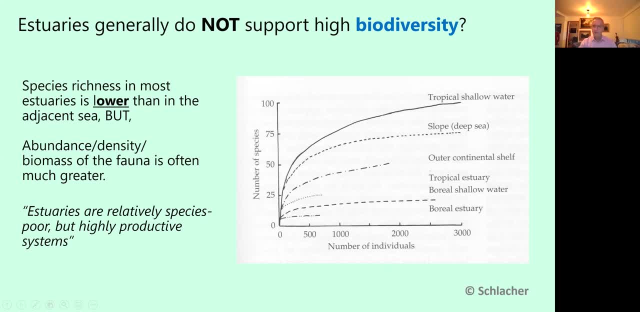 So, essentially, if you- I always say, if you're after studying highly biodiverse systems, either go into the deep sea or go to a coral reef. Don't go into estuaries. You're not going to find terribly many different species. 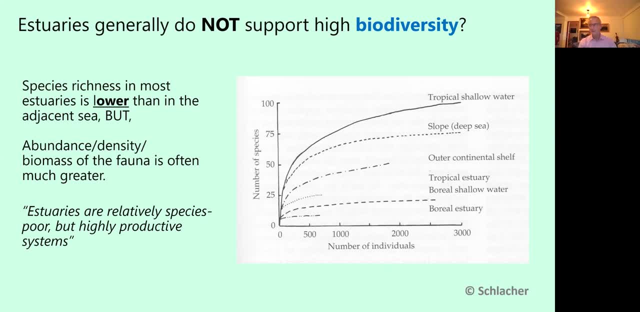 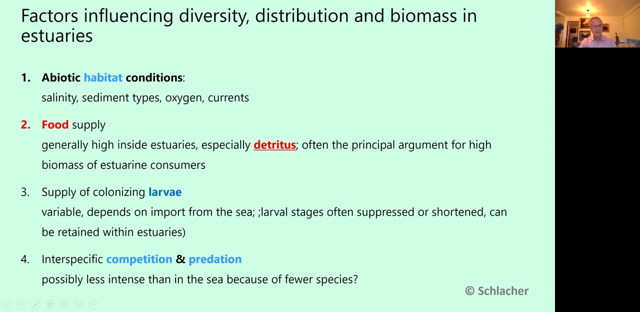 For the reasons we have just explored, because it is reasonably difficult to actually live there because of changing salinity, muds and so forth. So essentially the abiotic habitat conditions, like salinity, changes, different sediment types, sometimes oxygen is low and you're in deeper layers of the estuaries. the currents displaced here are kind of inimical. 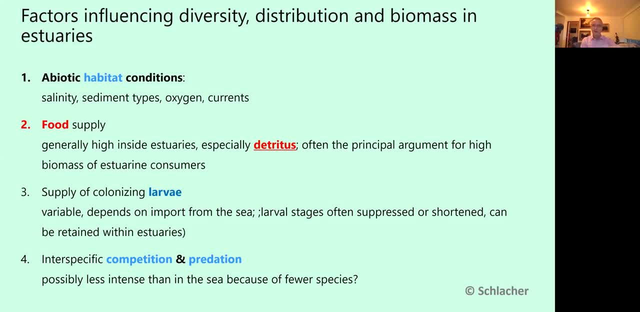 However- and this is going to be the rest of our lecture today and the lecture next week- food supply is high. estuaries are rich in food, and most of it actually comes in the form of detritus, bits and pieces of plants, but also animal carrion. you also often have quite a bit of larvae there. 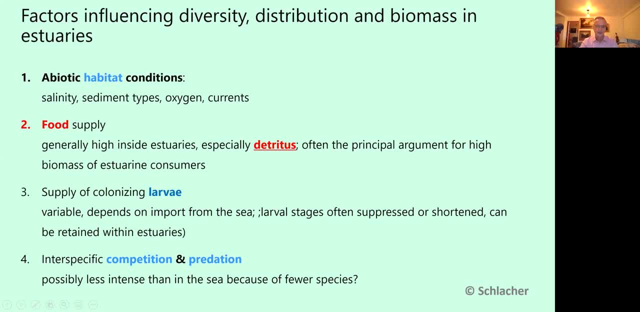 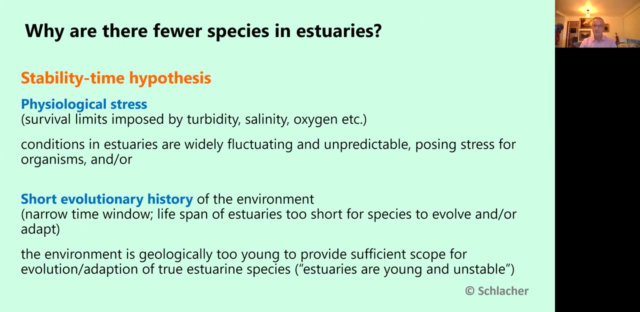 because they get retained inside the system and we have competition reputation. but you know we you're not actually going and discuss this at the moment. I just put it there to be complete. so you might actually say- and I just put it in because it's always interesting to come up with- you know big. 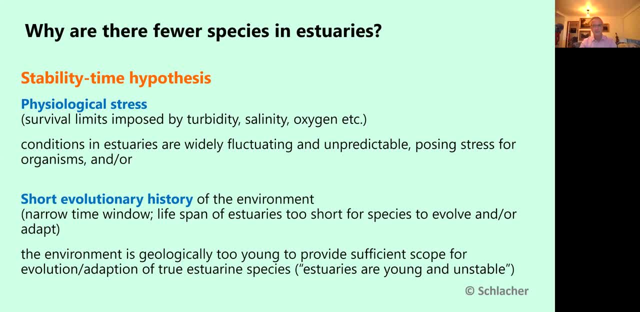 hypothesis you might say, ooh, why are there so many- you know so few species in estuaries. you can say, well, what we just discussed. think about the man trapped in a salt mine and his body's. like you know, it's actually quite funny on a camera. 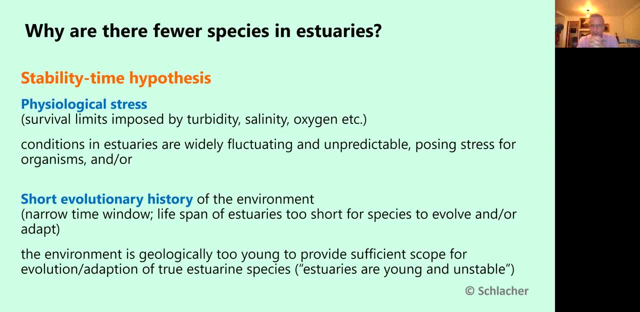 you know, essentially, you get preserved over centuries- bacon, vegetables, and so of course it's a challenging place to live. or another theory says: well, you know, essentially it's a short evolutionary history. those habitats are usually very, very young. why are they young? because many estuaries are created by the sea. 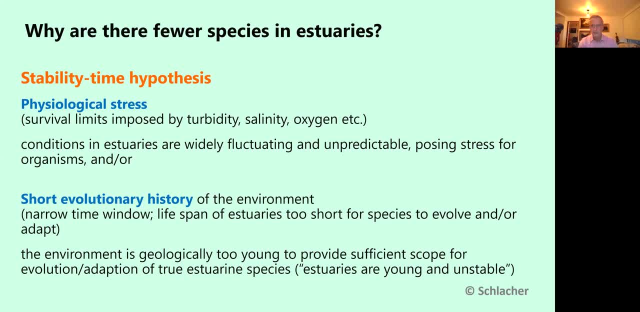 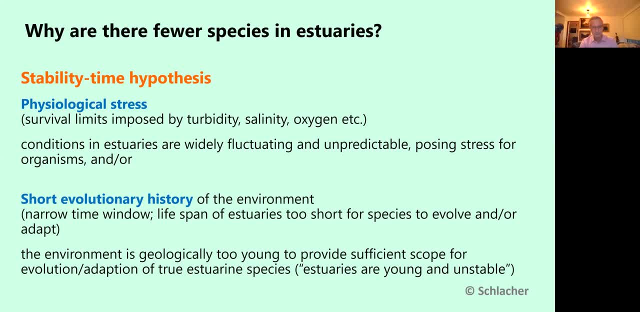 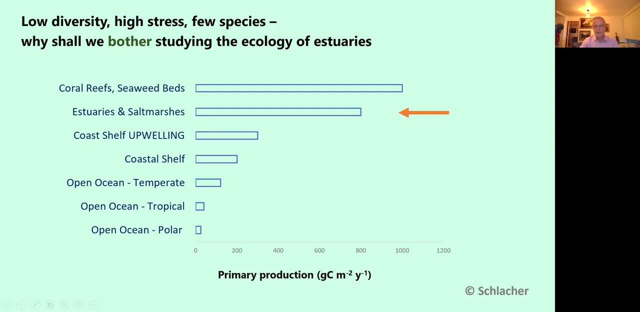 estuaries are, evolutionary speaking, and geologically speaking, very young, so maybe there wasn't enough time. who knows, it's interesting to actually muse about that. so you might say: well, low diversity, high stress, few species. why do I want to actually study estuaries? why bother about them? well, for the reasons we just said. we. 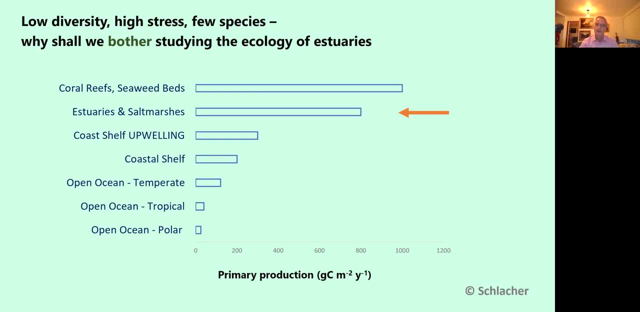 all live on estuaries, so we actually try to look after them, but also because they are very, very productive and if you actually look at the most, this is a kelp bed and this is a coral reef. I think this really is a little bit too high. so I put those values together. 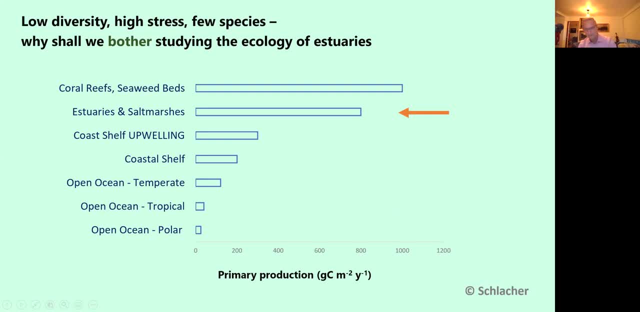 here. you know from various literature sources that's my own kind of doing, but what you basically find is is that estuaries are amongst the most productive ecosystems on earth. they are more productive, they're topical rainforests and even some of the most intensive agriculture, with lots. 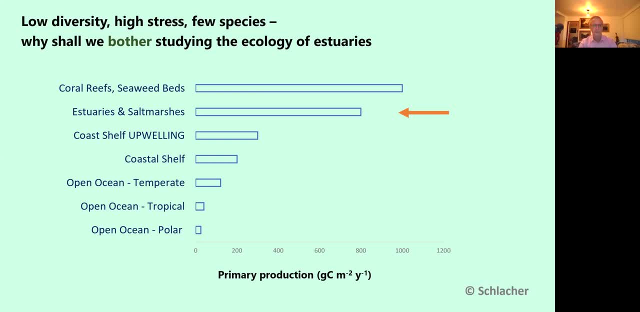 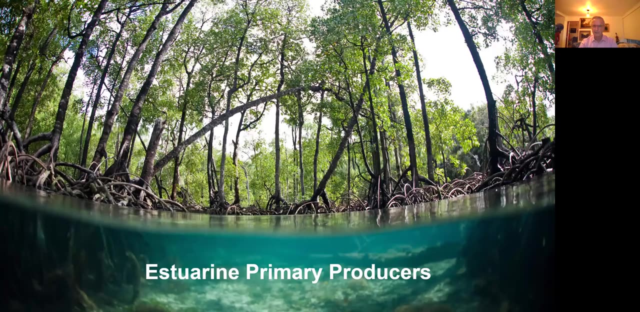 of fertilizers and very well managed corporate cooperation is often, you know, not as productive. now you might say that's a bit. you know, I didn't know that. why are estuaries so productive? the reason is we have to go into botany and I, you know, I I very deeply apologize for having to talk about you know. 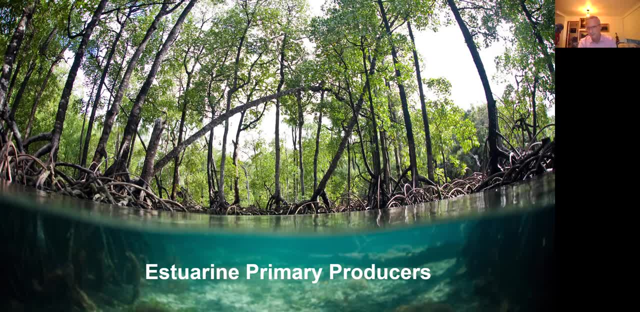 the next. you know 40 minutes or so about botany. I know it's a. it's the lesser one of the sciences. I grew up in a botanic garden. maybe there is a botanist, so I know all about it. but essentially what you're going to try and do is we're talking about. you know, the food supply of animals. 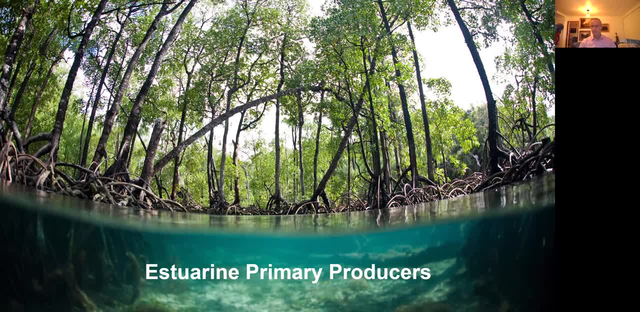 and estuaries really have one huge advantage because they're too large and they're too geologically or geomorphologically so diverse because they go from fresh water to the sea, you can pack just about every singular plant type which makes carbon into it. that's fantastic. 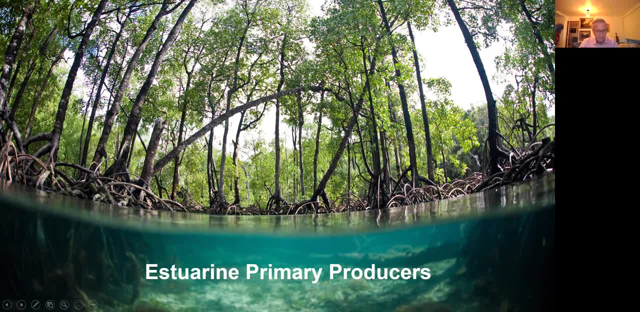 and look at this great picture. remember that when we talk about mangroves, there's all these roots. the fish can actually hide in there. the leaves actually fall in there. there will be benthic microalgae on the roots here. there will be phytoplankton in the water. it's really 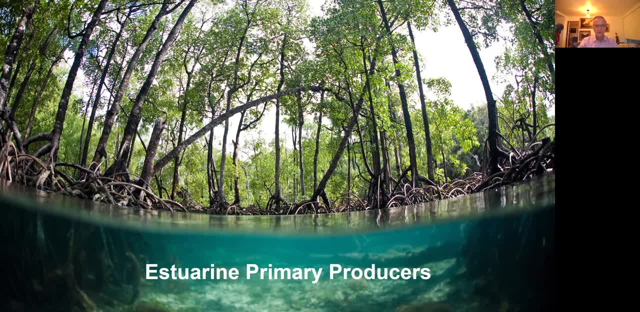 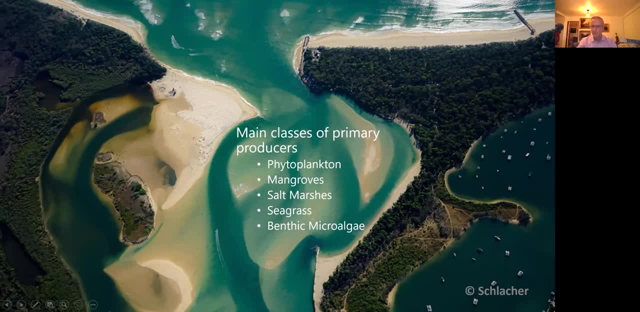 a bonanza. it's really, really a bonanza. So thank you very much. Thank you. So, yeah, isn't it a nice picture here? so it's actually. if you talk about primary producers, things which make carbon, this is Mnusa again. yeah, so this is, this is the beach and this. 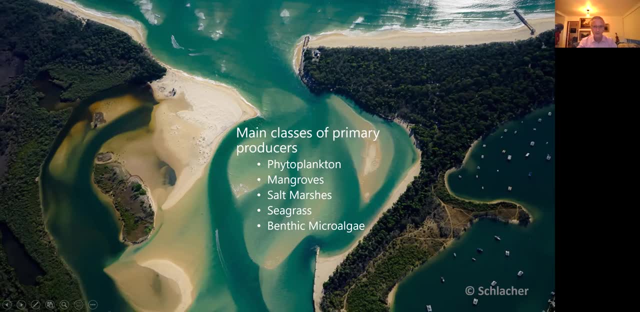 is the middle groin and it basically goes up into the estuary here. everything is in there. you know, we have this big mangrove forest here. fantastic isn't it? there will be phytoplankton in the water. There is seagrass A little bit further up. there is actually seagrass along here. we can't really see it. 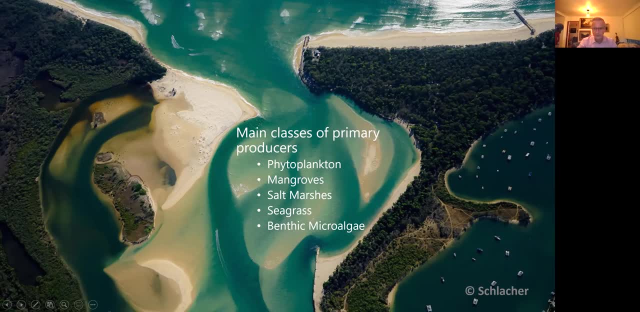 there is actually a few patches here. there is salt marshes here and we got all the you know muds here and sand is covered by thin layers of benthic microalgae. It's fantastic. it's this diversity of primary producers. yes, there is not type of that many. 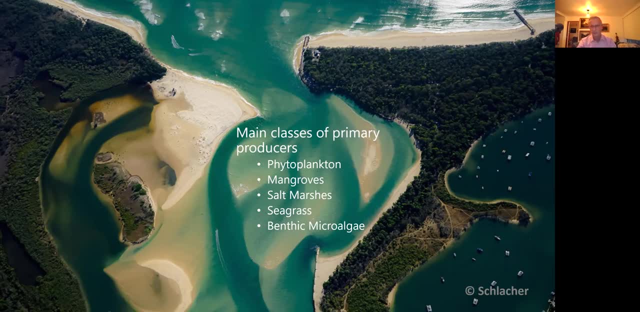 animal species or not that many- as we find in the open sea or deep sea or on reefs, but it really pumps carbon. So let's have a look at the fundamentals, why that actually happens, particularly when it comes to phytoplankton. Now here's somebody you know putting a bit of a fancy bottle into the water, but you can. 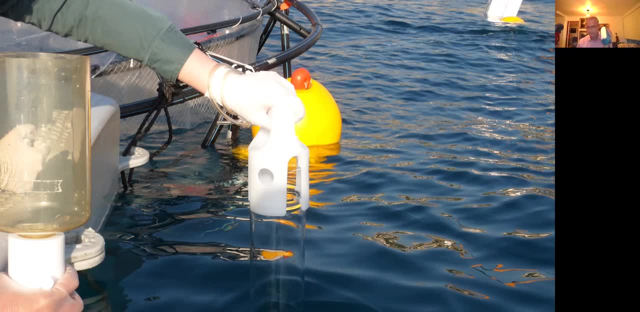 just use this one, but drink the gin first. you know, very, very important. So I predict that half of you will spend the first two or three working years of your life- if you stay in environmental science- collecting water samples, and this is exactly what I did when I came to the Sunshine Coast when this university opened. we just did lots of nutrient. 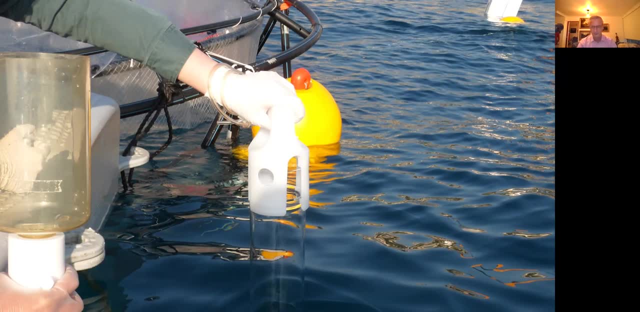 samples and lots of water quality and that analysis. I mean it is boring as batshit, you know, and that's actually, you know, being a little bit mean to bats- because essentially you just take the water and then you do a lot of chemistry and then you report on it, but people are obsessed. 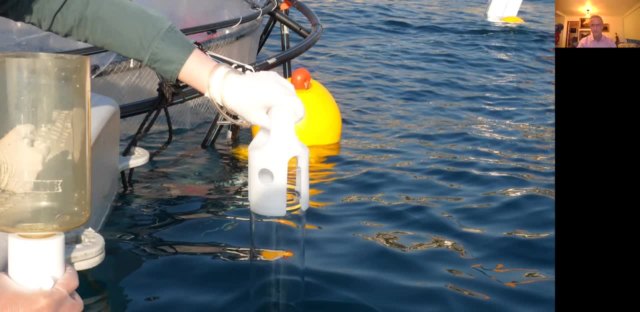 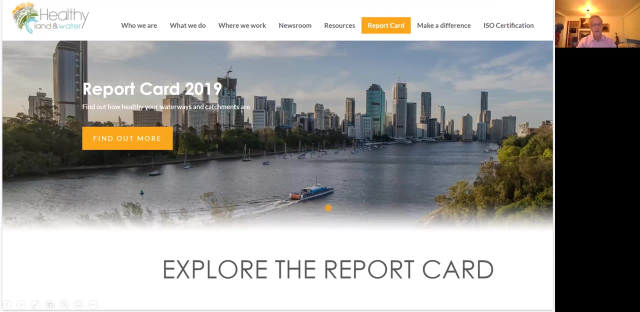 Absolutely, Absolutely, Absolutely obsessed with water quality, with nutrients. I'll give you an example here. This is the healthy water, healthy land and water. now it's called report card and it basically, you know, ranks all the estuaries and the different parts of Moreton Bay with respect. 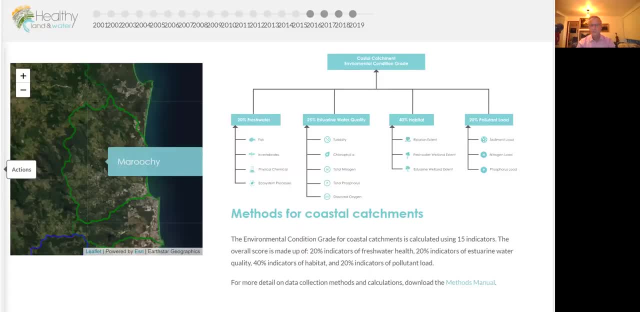 to the ecological health. If you actually explore a little bit, what this is all based upon is physical chemistry. basically that's nutrient, and here, look at this, for the estuaries, It's really, you know, debility, well you know. but here we go, nitrogen, phosphorus, and then 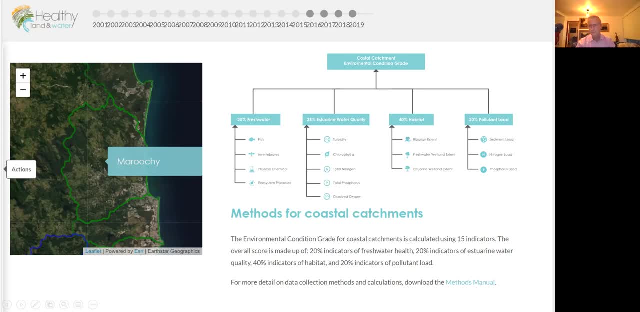 we go again: nitrogen load, phosphorus load. so it's actually half that report card, or arguably more. it's all about nutrients, so maybe it's not so much an ecological report card, but we can actually argue about that forever. we're actually doing a new one at. 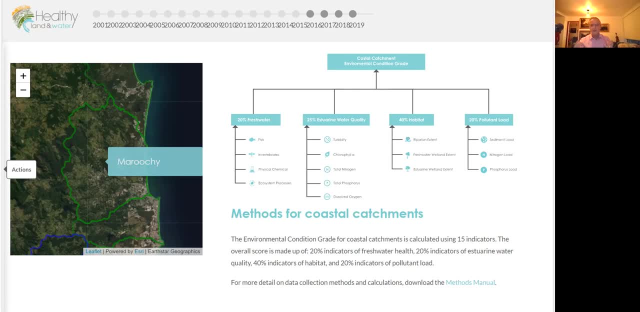 the moment. but never mind. there is an obsession, a fetish with nutrients and you might say: I've not quite, never got nutrients. I've never got nutrients. I've never got to that. be like I'll go out. and it's nitrogen, it's phosphorus and everybody. 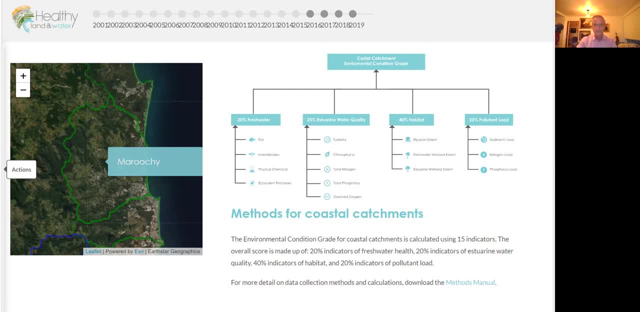 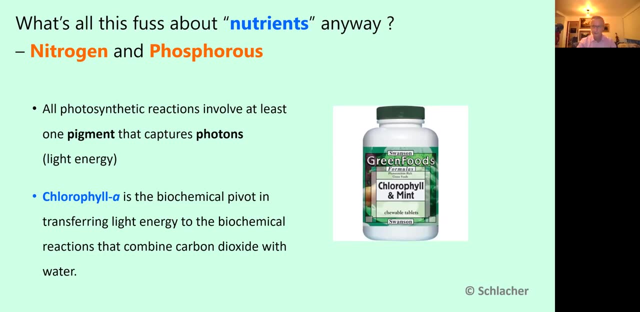 goes crazy about it, and there's different types of nitrogen. So you might actually say: why do we have this obsession when it comes to estuarine productivity, to study or to sample and measure nitrogen and phosphorus? I find this extremely funny. you know, you can actually go out and buy chlorophyll tablets. 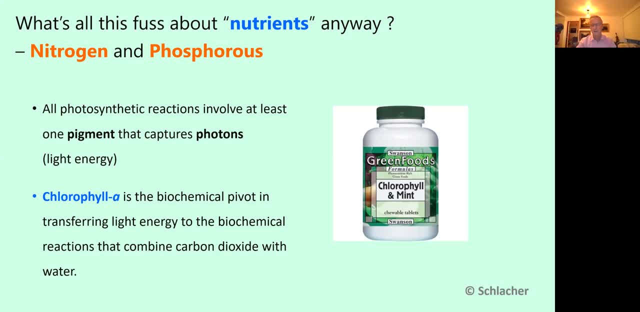 Well, Well. And if you have a deep- you know some people have a deep rooted, you know desire to, you know change, you know their biological sex and that's perfectly okay. I actually sit on the university's- you know- gender equity committee, So go for it. 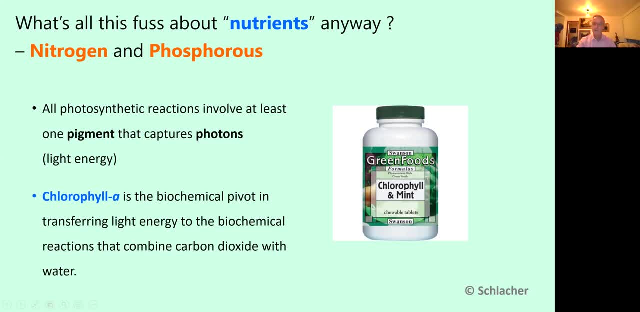 Do whatever you want, If you, however, have that desire. I don't really want to be an animal anymore, but we should never really be an animal, but, let's say, a heterotrophic organism. I don't know why people go out, and you know, You know. 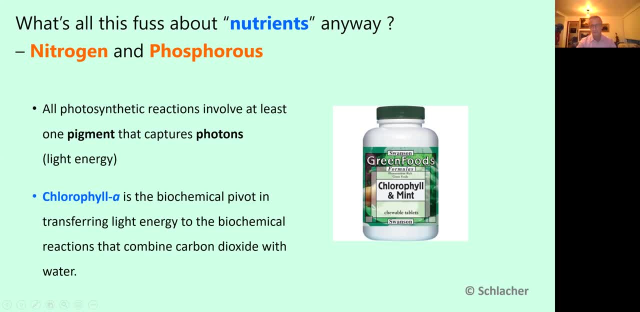 chlorophyll. Maybe they want to become a plant. Never mind, If you're a vegan and you want to become a plant, be one of them. You know, go and eat chlorophyll. Very, very strange. So essentially, there's a bit of an obsession of chlorophyll as well. 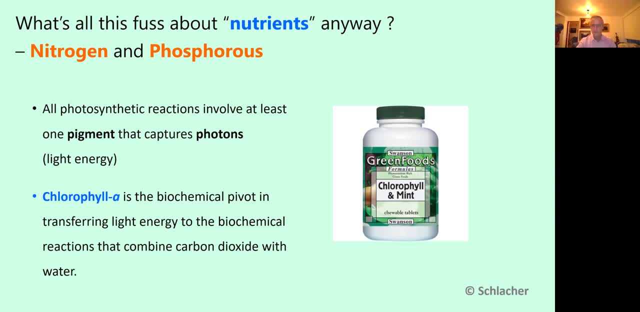 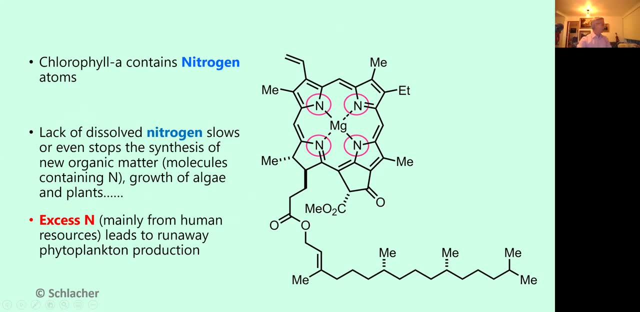 because they make our world green. Now, what has this got to do with nitrogen? Here we go. This is the structure of the chlorophyll molecule. It's a very simple one, actually, But it's that central group here, with the magnesium atom in the middle, which is literally bounded by four nitrogen atoms, And 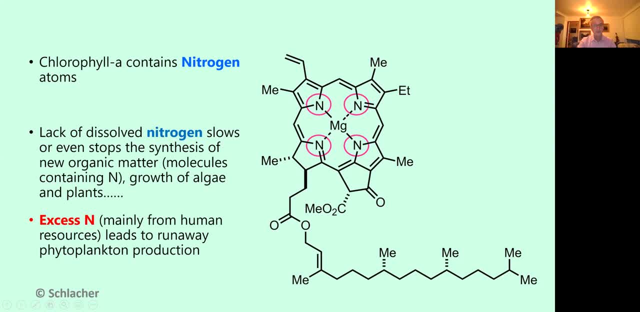 this is where the light capture basically happens. What this basically means is, if you don't have enough nitrogen, not terribly much happens in terms of plant growth, because the plants lack the chlorophyll atoms They can't make it. They run out of nitrogen to make what they're really. 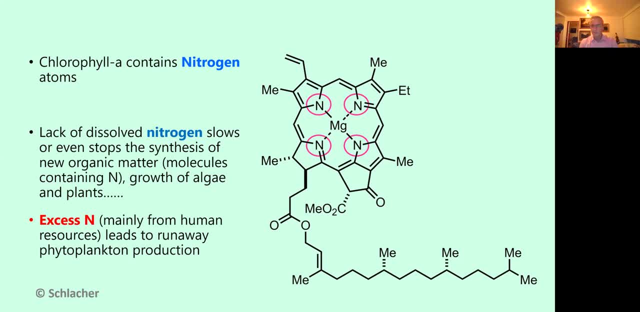 meant to do. If you, however- and this is the trick to understanding the obsession with nitrogen sampling and water quality- if you give it excess nitrogen bang and you have light and it's not too cold, it goes nuts And you fertilize your garden. 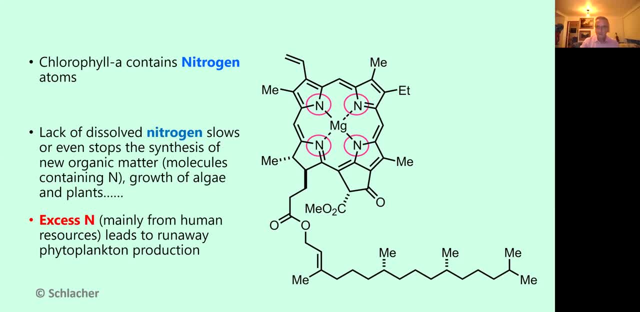 because, with whatever you want to do, actually fertilize it with. you know, we use horse poo. that's perfectly fine, because you're supplying extra nitrogen to make more chlorophyll, And more chlorophyll means the plant can capture more photons. Capturing more photons means you have 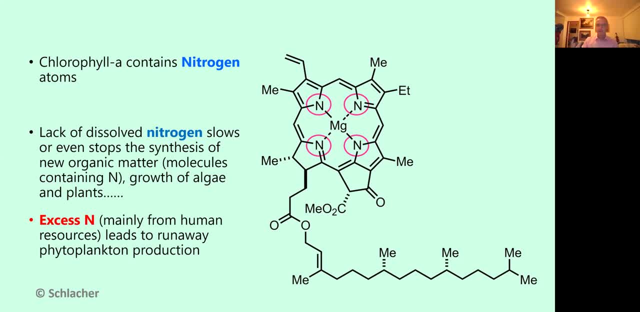 more energy to drive the photosynthetic reaction which combines carbon dioxide and water and makes carbohydrate sugar. Oh, no, Photosynthesis. So this explains why we focus on nitrogen. I quite actually never knew that, you know, when I graduated, So I thought I should tell you that, because 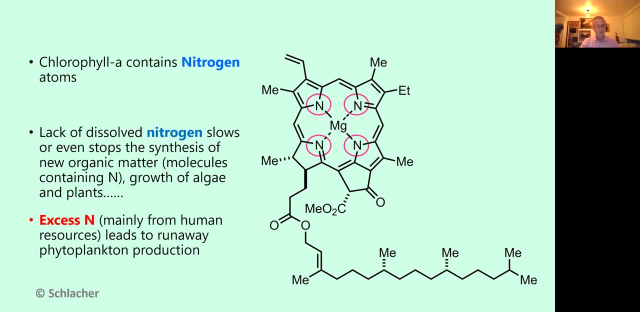 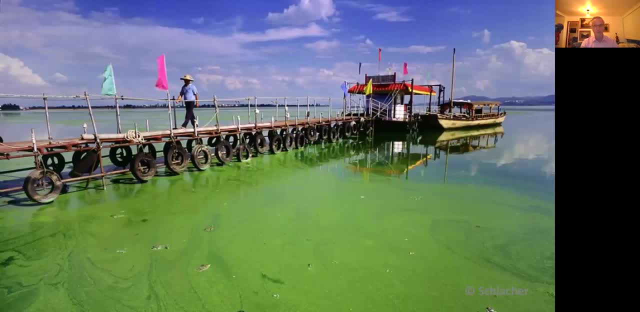 nobody actually knows. It's actually quite amazing. So why do we actually then- and this is basically what happens: if you have too much nitrogen algae go wabum, and we are actually a society rather charged nowadays or we actually seek not to. 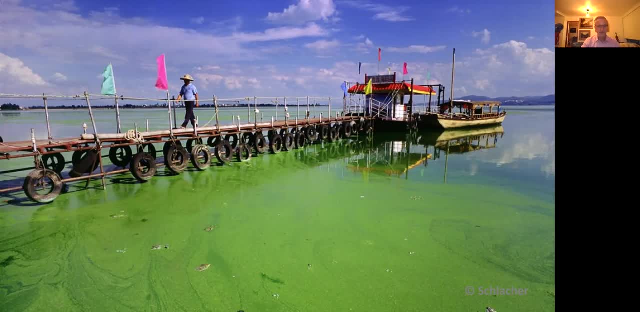 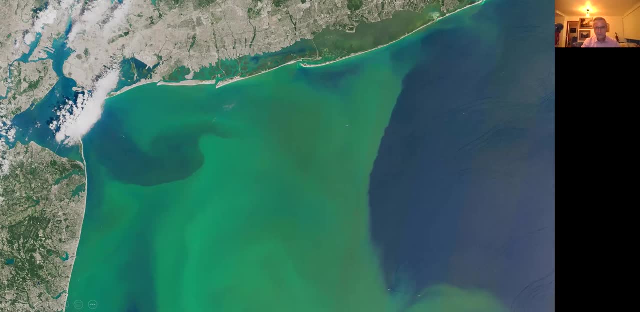 Not to actually have those conditions, at least in the developed world. And here's a fantastic one. Look at this estuary spilling out from this huge development that's in the States, Rhode Island. This is actually a phytoplankton bloom And it's all basically because of excess. 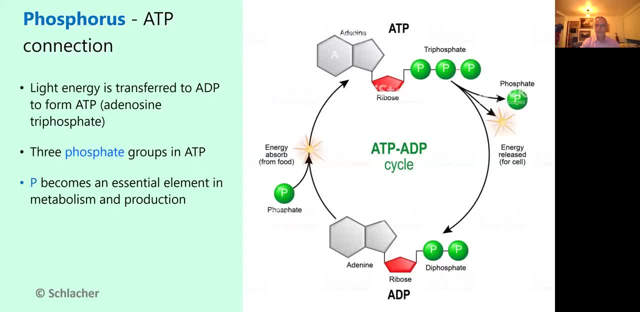 nitrogen. Right, If you have done wabum, wabum, wabum. If you have done biochemistry, you will probably get really specific Yeah. So, for example, I had a fucking great idea that I needed to go into biochemistry. 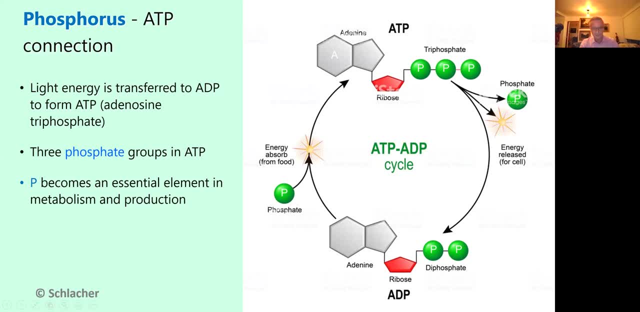 I had already started looking into it. you know, again I had to start looking at the other questions I had in my brain And you know I didn't want to go into. you know, go into a Spasmodic fit Looking at. you know those kinds of cycles I remember by chemistry A. 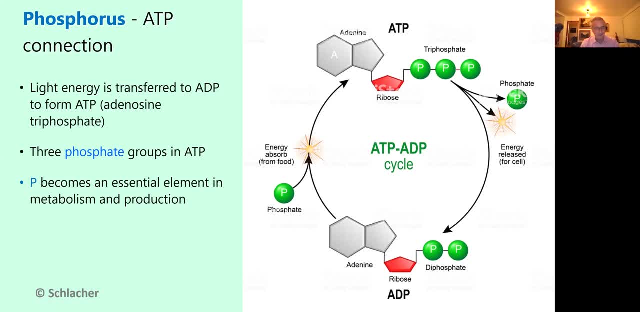 was eight hours a week for an entire year and there were like dozens and dozens of those biomolecular lack of cycles. but it's a very, very important one that we couldn't actually do anything with carbohydrates or proteins or fats into our body If it would not be for a very, very fundamental. 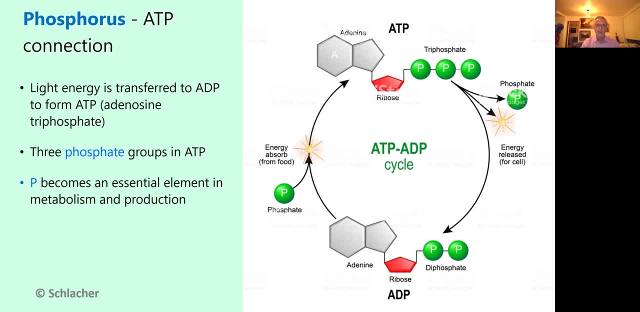 I was not the type of person that will do this 101 anddoor. So, yeah, I think we'll go with that one- our body- if it would not be for a very, very fundamental process called the ATP-ATP cycle. 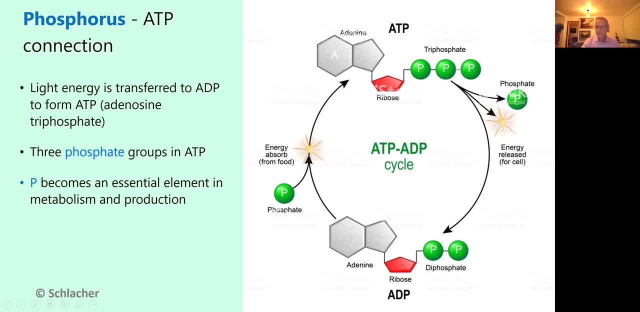 You have all heard about that. What actually happens is this is the molecule and it's in a triphosphate group, And when one of those gets lost, split off, the resulting binding energy, so to speak, becomes free energy. it gets released and we can actually drive our cell metabolism. 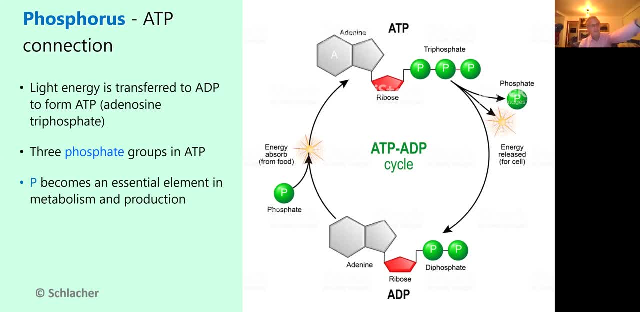 So as you sit at home now, you can probably have- now it's after five- you can probably have gin and tonic, because this guy can't see you and eat peanuts or M&Ms. I have to actually maintain the professional integrity here. 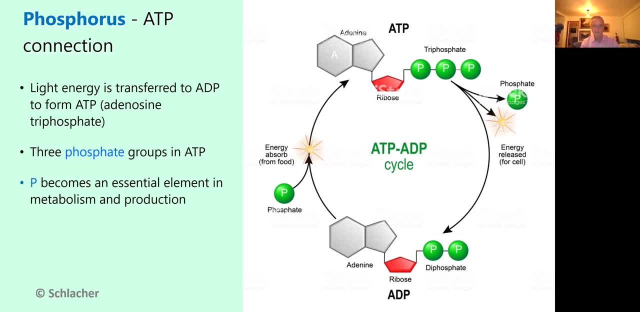 But essentially you're going to supply yourself with some sort of snacky energy, But ultimately, what makes your cells function and survive is that cycle here. And so if you lack phosphorus in your diet, you die. And because you could- theoretically, let's say, there would be a diet which has everything. 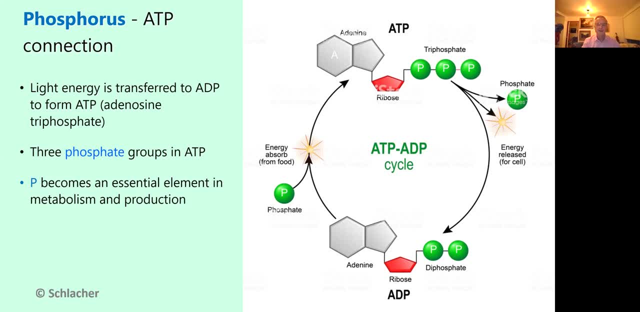 in the proteins, which is, of course, impossible. but then why? because they would have phosphorus in it. But let's say you could actually devise a diet which has no phosphorus. You can actually eat as much as you want. ultimately you will die if you don't have. 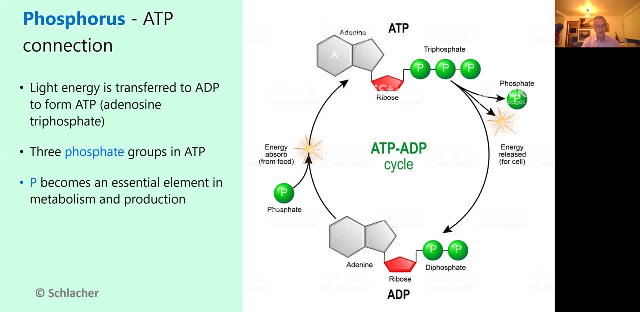 phosphorus, Because that fuels your cell cycle, So it's actually quite important. So it also means if you have more phosphorus in the water, the plants can actually cycle faster and make more stuff. They can produce more complex carbon from simple carbons, which they take up as HCO3,. 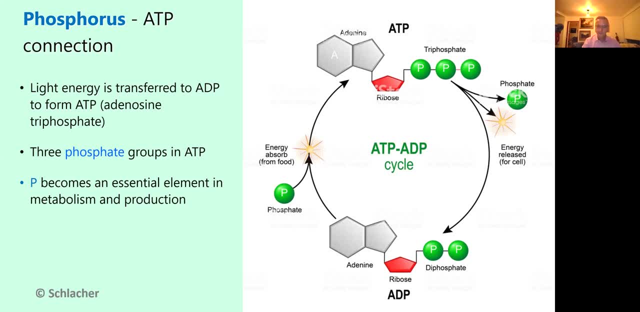 like bicarbonates from the water. If there's anything unclear, ask me now. I think this is actually very fundamental. So next time you have to actually take a water sample and analyze it. at least you kind of understand why you do it. 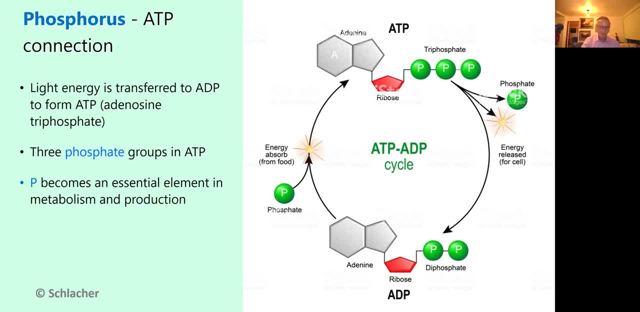 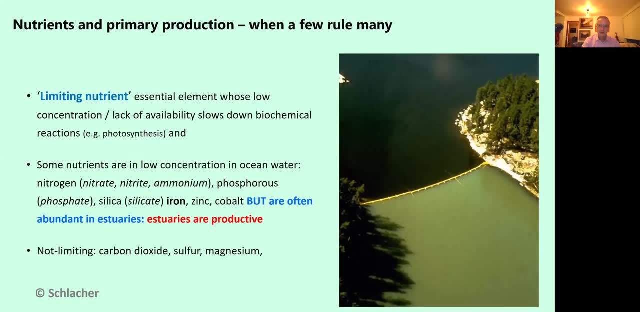 And that's why we have such a big emphasis in controlling the efflux and the import of nutrients into shallow water bodies. There's another thing, which is one or two more concepts. I have to actually explain to you why nutrients are so important for primary productivity. 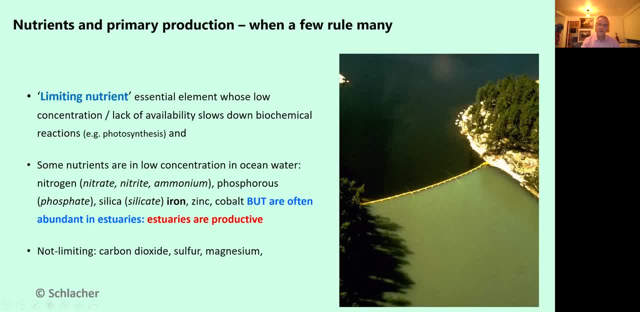 I know this is more botany. This is carbon. This is a concept which has been around in botany for quite a long time And you might actually know about that. If anybody grows plants, you can sometimes chuck all the nitrogen fertilizer on them. 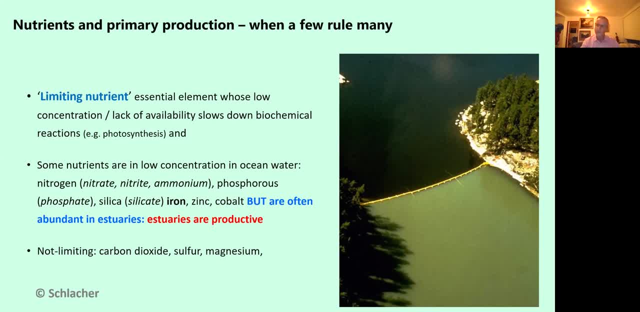 or phosphorus, And they still actually don't grow very well, Because if you have one or two micronutrients missing in the soil, it doesn't matter how much of the other ones you have. It's called the limiting nutrients, And sometimes they can actually be quite beside the minimum. 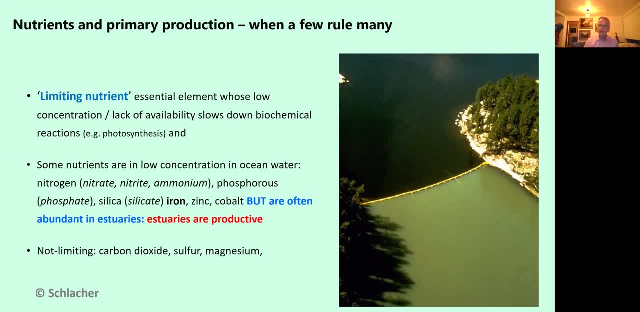 So if you have one or two micronutrients missing in the soil, it doesn't matter how much of the other ones you have. It's called the limiting nutrients, But variouschosシ are in small concentrations. One of the most famous ones is, of course, iron, or zinc and cobalt. 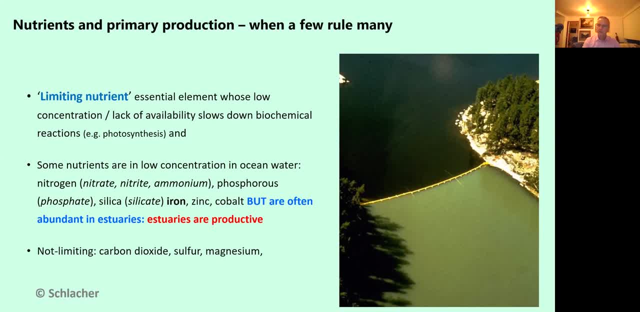 And usually there are not limiting industries. They are in the open sea and there have been very, very famous experiments where people ran out with very large ships and chuck a lot of iron overboard near Hawaii. The nitrogen concentrations are the same. the phosphorus concentration is the same. 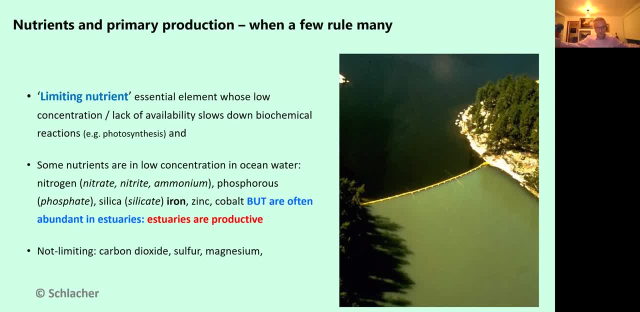 But the phytoplankton in the middle of the Peruvian Pacific skull is on the same, So the quality of oxygen there is very good. That's another concept that I'm going to talk about, And whether it becomes like a more drought. OnePlus and the ecofl selfie, timecze and production. 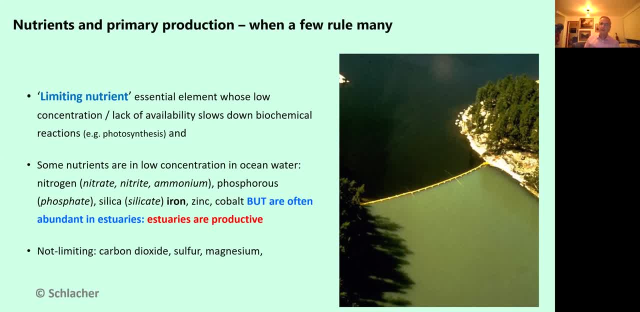 haven't started. the water's turned slightly green, So iron was a limiting nutrient in the ocean. we actually discovered that, But not so much in estuaries. We have usually enough, because they are tightly bound by the lithology, by the rocks on either side. So the other one is: if you have 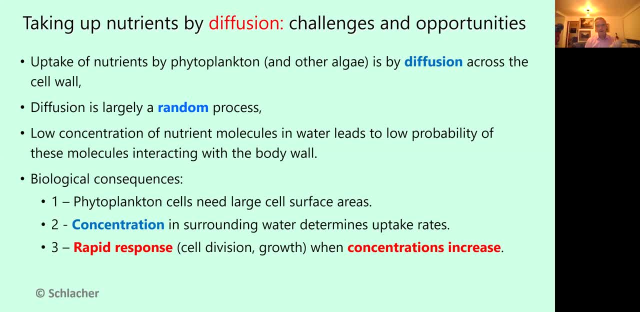 phytoplankton- I'm just telling you this very, very quickly- is essentially: you don't have roots. Phytoplankton don't have roots, So all the nutrients which you get you have to get from diffusion across the cell wall. That basically means this is a completely random process. You 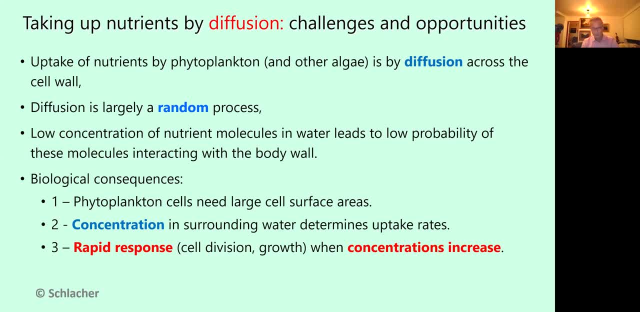 can't actually go out like a root and tap into a nutrient reservoir. So essentially, if that is, the concentrations in a surrounding water are the number one determinant of how fast it grows. that also means, quite frankly, if the concentrations increase, you grow a lot. 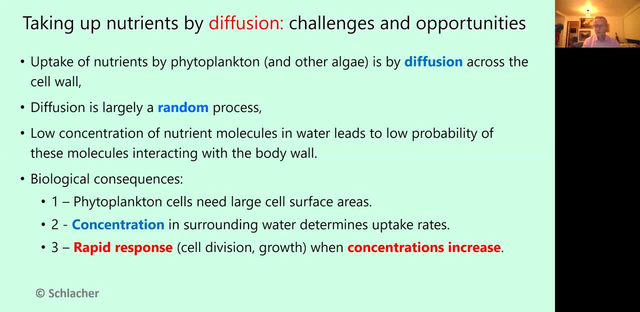 faster and like a lot faster, and that's why you get phytoplankton blooms. it's much less so the case on land, because the complex, you know- processes of the vascular plant taking nutrients up through the roots and then distributing it, you know, throughout the rest of the body. right here comes my botany train. 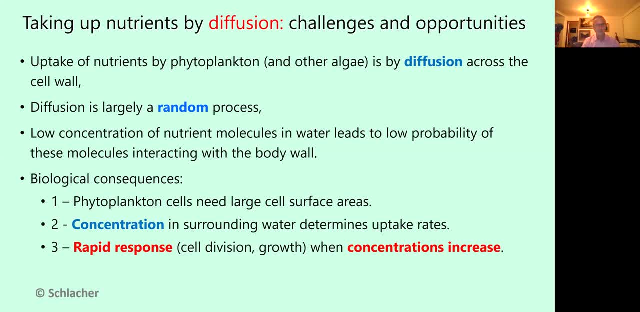 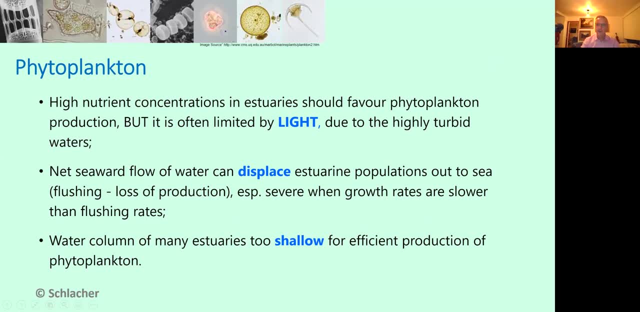 to the floor. I apologize, you know any case. so we have a few of the major groups of primal producers to actually cycle through, but I just, you know, want to, you know, get out of ten minutes and then get on with the. phytoplankton is the. 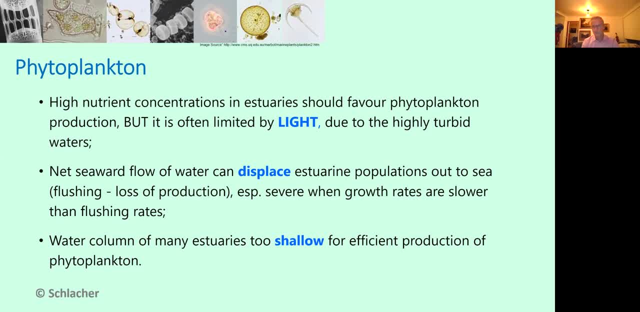 first one and then we do the rest one in the next lecture and also move on to the anemones. so if you are one of those phytoplankton cells up here, what you will experience in an S3 is can be very favorable conditions, but also. 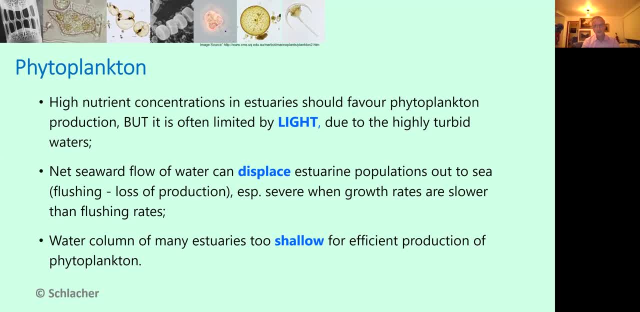 very challenging. remember you can't really swim against the current. we are talking about the pre-linked on again, and those are- I mean, I got a little flat jelly but they're not actually terrible good. so essentially, bacterial concentrations are high right, so this would actually favor, but I 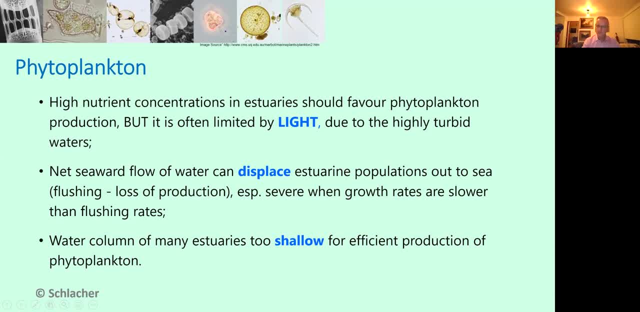 but light can be limiting when the waters are very turbid, And environmental managers are often extremely disappointed because, let's say, they want to get phytoplankton blooms down in occurrence and in frequency. so they clean up the system, so to speak. And if they make the S3 too clear, the water too. 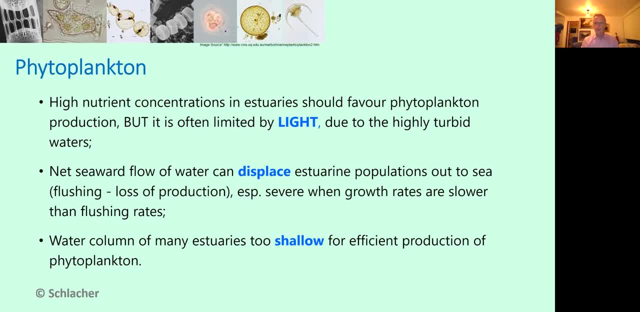 clear. you get more phytoplankton And they go like: oh, we have done everything right, Well, you have just provided more light so they can actually grow. What you need to do is reduce the nutrients and the turbidity. at the same time, Phytoplankton often gets washed out. 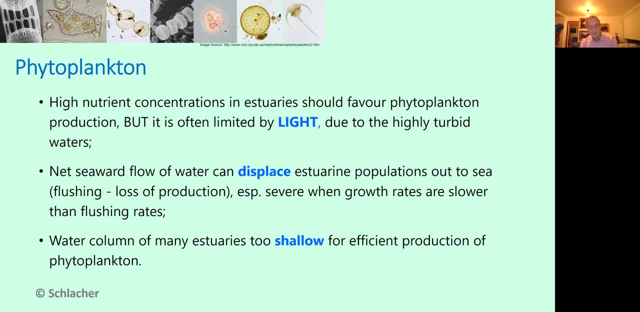 to sea. so they have behaviors which actually minimize this And, interesting enough, they can actually migrate up and down in the water corium. So if you have a phytoplankton, you can see that they can actually migrate up and down in the water corium. So if 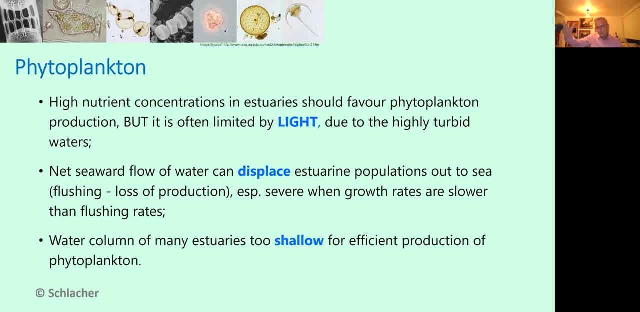 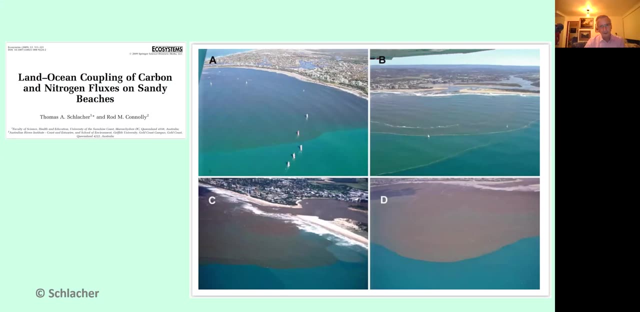 the net seaward flow is too high at the top, they migrate into deeper waters where sometimes you have actually a net upwards transport system, So that all seems to be good. So what do I mean by displacement? This is a study, you know. we did a few. 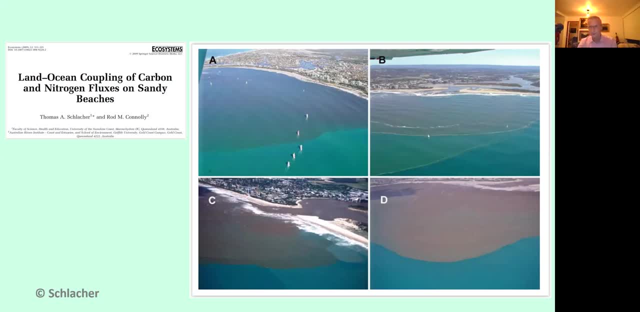 years ago and we, you know, got quite royally funded. That was fantastic. Canberra gave us money and it actually enabled us to rent little planes all the time. Fantastic. We flew up and down the coast because we were chasing blooms of turbid water going out into the sea. 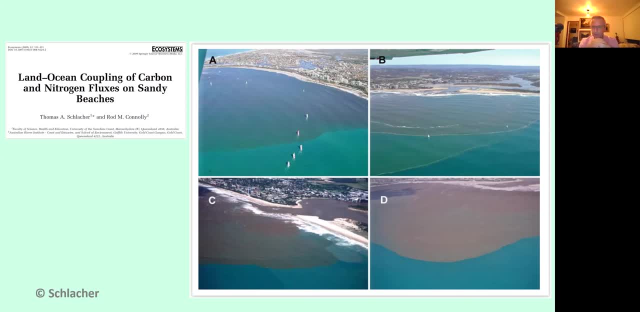 Oddly enough, not many people have done that before, because we figured this is actually a very major event and we actually got a few of those over two years. As you can see, this is Miglura power and this is the groundwater pushing up. This is the essригens and different blooms. This is very interesting. 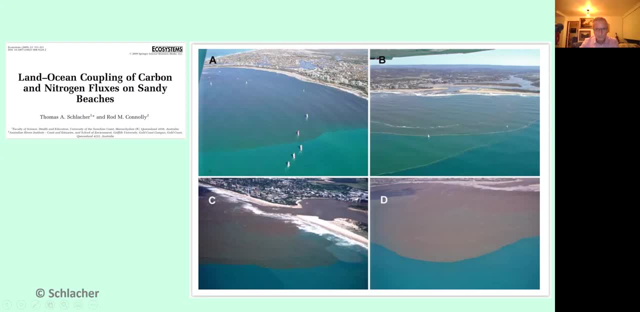 these blooms have a veryae60 percent growth from people, orалось, some, some animals, from environment to environment. This is quite interesting. Those blooms are getting ahead. A lot of them were going out there, a very sharp edge, so obviously this major pulse of water going up would actually have displaced. 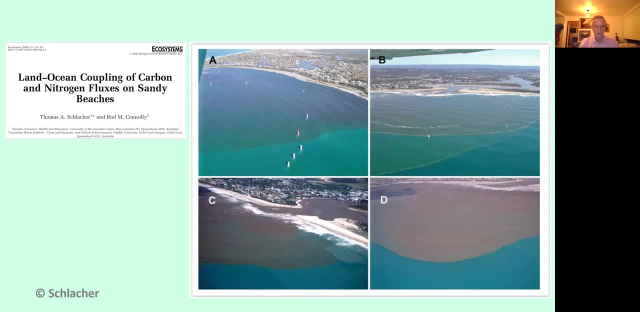 a lot of the phytoplankton inside the S3. but what we actually found is, once this actually phytoplankton reaches the sea and the turbidity over time goes down, we have an incredible phytoplankton response to it. it's also a very convenient system because what we discovered by 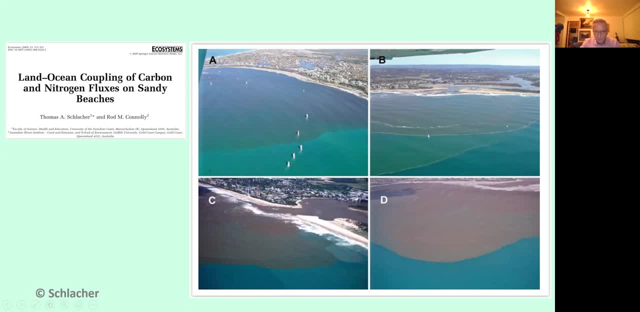 you know, using a boat. those are the yachts coming in and here's my house. you can actually see that I shouldn't really tell you about it. if you come and steal all my paintings, never mind is that. it's very convenient because it's such a sharp edge, so you can sample here bloom conditions and 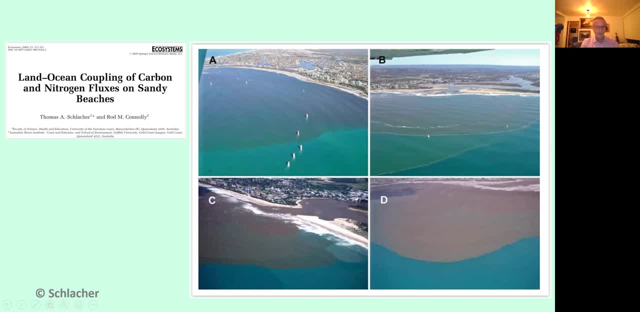 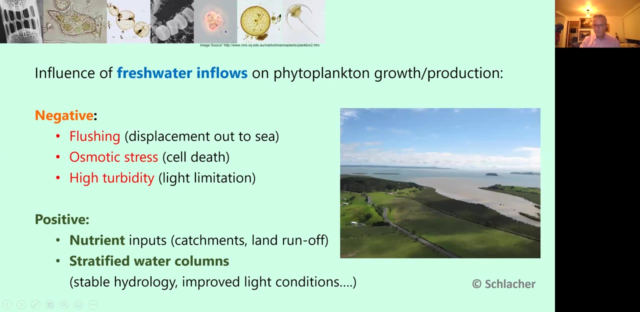 then you sample here oceanic conditions. where else in the world do you actually find such a great difference in water masses between over a very short distance? so that actually worked out quite all right. so it is still, you know, a little bit of a problem if we have a turbidity problem like this going out, so flushing is a. 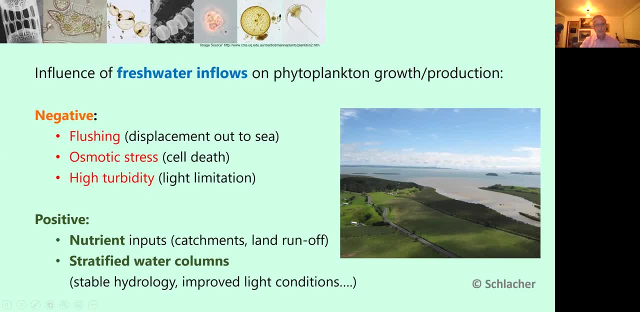 problem that creates osmotic stress and turbidity, can be limiting for light, but it is nutrients. those blooms deliver a lot of nutrients and they also create a stratified water column. why is that important? stratified means a layered ones. it basically means if there's a more stable hydrology. 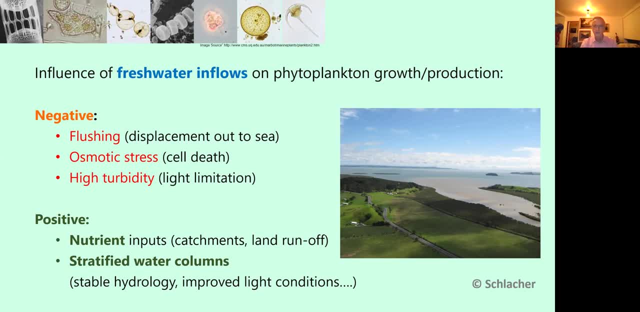 ie different water layers exchange, you know, water masses less so than a unified water body. you can literally hang out in better conditions if you have fight the plankton bloom, because you don't get displaced and sometimes there can be a more clear layer of a more turbid layer. so that's actually all right. 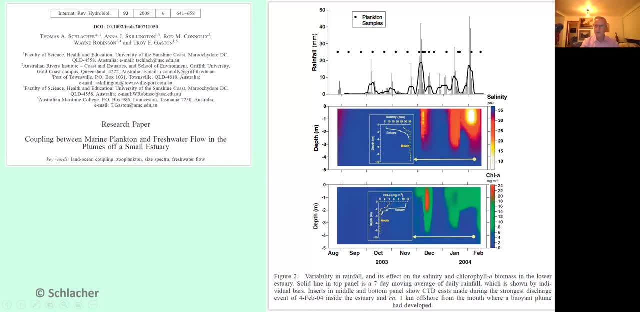 how do we actually know that? it's another study within with answer? you know again. you know i try to look at the graph, so the here we can see the average of the climate and the climate of the world versus the average of the environment. um, so these are the data that's used in the 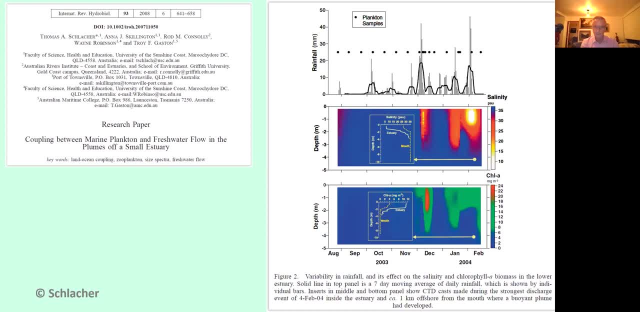 this. one of the data is that the climate is always definitely dependent on water, water storage, and what we did was we found that the most common point for water storage is that the water is kind of separated, as you can see from the diagram and as you can see, 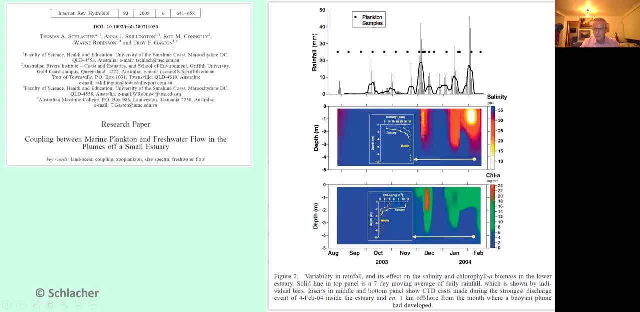 from the graph. then we found that, sorry, that's the degree of what and what. we entered into this study. so we had a bit of a chat about what you should do as an ecologist, and my advice is: do everything you know. the world is fascinating. so what we basically did- this was a study we did in the estimated in the Boologhandi today, just down from my house, and 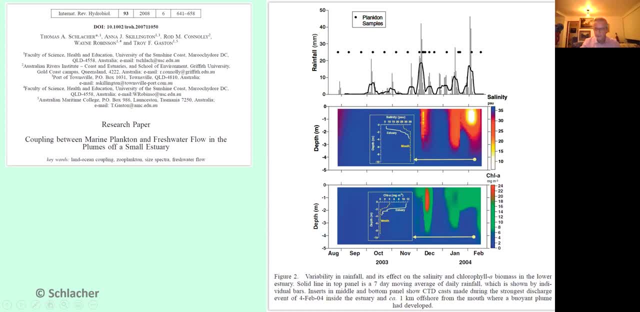 the freshwater flow. the rainfall goes into the street, you know. the salinity goes down. but what also happened is look how stratified the s3 became fantastic. like a stable hydrology. it created this freshwater layer which went out as a brown bloom into the bay and it was like whoa. you know not so. 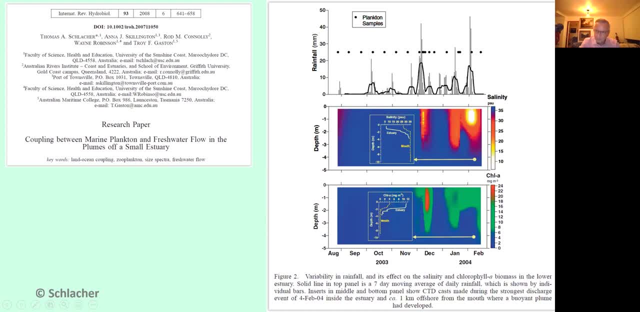 good, but it was only just at the top that suddenly it didn't penetrate even a few meters down. this is like five meters deep at the mouth of the muller s3. but what it actually did is it created a fantastic bonanza in chlorophyll that it just bloomed literally, and i have to say it took me. 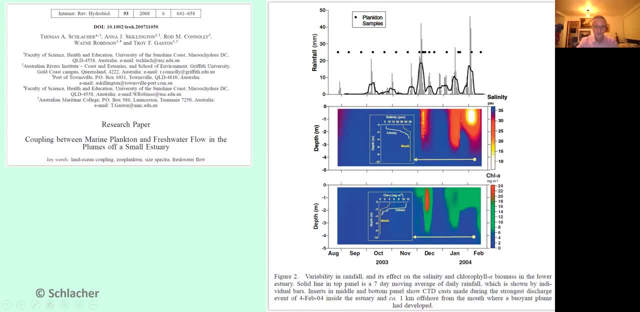 quite a long time to to do this particular graph and analysis, but you couldn't almost invent, meditator, if you tried to- that the change in a rainfall and in salinity with a stratification almost mirrors perfectly the chlorophyll, a concentration which we use as 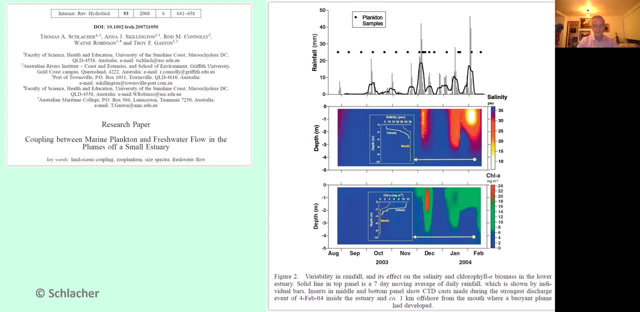 an index for phytoplankton. i mean, if you ever want you know a better, you know uh? example: that land runoff, runoff from the catchments, or the americans call them, the watershed, promotes what creates blooms of phytoplankton in an s3 at the sea. here you go, perfect. 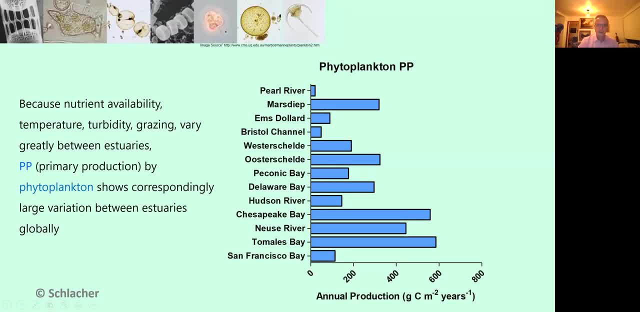 now, because you know phytoplankton is, you know, often, you know so- governed by the differences between light and humidity and otherwise it's. you know this is our. those are values i sucked out from the global literature. and when you actually do that and you work out what the annual production, 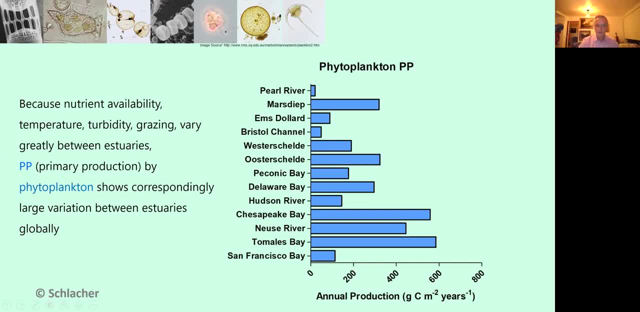 is in grams carbon per square meter per year. there's a huge difference and it shouldn't actually surprise us. you will see a few of those diagrams as we go through different classes of primal producers and it's important. you know they look a little bit confusing, but i put them in so 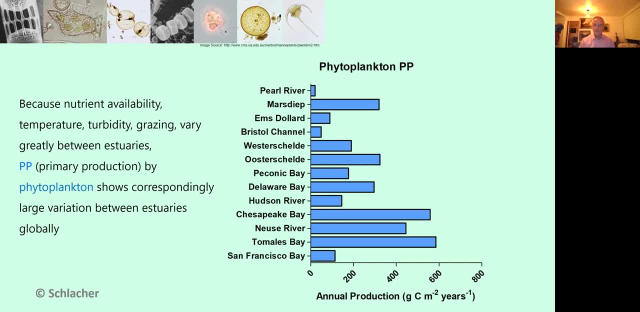 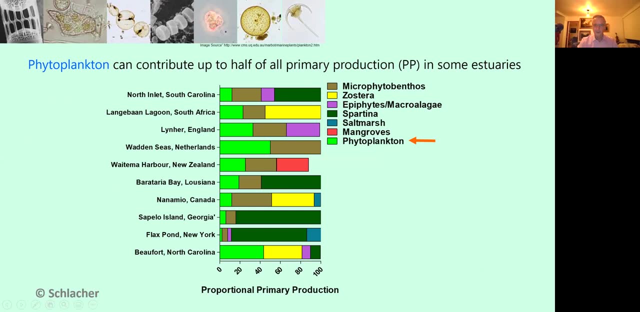 you can see that no system is the same. you have to study the principles but the actual values they don't actually often matter that much to actually compare them because every system has a different dynamics. so this actually shows it a relative percentage contribution of that green one.